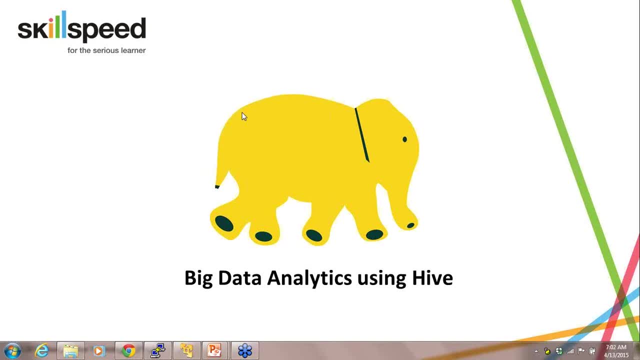 Okay, Sudip, is Hive a query language similar to SQL? Yes, Sudip, Hive is a query language similar to SQL and that's called SQL Hive Query Language, Trying to understand real-time usage. Okay, Sachin, how about the rest guys? 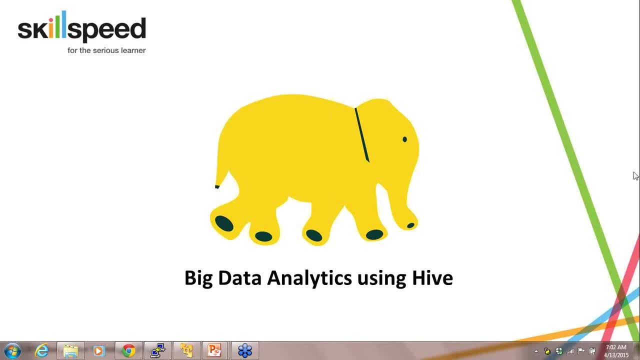 Now Abhijit, Abhishek, Ajit, Akshata, Avarnath and our. Okay, why it's called as big data. Okay, Siva, we'll uncover that, as well as to why it's called big data. Do you use Python with Hive? Absolutely, we can use Python with Hive. If you're interested in that, I can give you some examples as well. 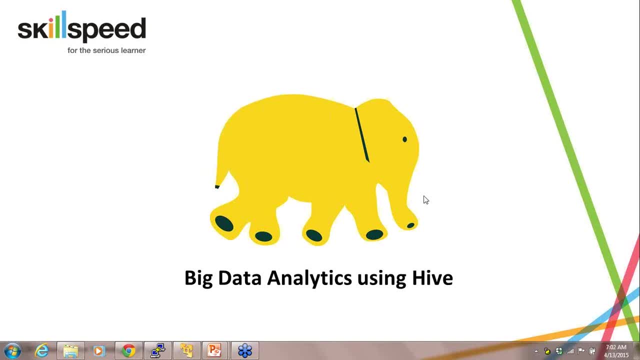 Okay, Kalyan. hey, Kalyan, learning how to use queries for big data. Okay, Madhusudan, want to know practical use in different industries. Deepak, okay, Deepak. What about R? You can use Hive in conjunction with R, but that's not what we are going to cover today. Okay, so I'm going to cover things from big data analytics using Hive. 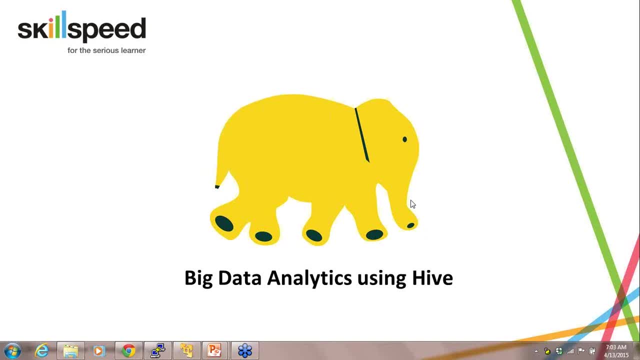 Now, Hive can be integrated with R. Hive can be integrated with Python. Hive can be integrated with Java, so Hive can be integrated with almost all languages for which interface has been built. We are. we will not be talking about R today, Ajit, Okay, what's the difference between Hive and Pig? Okay, so we I'll try to touch upon that as well. The two are different languages but built with the same intention. 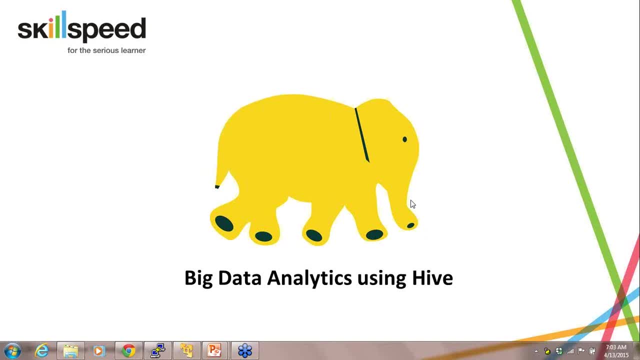 Pig was built by Yahoo, whereas Hive was created by Facebook, and they have similar properties and they do similar stuff as well, but then there are small differences as to why one should be used for one type of data processing and others should be used for other types of data processing. 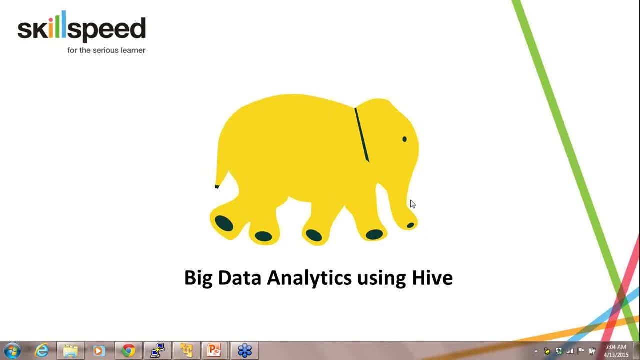 If I have time, I'll discuss about the difference between Pig and Hive as well. Niharika says her expectation from the class is to just get basics in big data. I'm looking to switch platform. I'm currently working in open system and want to check if big data is the right move. 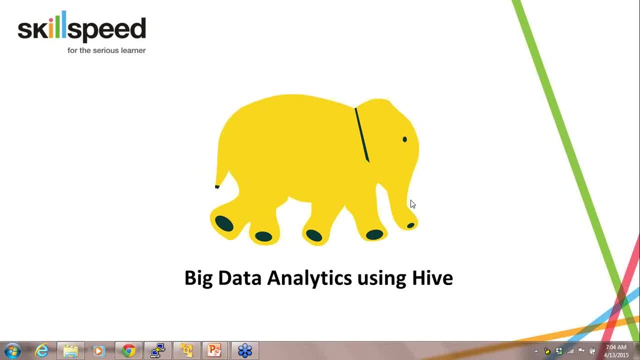 Okay, Niharika. why is it preferred compared to existing SQL? Okay, Kumar, I'll explain that. as to what's the difference between HiveQL and Pig, You know normal SQLs. I'll explain that as well. Hive is similar to SQL, just that it's schema on read- Okay, excellent. Whereas SQL is schema on write. You already know that answer. 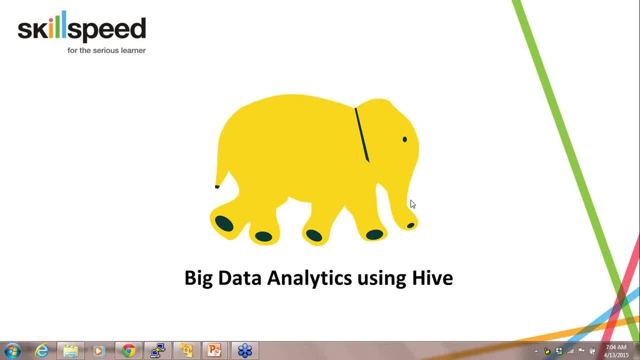 So we will uncover more of that a little later. Guys, one more minute. If you want to type in something and then I'll get started, Okay, if you want to type in your expectation from the class or your understanding, what is your understanding of Hive? I'd be able to put it in. 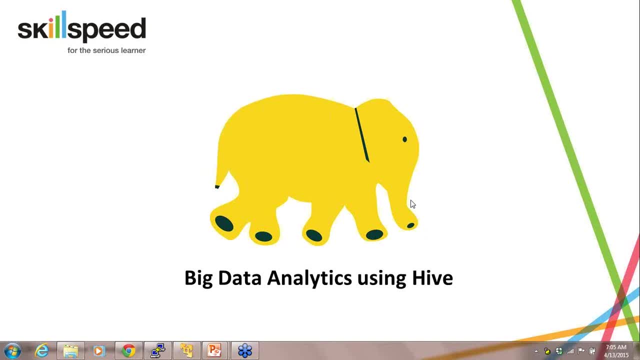 Better terms. Sudeep says: please explain in layman language. Absolutely, Sudeep. This will be completely layman language. It will start from zero, so you can be rest assured of that basic idea about big data. Okay, Amarnath, Moving data in and out of Hive. Okay, Sachin, Introduction to big data and best ways to learn more. Okay, Akshata, Sanjay, here I am expecting to get a good grounding in Hadoop. Okay, why Hive? Okay, excellent, Balaji. 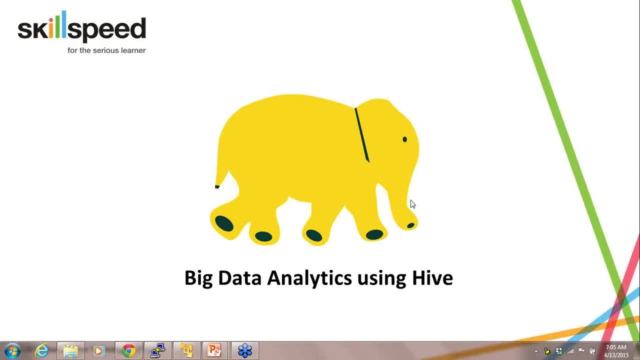 Okay, excellent, Balaji. Okay, I'll wait for four seconds and I see lots and lots of questions coming in. Okay, Could you please also cover read on schema feature of Hive and how unstructured data in Hive is different from MongoDB? Okay, absolutely, and so I'll cover that as well. 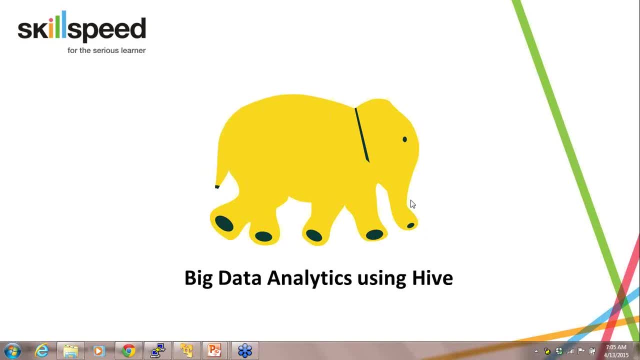 Vishal, something about security in Hadoop will help. Okay, Vishal, I think I will not be able to touch base on security in Hadoop and Hive right now because of time constraints, Vishal, which we can do some other time, I guess. 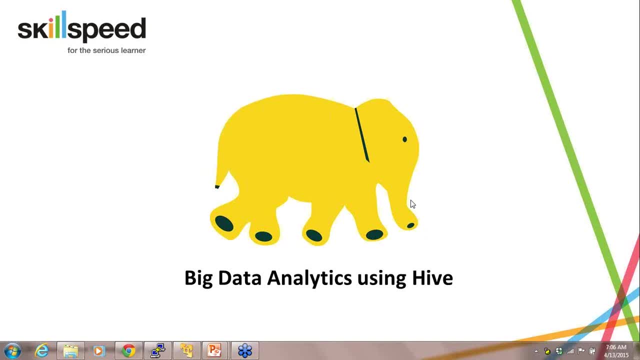 Okay, Balaji, Okay, but I'll try to at least touch base on that. Okay, Hey, isn't PIG a programming language and Hive a query language to query the big databases? Okay, PIG is a data flow language. PIG, by definition, is a data flow language and Hive is a query language. Okay, but then they were meant to do the same stuff. They were created with the same intention and hence the functionalities are quite similar. We will see the differences later on. 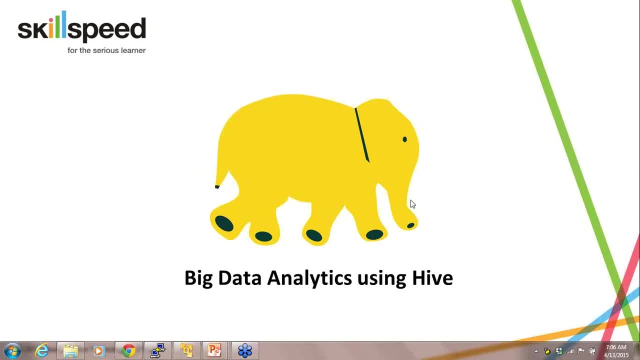 See, I am working on integration platform. want to know how big data training for my advantage? Okay, SQL is for structured data, Hive is for unstructured data. Okay, Akshata. So there we go, guys. We have run out of time on taking your questions, so let me get started straight away. 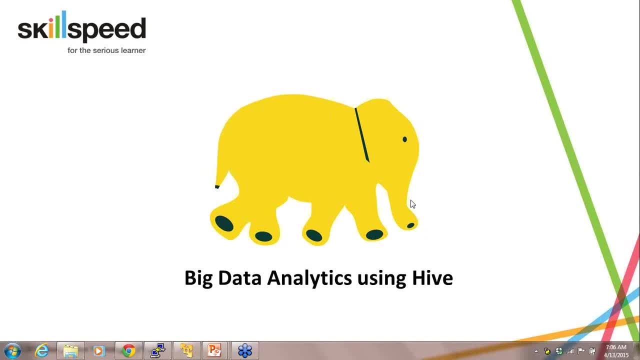 Okay, Edwin says I'm currently studying CIS database management, but my school does not offer any Hadoop courses. Why are so many schools not offering Hadoop, even with its propriety? Okay, so I don't understand the fact as to why schools are not offering Hadoop. They are supposed to because there's huge demand for Hadoop and there's so less supply. 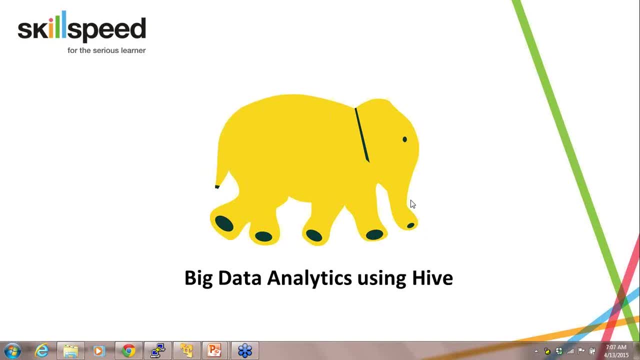 I think they will eventually come up with this initiative to teach Hadoop, but right now I don't think. apart from some of the main schools, none of them are teaching Hadoop. People do go ahead and teach big data analytics, but that's more from perspective of mining data. Okay, so I'm currently studying CIS database management, but my school does not offer any Hadoop courses. Why are so many schools not offering Hadoop, even with its propriety? Okay, Edwin says I'm currently studying CIS database management, but my school does not offer any Hadoop courses. Why are so many schools not offering Hadoop, even with its propriety? 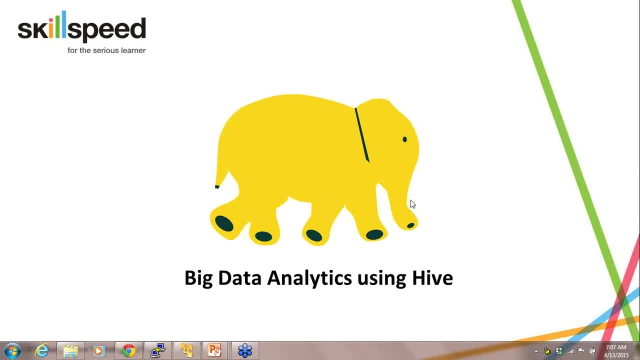 It's all data perspective. They go ahead and teach Python. they go ahead and teach R in order to do data analytics, but not Hadoop as such. Okay, so they have Udacity intro course in Hadoop and MapReduce by Cloudera. I think it's a good start. 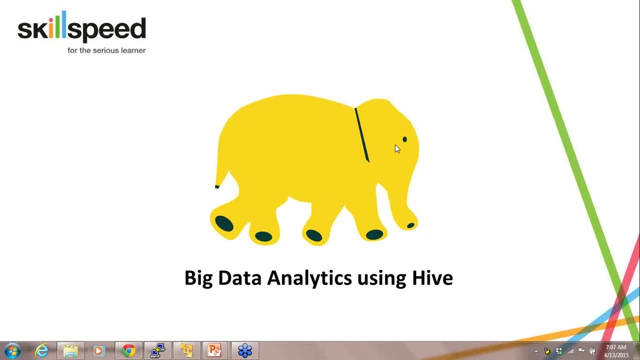 Yeah, Kumar, for a starter that's good, but it does not give you a lot of insight into what actually Hadoop is. I mean, for a starter, yes, that's it. I think it's a good start. I think it's a good start. 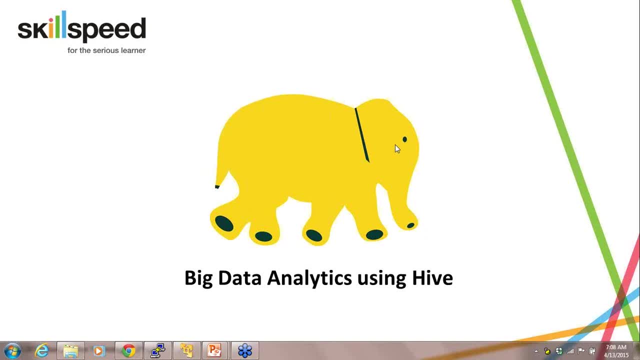 that's a good place. Hi, okay, Rohini, here I would like to learn the basic query issues in Hadoop. Okay, guys, let's get started. Okay, thank you guys. Thank you guys for putting in your questions and your expectation from the class. 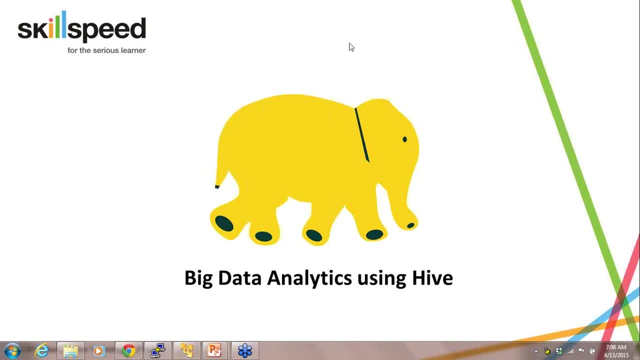 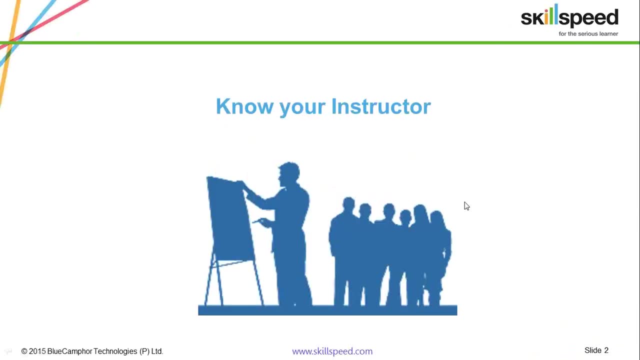 Now let me go ahead and tell you as to what big data and let me explain to you as to what big data analytics is right that we're using. hi, Okay, now you're instructor of. by now, you would have known my name. 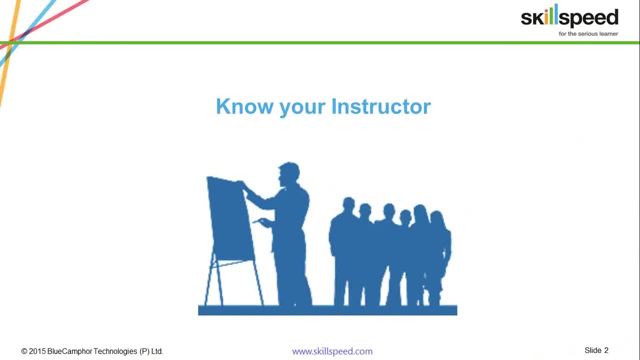 You'd have gotten my name. My name is Yogendra and I've been working in this industry for a very, very long time. It's been almost a decade and a half- right, Even more than that- I've been working. I started working on various technologies. 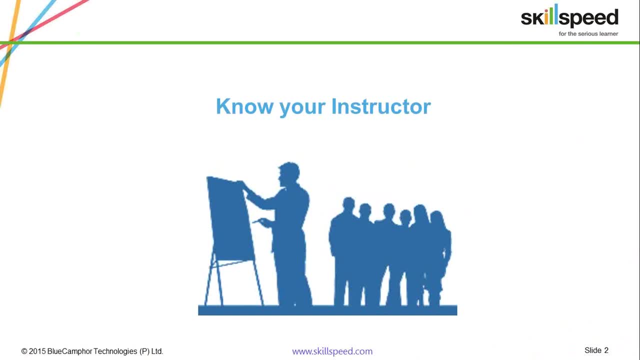 started working from Java to Oracle to lately, when there was, you know, when big data initially started. that's when I moved into big data And from since then I've been working on not just big data, work on big data I've worked on, you know. 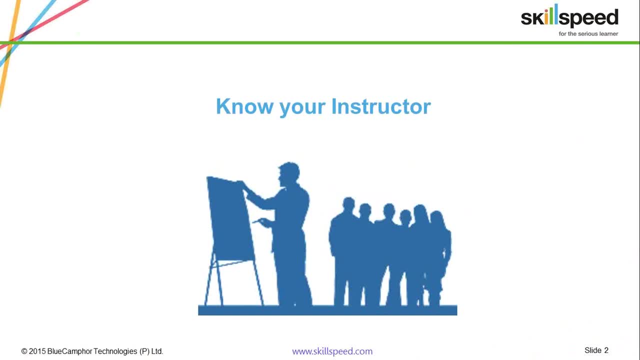 I've worked on Python, I've worked on R, I have worked on Informatica, just name it- and over this, so many years, right, I've worked on many tools and technologies, of which, and you know, I have fallen in love. 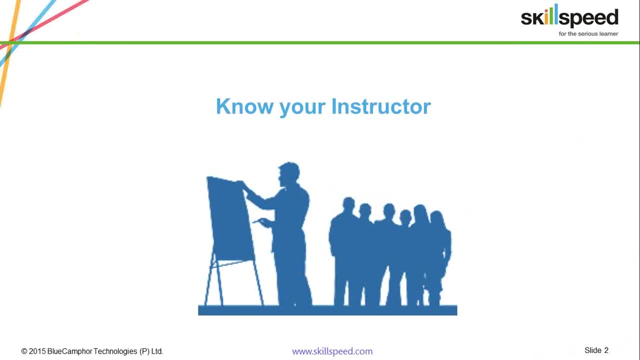 with a couple of technologies. right, I have fallen in love with Hadoop ecosystem, And the other thing I love is Python. Okay, these are the two things I've fallen in love with. That's about me. I've also worked on from starting an MNC. 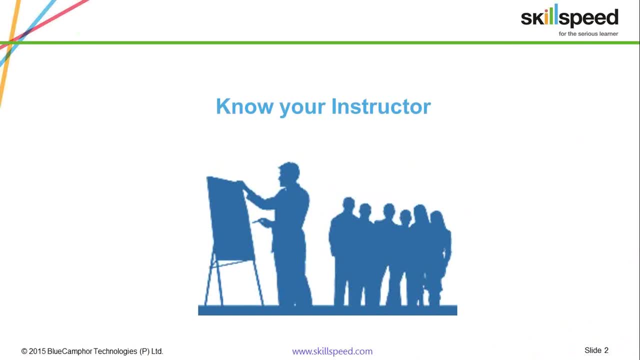 which I started my career and then moved on to start up, created something of my own which actually did not run, and then had to go back and work again. So that's my introduction. I have different types of experience of trying to learn something of my own. 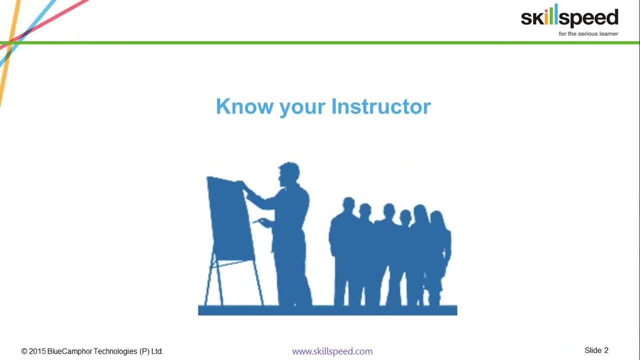 to supporting a product, to creating a product for someone else. So that's mine, And over the period of, I'm sure, with this much of experience, all of you will go through these phases, okay, So let me go ahead and talk about. 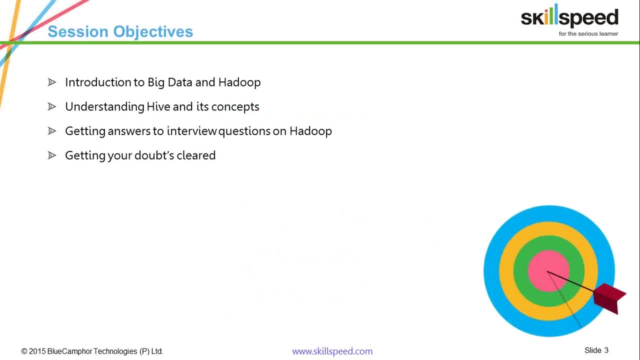 session objectives. I'll give you an introduction to Big Data and Hadoop, understanding Hive and its concepts, getting answers to interview questions in Hadoop and getting your doubts here. I already know as to what your expectations are from this class And apart from that. 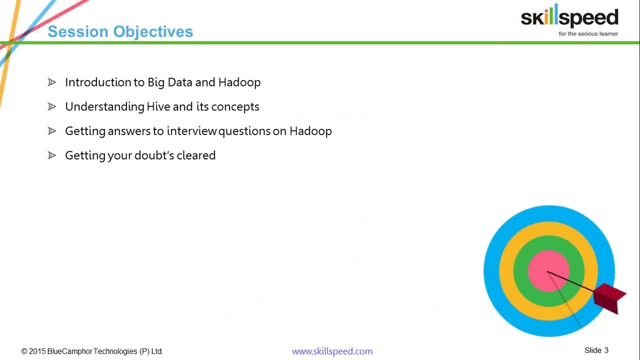 I would also set the ground rules on, basically on how Hadoop works right. I'll also tell you things as to how industry perceives Hadoop and Big Data, or Hive, right As to how Hive is actually being used in industry and which are the industries which are coming up. 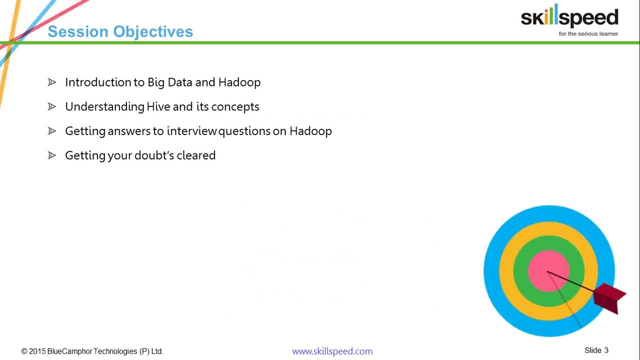 with lot of requests on Hive and a little bit of Hadoop, right. Mostly this is what I have seen. okay, I have worked on in various places. I know a lot of my friends, colleagues, working in various different places, right. 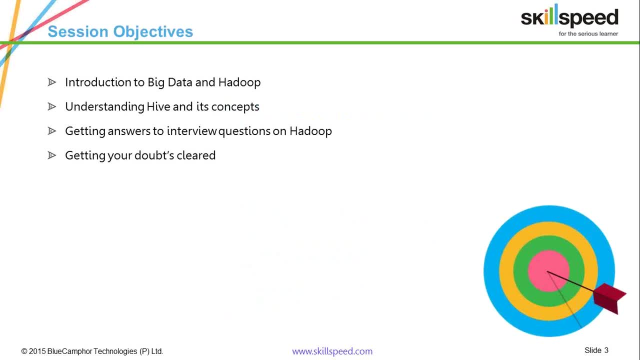 And I know for sure that most analytics company are using Hive- okay, Hive in conjunction with Python or Pygmy, and so on. Okay, Hive in conjunction with Pygmy, Python or R. right, That's what they are using. 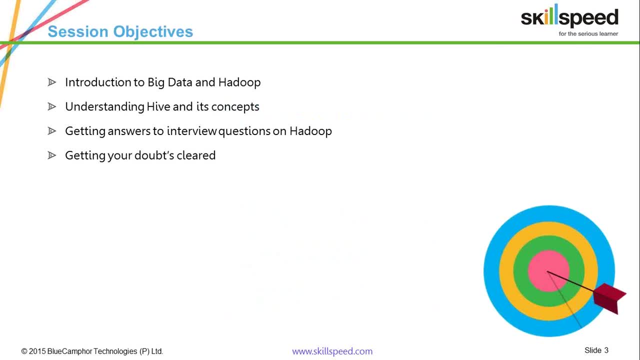 But majorly many of these companies. the reason why we came up with this course of okay, with this webinar- Big Data Analytics Using Hive- is because there's a lot of demand for folks who know Hive already right In analytics field. 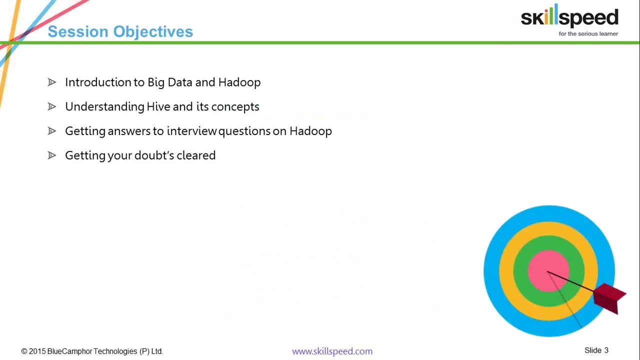 So that's where we came up with this whole idea of doing a session on Big Data Analytics Using Hive Now Big Data Analytics Challenge, Even before I go into details of Big Data, right? So what is it that we understand with Big Data? 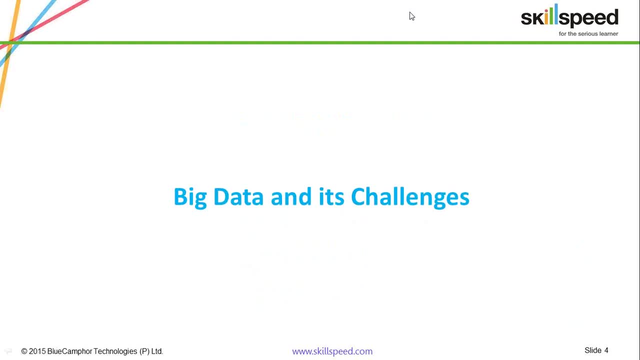 I mean there is a standard definition to it. but what is it that you guys understand from Big Data? If you can start typing here, you know I'll be able to read out. if I like some of the answers I'll read out to all. 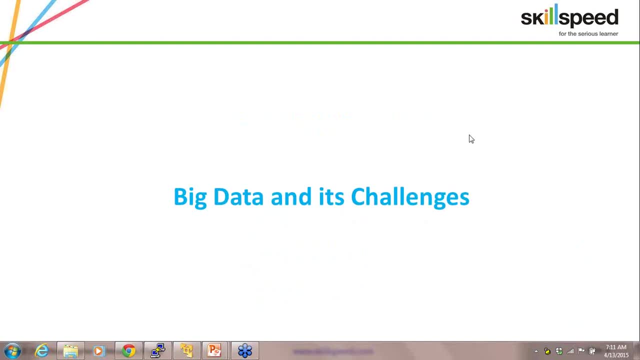 or else I'll just go ahead and start explaining: okay, Okay, so we've said it's unstructured data. Akshata says it's large amount of unstructured data. okay, So the question: we want to ask that so we can exercise. 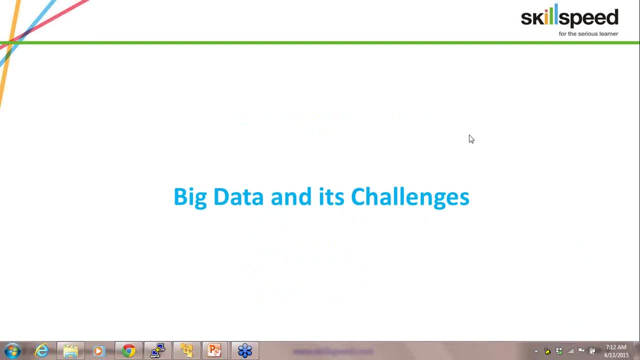 is such a data, not big data? Just think about that, ponder about that question. Big and discrete data, such as we saw a huge volume of data, lot of Amarnath says huge volume of data and so lots of volume with a variety of data format. 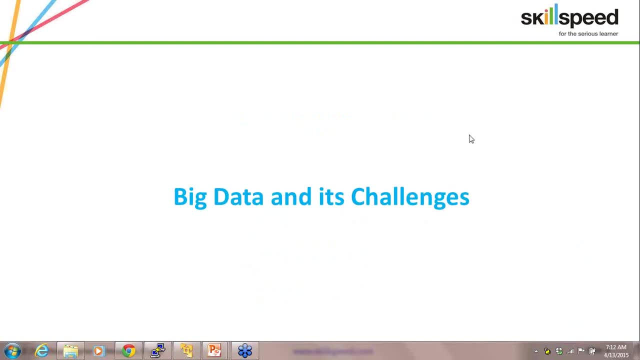 Well, Surya, you have given me the definition right: Volume, velocity and variety. okay, okay, Real-time data, so data with giant volume, variety and velocity. I understand it's mass amount of data set moving. 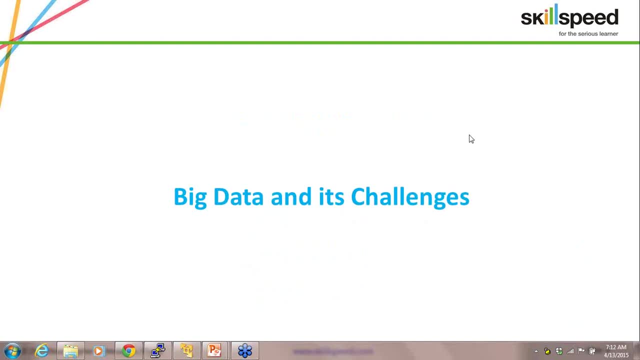 See, all of you are correct. Abhijit says any analysis which cannot be done with normally available technologies okay, And Vamsi master data MDM says Vamsi, okay, Okay. so I'm going to discuss some of the myths. 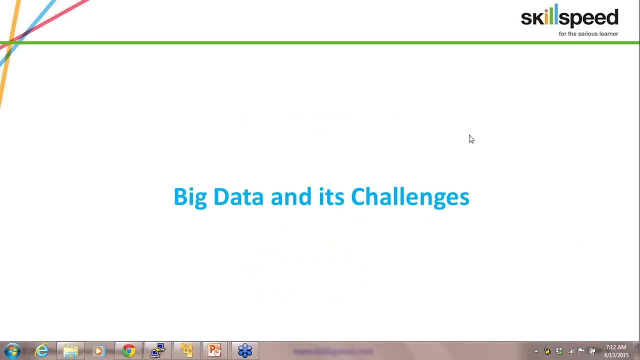 relating to this data. okay, That's why it was very important for me to know your thoughts on this. Any kind of data says Siva, which is huge volume and can be converted to information. It's large amount of unstructured data. 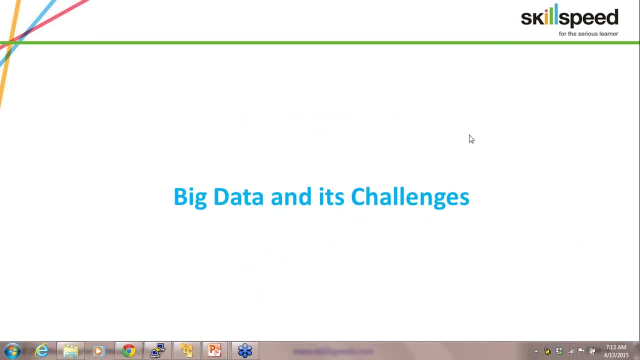 data generated at high speed. Okay, okay, Anshul, Now there you go right. All of you guys are correct. I mean, to a large extent you guys are correct, But big data is not just about data, okay. 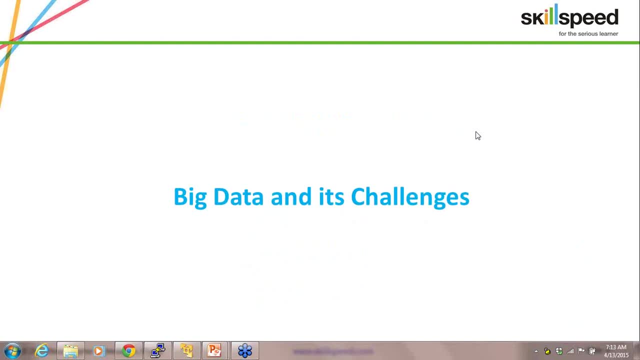 It's not just about large amount of structured or unstructured data. It is a humongous amount of data. That's well, that's good. But it's not just the data, right? Let's say, for example- I'll give an example. 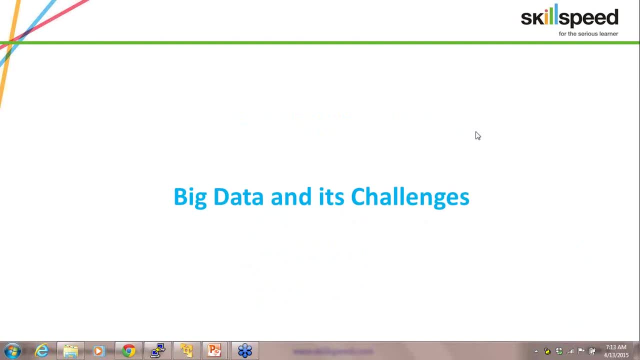 stating that, let's say, I have a GB of data which resides in my tape right from 1930s and then there has been no change in that data whatsoever. or 100 GB of data. Let's say, for example, I have 100 GB of data. 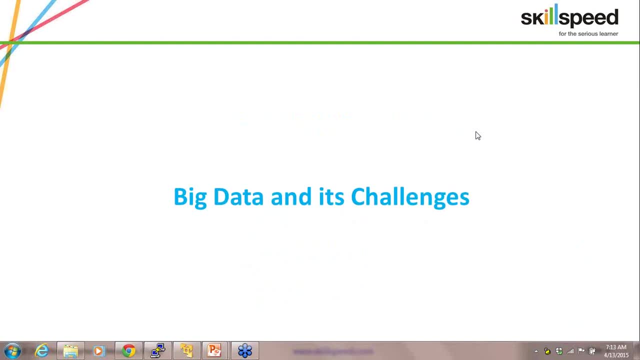 since 1930s and 40s and there has been no change in that data since then. That's a huge volume of data, but does that qualify to be a big data? I don't know, I don't think so. 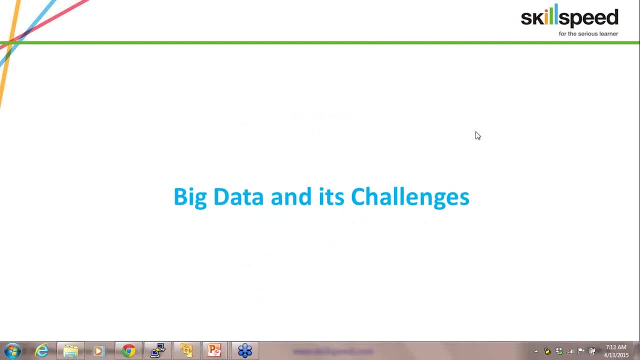 But then let's say, for example, I have a GB of data and yesterday I had a GB of data and I know for sure that today there will be some increment in that data over a period in time Absolutely unsub. 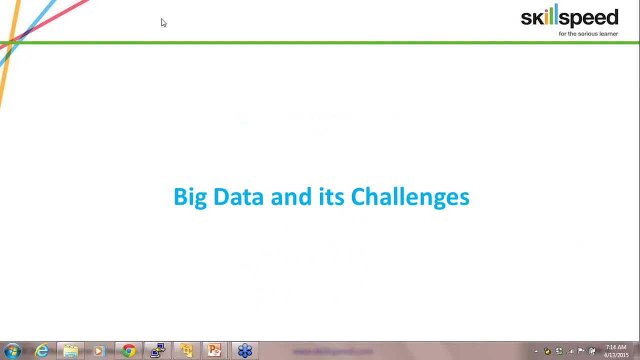 Okay, I'll get to that. So let's say I have a GB of data and I have a probability that in future that data is gonna increase and increase by MBs, KBs and GBs to become so huge and humongous. 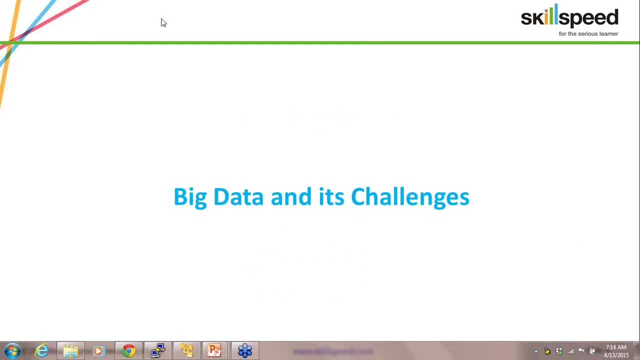 that you will not be able to deal with it. If you have that foresight, if you have that probability, that data can be considered as big data. So it's not just the volume. Volume is one thing, but you need to have velocity associated with that volume. 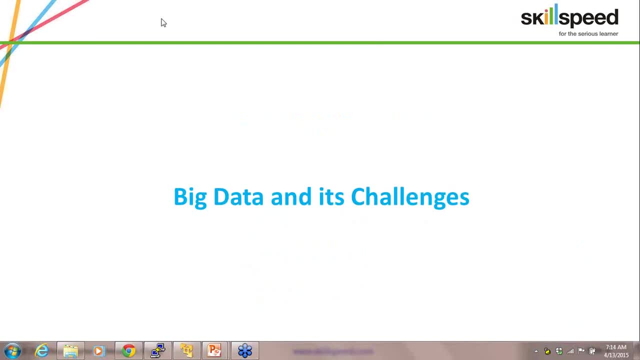 and that's when it's called as big data, And not just that, it's not volume and velocity. It's not one type of data. It's not only structured or unstructured data. It can be structured data. It can be semi-structured data. 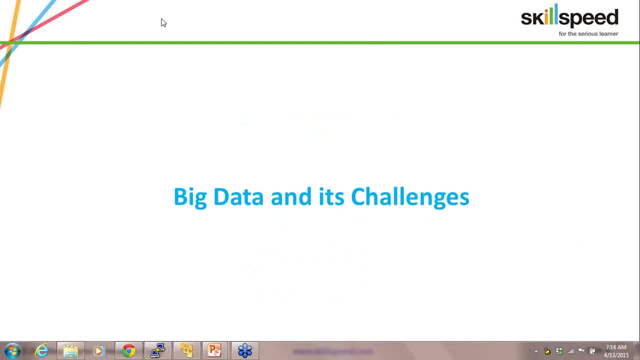 It can be unstructured data. Now let me go into, let me deviate a little bit. Okay, so let's say I have a GB of data and I have a GB of data. Let's say I have a GB of data. 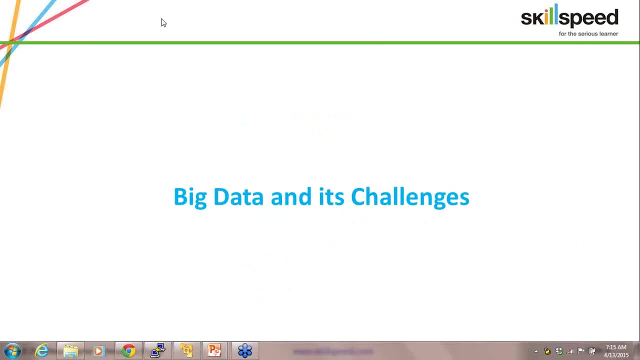 Let's deviate from topic a little bit and let me talk about what's structured and unstructured data. Now, structured data: I'm sure all of you- either you are studying or either you are working right. And if you are studying, 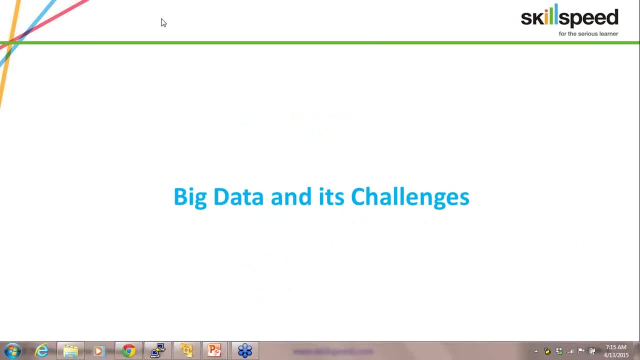 you would have read a little bit about DBMS Database Management System. If you have already studied and working, you definitely know about DBMS. right? You have at least fired one query in your life. You have at least said: select star from table right. 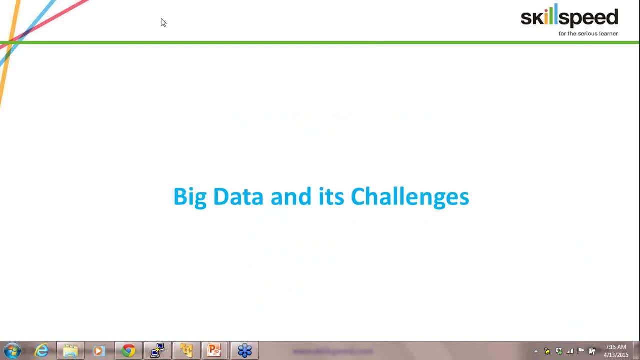 You would have absolutely done that, And even if you have not done that, that's okay. You know, select star from table would retrieve the data from table right In your database. normal databases like Meet, Oracle, SQL Server, MySQL, DB2,. 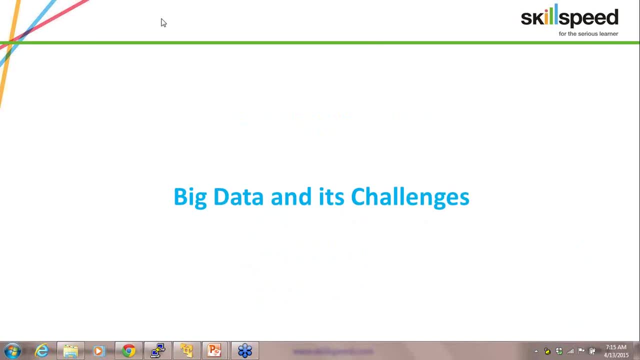 Teradata, so on and so forth, right Wherever you use a query language in order to pull a data that's called as structured query language. And if you have pulled this data from various different sources, right Those data residing in these relational databases. 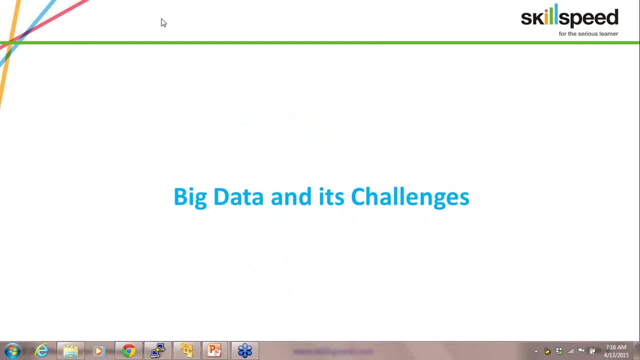 are called as structured data, right, So they have a particular format to it. they have a table structure, they have data inside it, So they are nothing. but they are called as structured data. What's unstructured data? Any data that you see online, right? 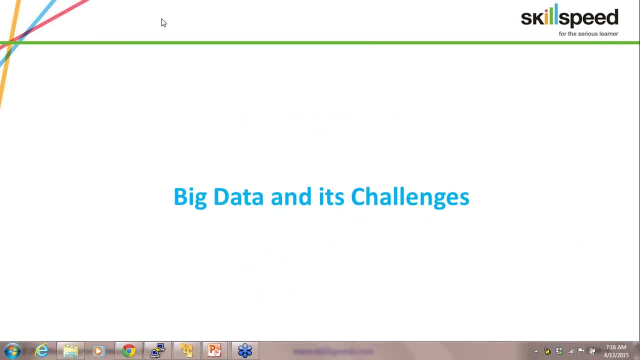 Be it text data, be it RFIDs data, be it the data that is being sent from Mars by robot- right, That's unstructured data- Be it the data from weather forecasting system, where MBs of data are generated every second. So be the data, MBs and GBs of data. 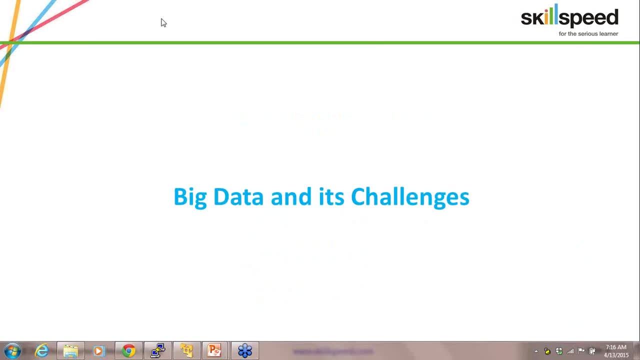 are generated every second. That's big data. Some of the space exploration, deep sea navigation system which generates data. that's unstructured data. Your music file, your videos file, your Facebook uploads that you have done right. How many tons of data that you have uploaded so far. 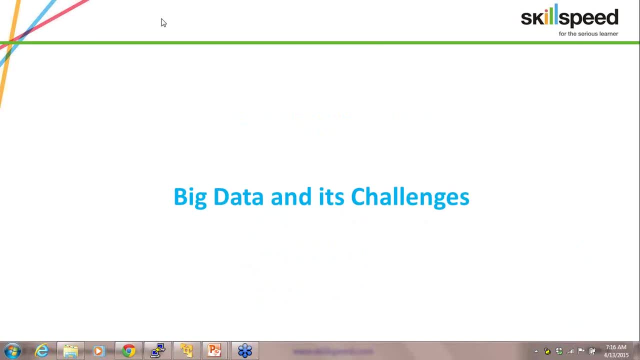 I mean personally. I would have hundreds of pictures there and even videos in Facebook. I'm sure all of you have an account in Facebook and Twitter, So just think of the amount of data that you are dumping, dumping into this system. 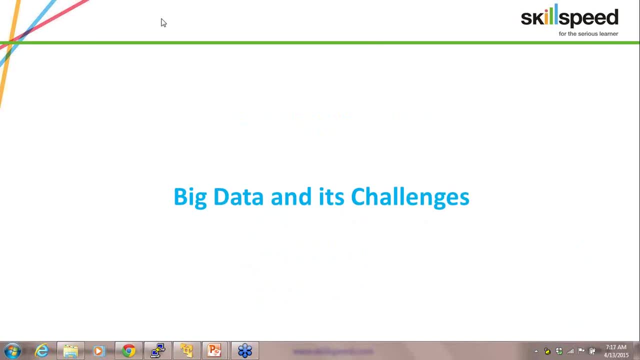 They all constitute big data and they're all unstructured. So picture is unstructured data. So that's the difference between structured and unstructured data. Now, coming back to the main point that we were discussing: big data is not just about volume. 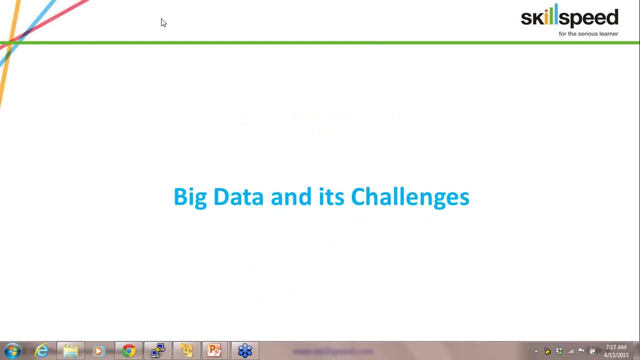 It's about volume velocity, with its growing and variety. Volume, velocity and variety: This is the three V definition of big data. Now there is one more V associated with it, which is called as veracity of the data, which means to say that I mean IBM added it later on. 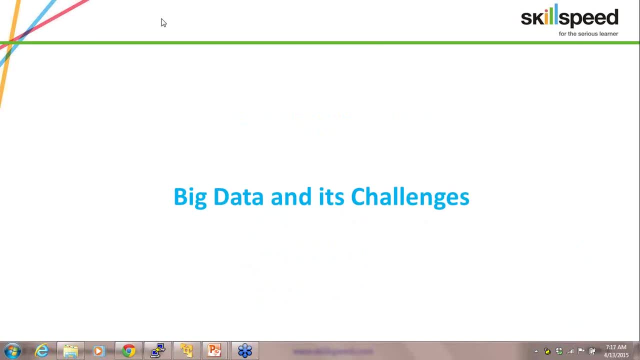 So veracity is nothing, but you'll have to have proper data in order to do big data analytics. But then, if you have data, I have the means to make it proper. So that's what I feel, So that's why the three Vs remains the four V people. 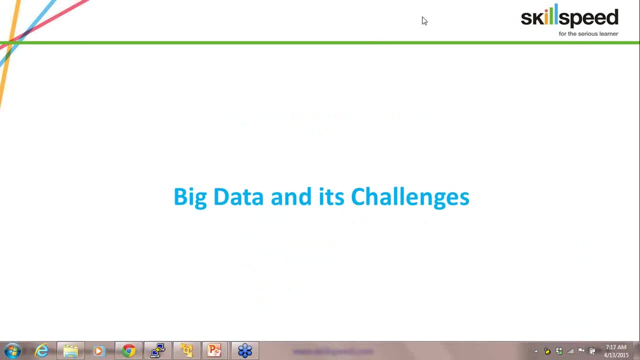 Some people use it and some don't. So that's the definition of big data. Okay, Akshata says: what about page clicks? right, This is a very big thing which is coming up. Akshata, You are talking about click stream data. 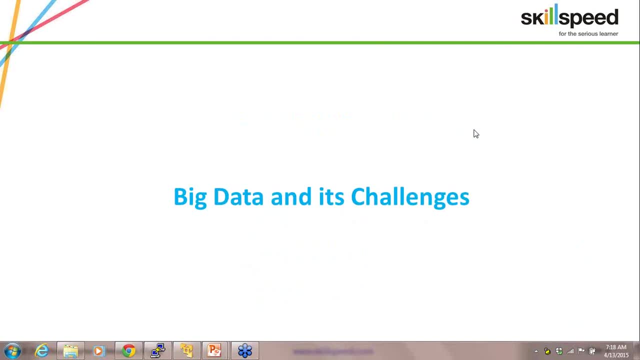 And we saw that's right: File plus web plus RDBMS, plus zips, plus images, et cetera, et cetera, absolutely right. So, Akshata, to answer the question right. 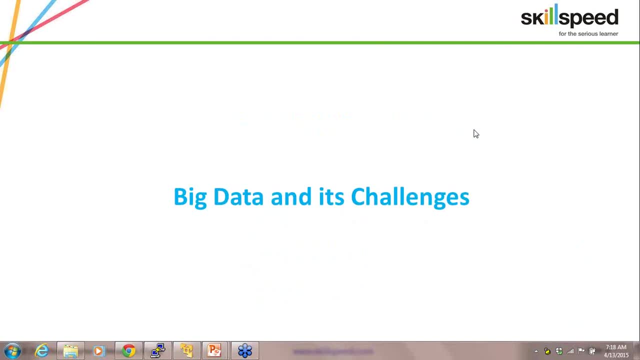 Click stream data is coming in a very big wave in this industry And people with experience in customer domains who do analytics in click stream. they're very high in demand. Sentient data- absolutely So. the sensor data and volume velocity. volume velocity, variety and veracity- Siva. 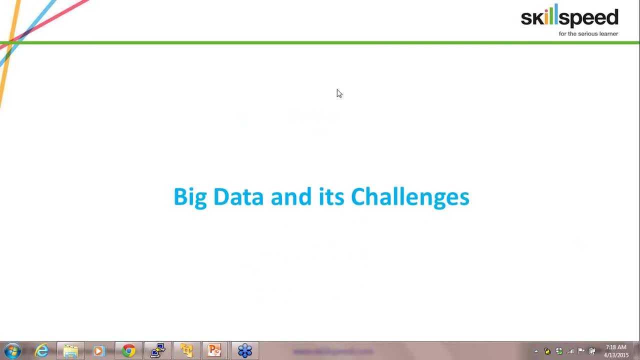 It's volume, velocity, velocity, variety and veracity, Yep, yep, Kumar. web server log file. These are classic examples that we are all talking right: Web server log file, huge amount of Apache logs, et cetera. 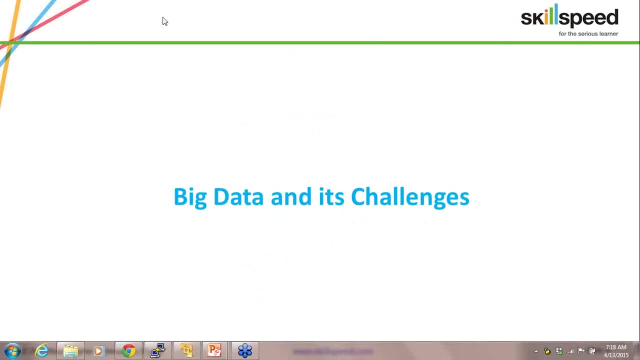 that we process and so on. So these are actually. this has become like hello world of data: Big data programming, right Processing, web server log file, your word count problem. They're all like hello world program. They are the ones with which it all started. 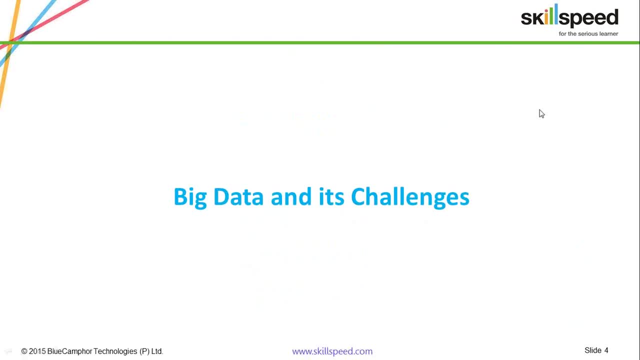 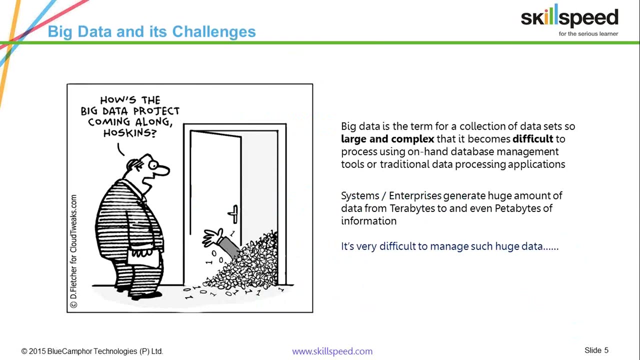 Yep, actually, yeah, click logs as well. So moving on. okay, guys. Now big data and its challenges. Now I've talked about what comprises big data. right, Huge amount of data, volume, velocity and variety- That's big data. 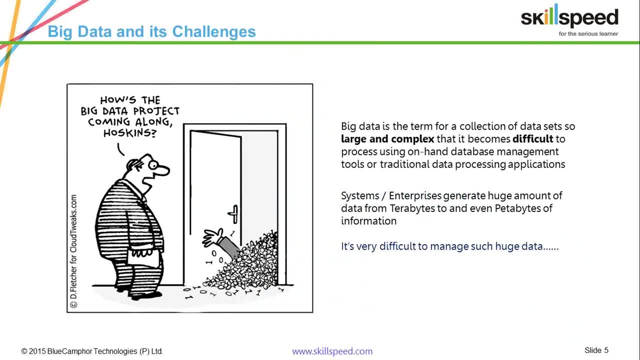 But what are the challenges associated with it? Big data One, first of all. we have tons and tons of data, but we don't know what the data help us. For example, let me talk about one of the industries that I was in long back. okay, 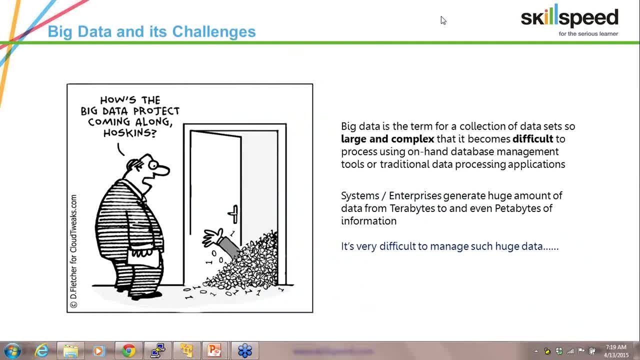 So in that industry- it was a manufacturing industry and, in that particular place, very big organization- They had tons and tons of data. The company was there since the 70s and 80s and tons and tons of data, everyday data. 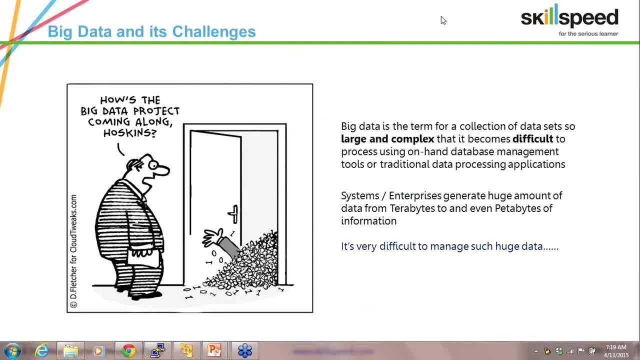 They used to sell something, They used to store those information, But because of lack of any processing or because, I would say, lack of any powerful machine. see, there are servers, right, There are million dollar servers. You can have hundreds of servers, so on and so forth. 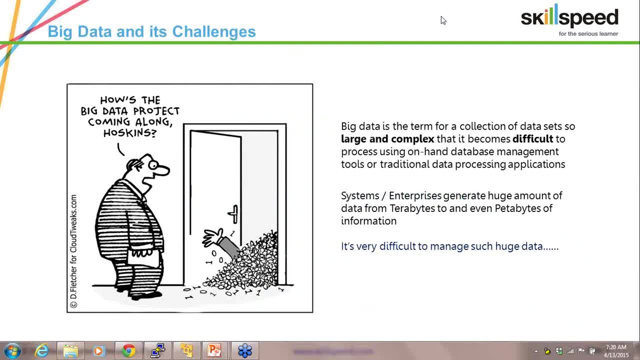 But then at a certain point, right, your server will also be able to only process so much of data. Let's say, for example, my laptop is 16 GB memory, Intel i7 processor, so on and so forth, right? 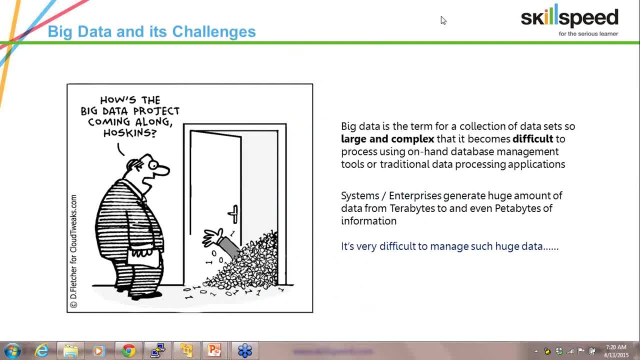 I'll be able to process, let's say, 100 GB of data. Let's say I am able to process 100 GB of data. Extrapolate this to a server, Let's say, that has 100 GB of memory RAM. 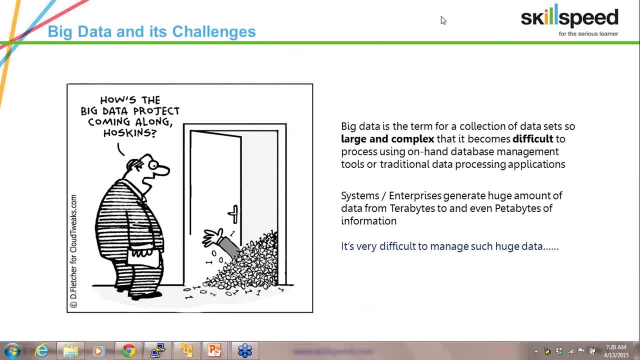 and then I don't know, quad-core, octa-core, what not processor they have, But eventually, at the end of the day, it will have some limitations, right? So, going back to the organization where I was working, that huge amount of data, tons and tons of data. 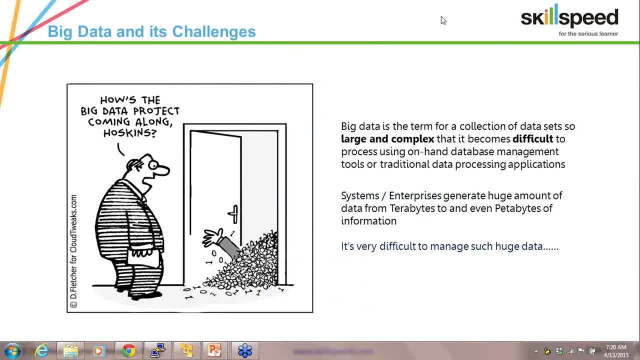 decades of data, 40 years of data, but then, when we were building a prediction system on top of that, a forecasting system on top of that, we were not able to use them all right. The simple reason being is that our hardware 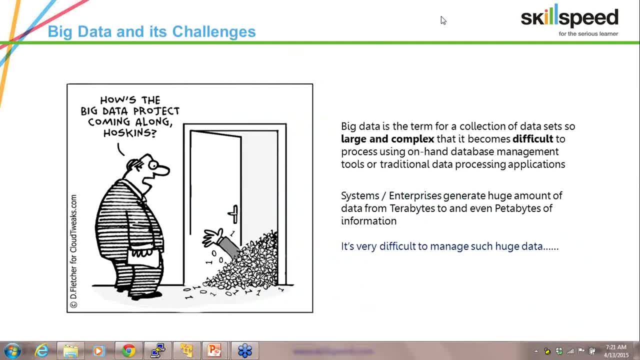 and software were not capable enough to handle such huge load of data. So what we used to do is we used to take last three years of data and, based on that three years of data, we used to write programs, you know, which would eventually do predictions. 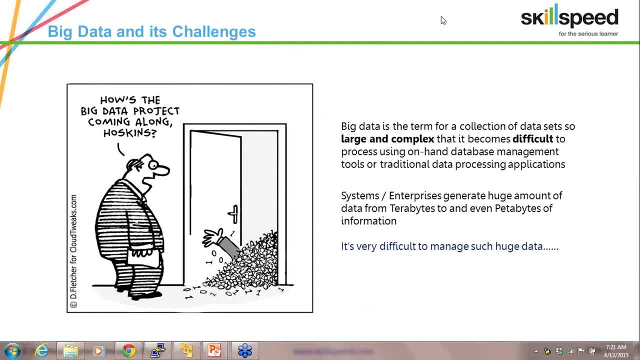 which will eventually do forecasting. Let's say, for example, I sold an X item last year and last to last year it was 1.1 GB, And prior to that, 1.2 of X, and so on and so forth. 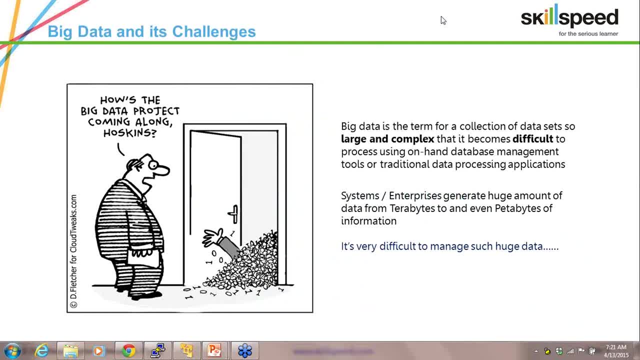 You know, we would just use those data, we'd just use those numbers in order to write our prediction algorithm. But with the advent of big data, everything has changed. Now they are able to process 30 years of data, find a proper pattern to it might actually, you know, 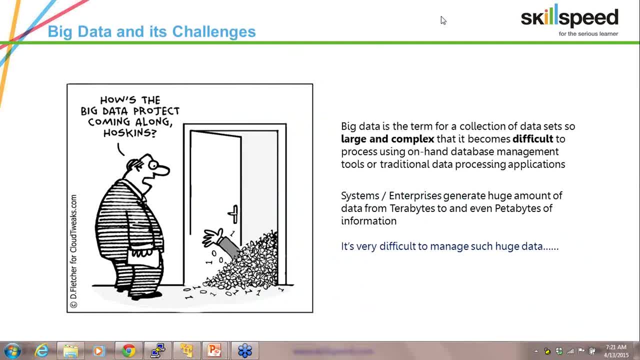 so this is what happens in the manufacturing industry. okay, Some years are good and some years are bad. It's almost like a sinusoidal wave, right? It's all like everything goes around in a circle. It started with a good year, next year it becomes bad. 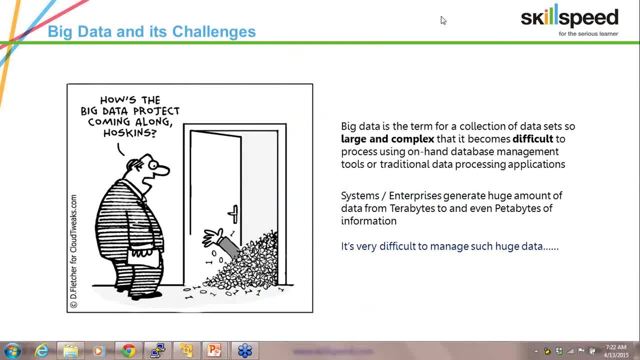 third year, again it's good, fourth year, and so on and so forth. Now, if I did not have this data, what would I do? I would just look at my sales data and then say, okay, fine, this is the sales that happened. 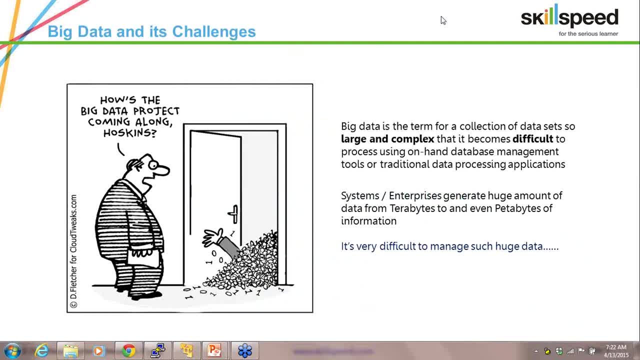 a couple of years back and this is what might happen this year. right, But we would not be taking into account all the different features like, let's say, the inflation, the markets, the tragedies that happened, these natural calamities that happened. 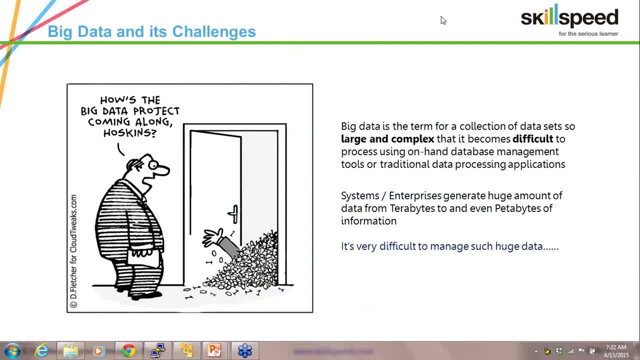 We don't take into consideration those features while we are doing actual forecasting right in those systems. Most of the organizations have changed, but there are many which have not changed. I mean, I think the big ones have changed, but then the medium ones and the smaller ones. 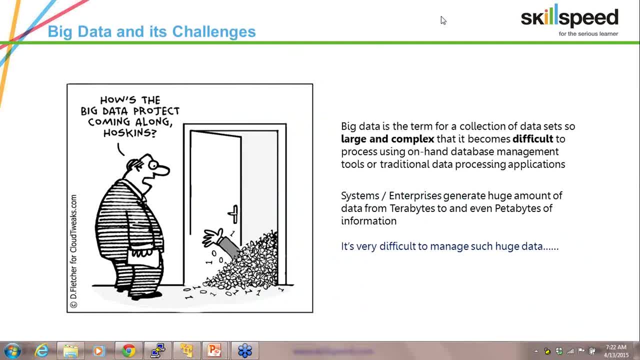 have not changed this year because they still don't know as to how to use big data in order to optimize the whole processes. So big data and mining this big data and challenges now having this pile of data and trying to bring out something or something useful out of this big data. 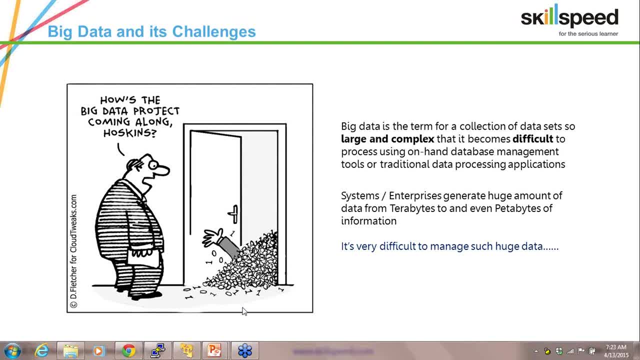 is also called as data mining. okay, So it's more like, if I take an analogy, it's like a diamond mining. right, You go, you start, you know, digging the whole hill or mountain. you start digging the hill or mountain. 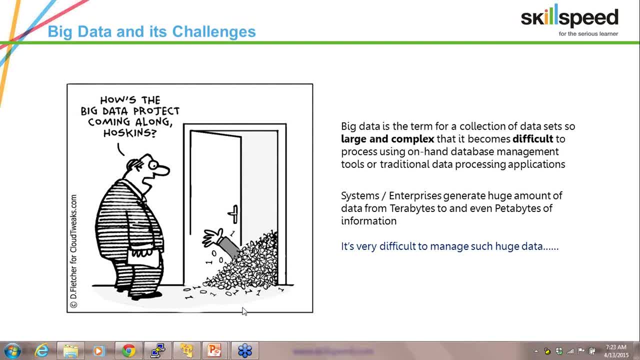 and eventually you get a stone. you don't know whether that stone is diamond or not, but then you polish it, you slice and dice it, you mine it and eventually there will be something you know, which you get, which is diamond, after having you know. 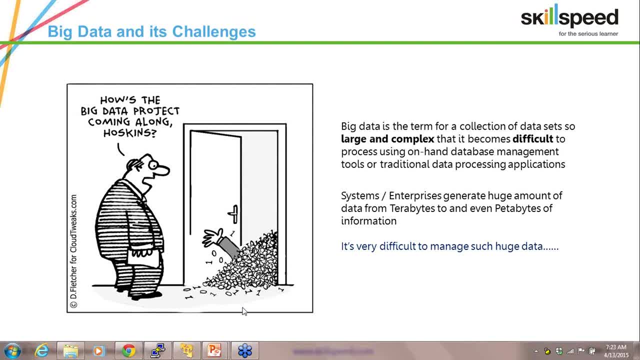 cut it after having processed it a lot, right? So similar thing with big data. you will get data which is in extreme raw format, right? You don't know what to make out of it. You will pull into those data. you will cleanse that data. 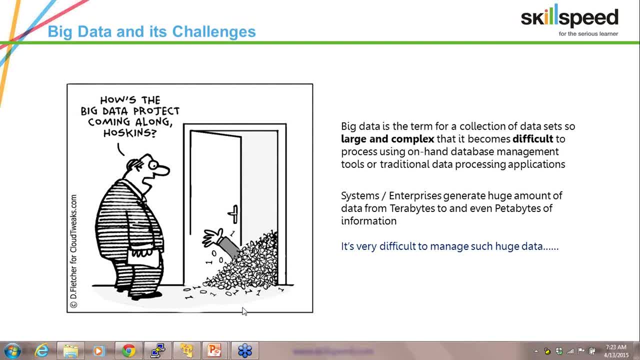 you will slice and dice those data, you will fill all those unfilled information over there and eventually you will have a set of data Now which will be fed into some kind of machine learning or artificial intelligence right Or artificial intelligence program. 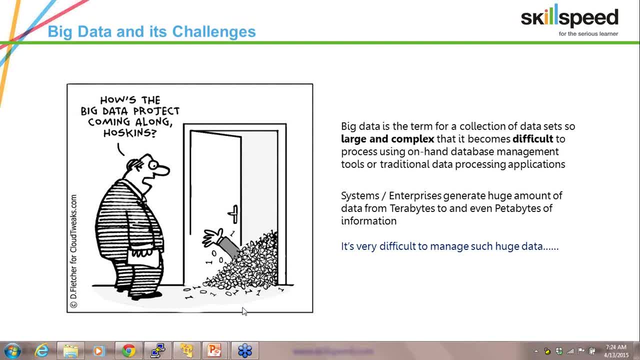 and eventually you will have a pattern or a prediction module in the end, right? So that's about big data, its challenges and how do we mine that? Yes, finding amounts and large amount of data, absolutely, et cetera. 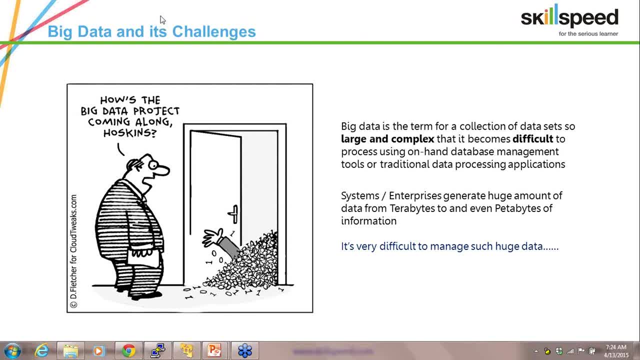 Now, this is done using big data, okay. So whatever I just said, pulling, you have big, huge amount of data right. Pulling this different data from different sources, like, let's say, for example, your picture information, your text file. 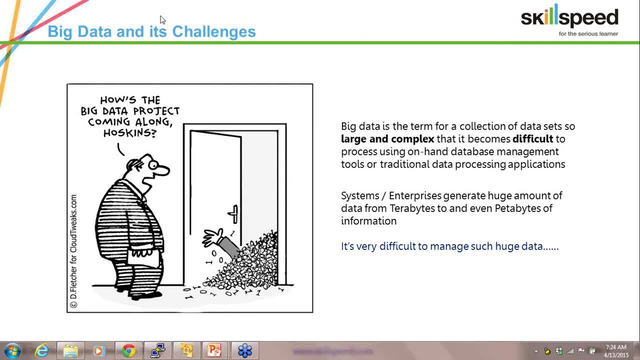 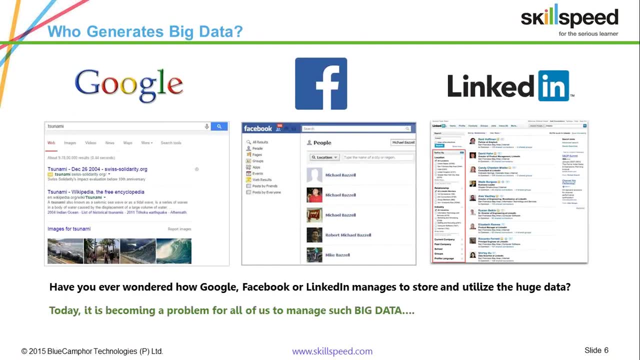 your so on and so forth. right, All those information. you pull in those information. and then who does all this processing for you? It is the big data or it's Hadoop which does this processing for you. okay, Now who generates big data? 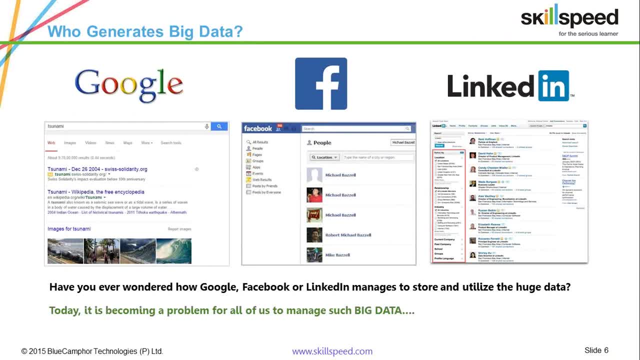 Your Google, Facebook, LinkedIn. that's what I gave an example: Your sensors, your RFIDs, your deep space data. right, Yes, You see. navigators, Mars, a robot that went to Mars, so on and so forth. right, 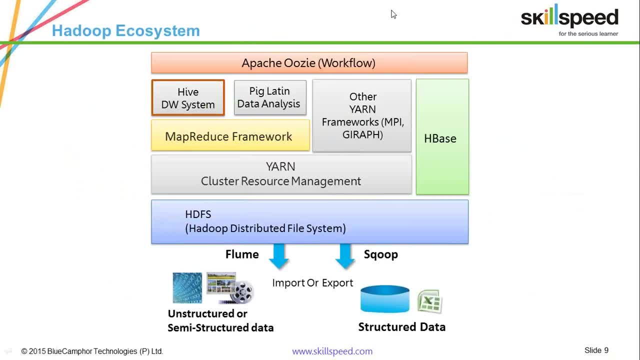 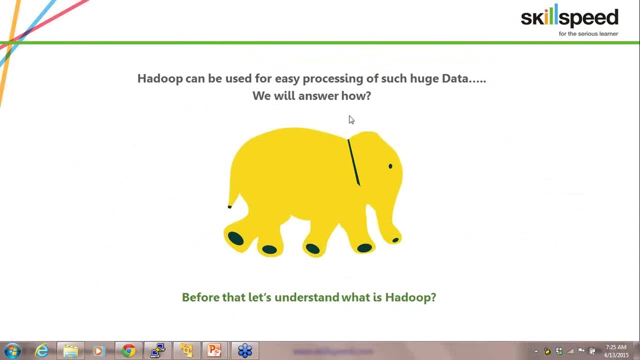 We all generate big data. Now, oops, let me go back Now. yep, yep, and so we can also review what people. that's what I would also talk about: sentiment analysis. This is one program that I wrote, right. 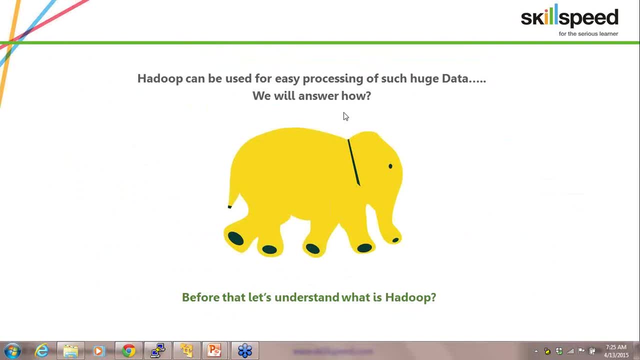 Actually, I was asked to write a program wherein for famous individuals, big network individuals, I have to pull data from all social media for them, be it Facebook, be it blogs, be it Twitter, et cetera. I had to pull all this information. 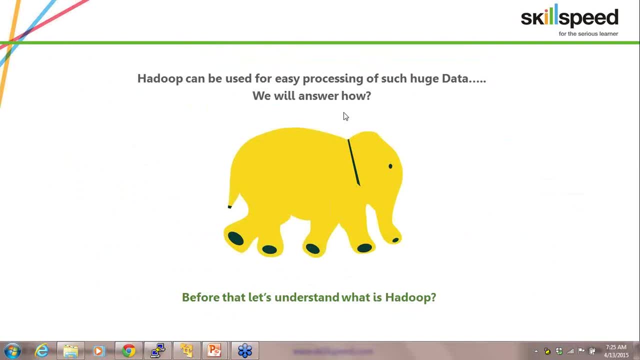 First of all, pulling this data from different social media websites and even blogs is not that easy. It takes a lot of effort, Most often than not, when you are writing a printable, it takes a lot of effort When you are writing a predictive module or when you are trying to write a machine learning. 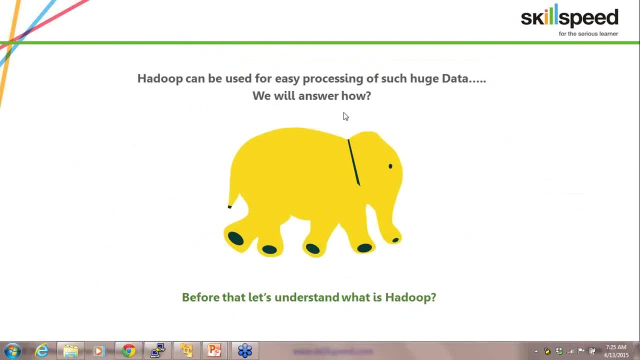 algorithm, the maximum amount of time you spend is in collecting data and cleansing it. That's the 80% of time that you spend your time. 80% is spent on just collecting and cleansing the data, and it's just 80% where you actually 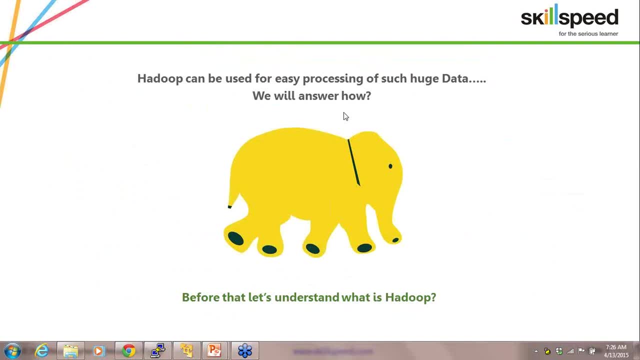 write an algorithm. So this 80% piece is what Hadoop offers us. So when I was told to do this to find out, let's say, 10,, 20 people, a big network individual, I had to do an analytics on them to find out what people think about them. 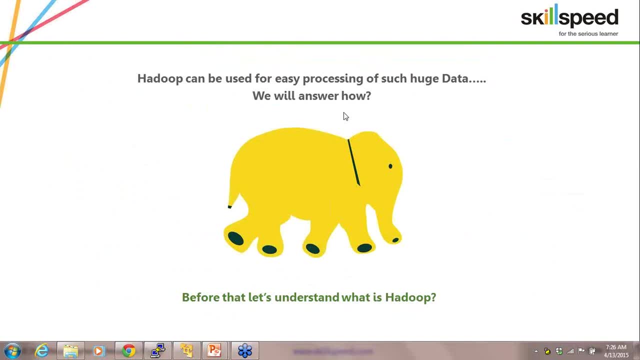 Okay, What are the tweets they have? what do people write about that? whether people have positive opinion about them or negative opinion about them, so on and so forth. Image building is a big exercise when it comes to big business. If your image is bad, your business will be doomed eventually and there will be negative 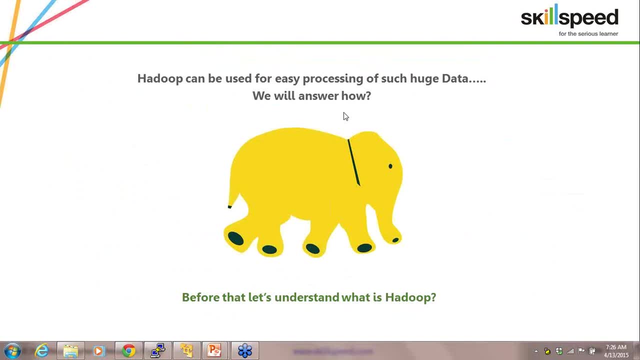 sentiments in the market and eventually your company will go down. So I was asked to collate this data, find out, do some sentiment analysis, and I did that. So I collected data from Facebook, Twitter. I went to multiple places in order to collect the data, even the text data that they had. 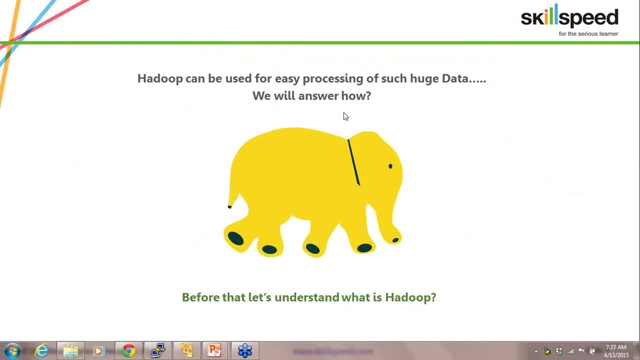 lying in the system. I took out all the data and then told them that this is what the people are saying. this is the adverse feedback. this is the good feedback. now, based on this, you take your action. So that was quite an interesting program. 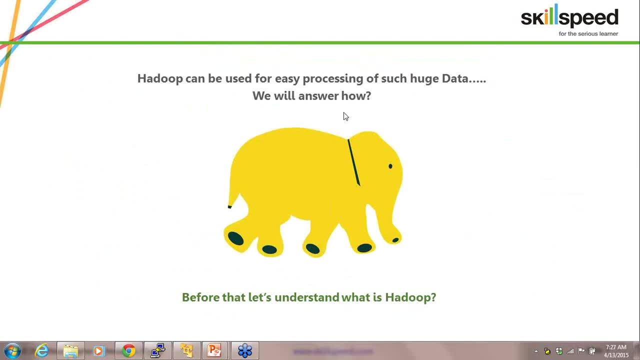 Can traditional warehouse be used in big data environments? Absolutely, Sudip. You can plug in and plug out traditional data warehouse. No, it does not need a complete revamp. There is something called a scoop. You just hit the traditional data warehouse, pull the data inside big data and then process. 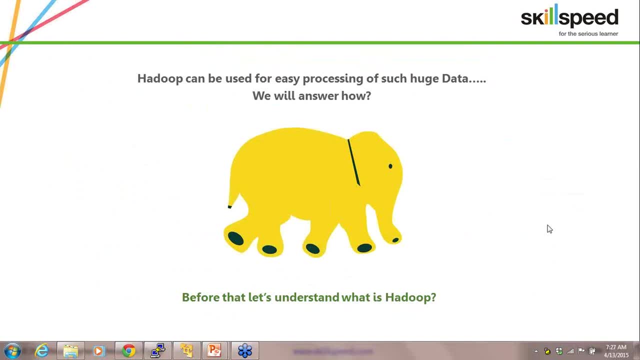 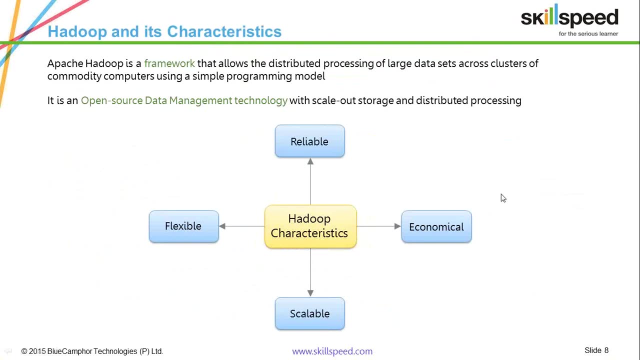 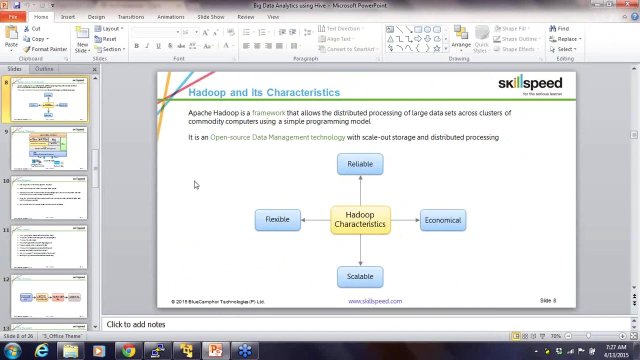 it Now. Hadoop can be used for easy processing of huge data, will answer how right. So let's look into some more details of this Now. even before I go here, I will talk about this and then for three minutes I'm going. 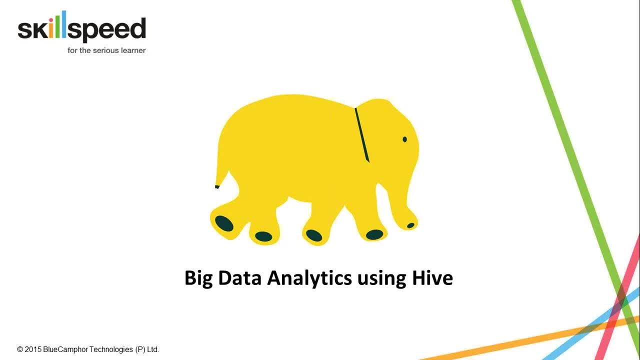 to talk about this. I will straight away move to something which will actually be helpful to you. Now, these are a lot of theories that I'm talking about, a lot of good stuff that I'm talking about, but it will actually not make sense until and unless you are able to actually 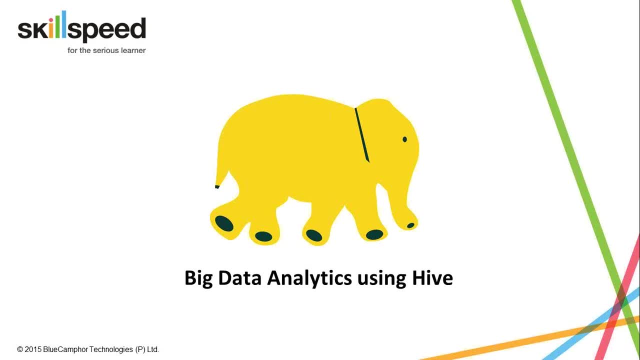 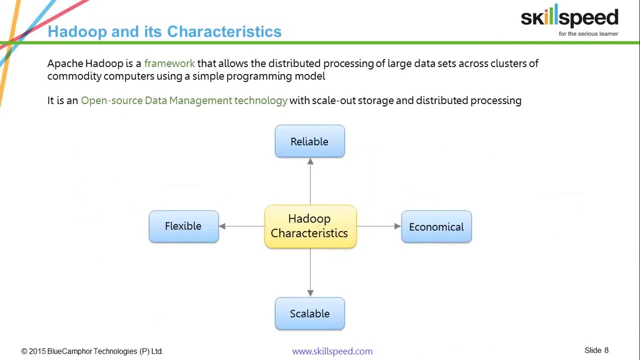 see it and feel it as to how it looks like. how do I process huge amount of data, right? So now let me go here: Hadoop and its characteristics. The beauty of Hadoop is that it's economical, Like I've been telling you that all these companies use this big server, right. 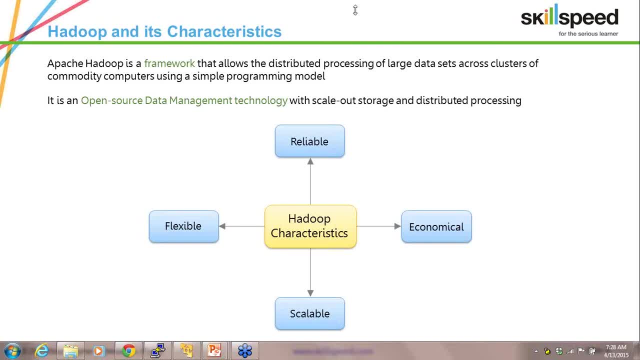 You might have seen this, All of you, right, If you are working in an organization. okay, before I go there, let me read what Surya has written. So your machine learning program and you can use it with big data. 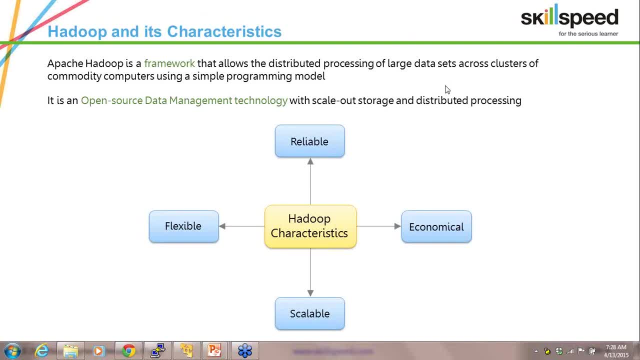 Absolutely, Surya. Okay, Now I was talking about million dollar server, right. That is what big companies can afford. I mean, what do small companies like mine right, do when I don't have that much capability or when I don't have so much of money? I don't have million dollars with me. 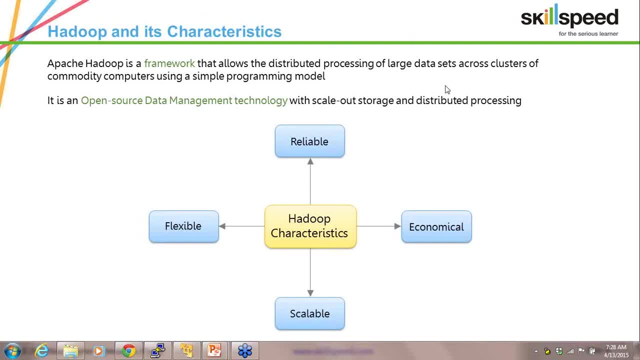 I just have a few thousand dollars, right. What do I do? I would rather buy commodity hardware, large number of desktop type hardware, right, I can still configure a good desktop for around 300, 400 USD. So if I can pull in large amount of desktops, connect it and then create an ecosystem, or 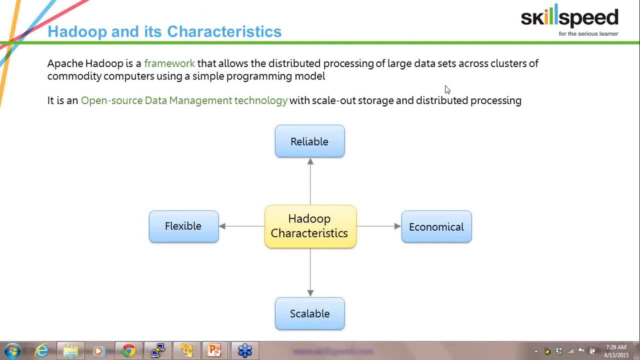 cluster of Hadoop right that and if that can give me performance as good as a million dollar server, I mean it's not bad right. At the end of the day, I am able to process huge amount of data, So Hadoop actually provides that. 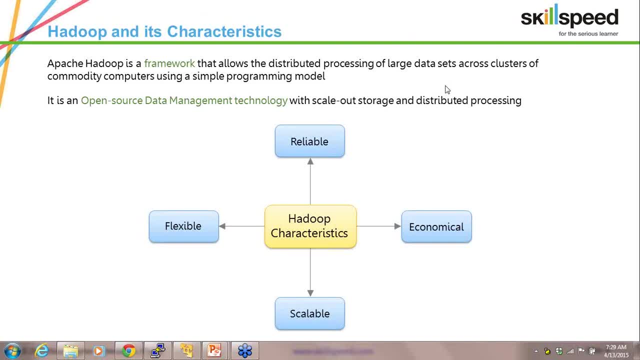 Hadoop provides parallelism using commodity hardware. okay, So that's what Hadoop provides. It provides you. it provides it lets you use commodity hardware as cluster of machines and then with that you are able to compete with those million dollar servers. 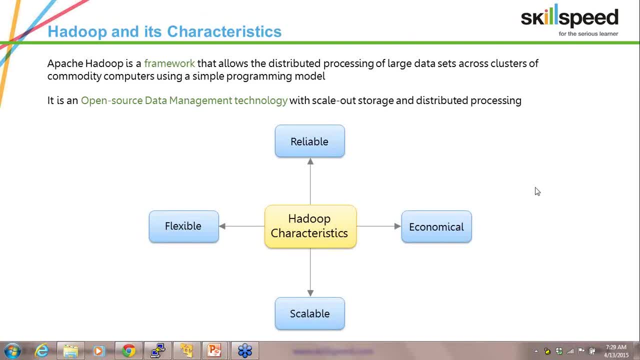 And I was talking about all of you being in some type, some kind of organization where eventually, every weekend or on any weekday, you get an email saying that the server is going down for so and so reason, for maintenance purpose, and you know you'll not be able. 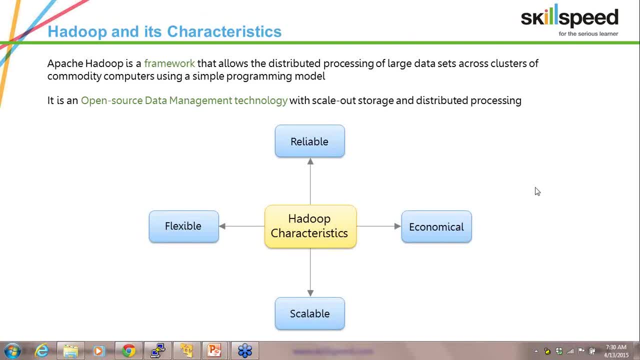 to access it for some time. There is hardware upgrade, there is software upgrade, there is some kind of memory upgrade, so on and so forth. right, All of you might be getting this email in your inbox once in a while. The reason they need to bring down the whole system is because that's just one server at. 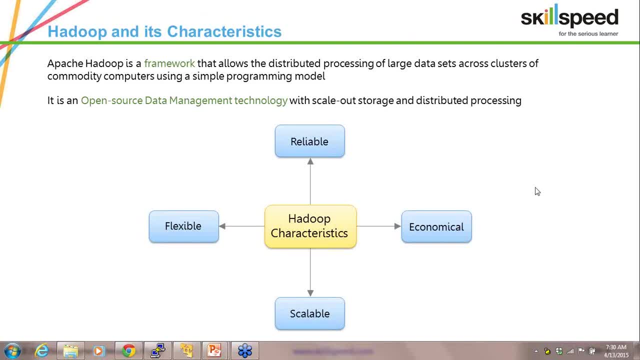 the end of the day, You add more memory, you bring the entire server down, you add more memory to it and then you bring it up. right, That's part of maintenance purpose, but with Hadoop you don't need to do that. 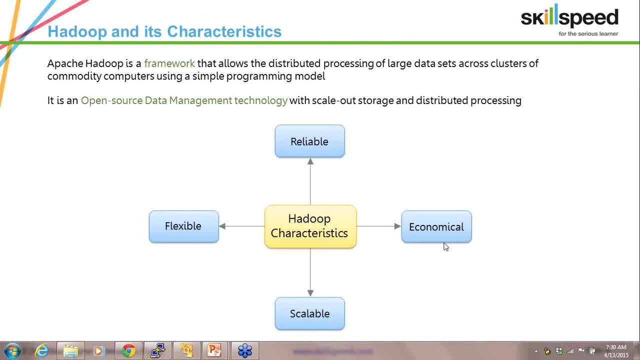 All you do is there is a plug-in and plug-out. Let me show you how to do that. okay, Let me explain to you guys and then let me go and show you as to how actually it's done. So it's economical. it's extremely scalable. I'll show you how it is. it is also flexible. 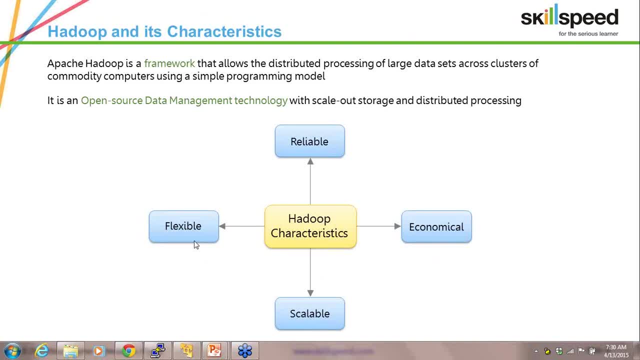 because you can plug-in and plug-out your system and it's extremely reliable because there is something called a system. There is a replication factor based on which each data, each piece of data, is stored in at least three different places. okay, Let's say you have one GB of data. that GB of data is stored in at least three different. 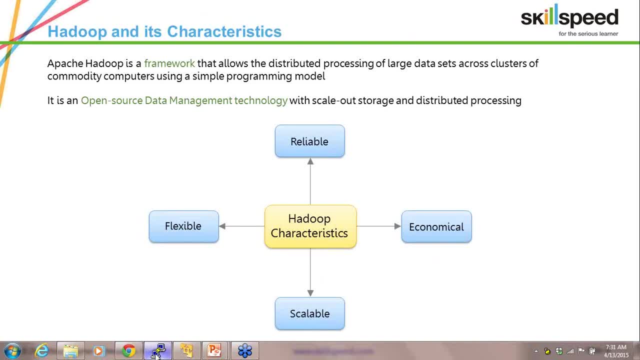 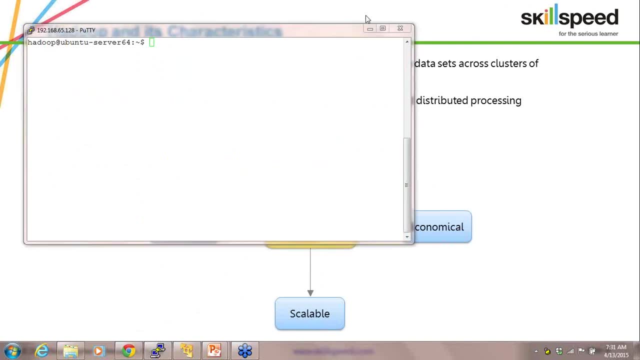 places, so that if one fails, the other still remains. okay, Now, let me straight away go here and let me clear it. okay, Let me show you as to how it works. Yep, yep, Aditya, I will explain to you as to how it works. 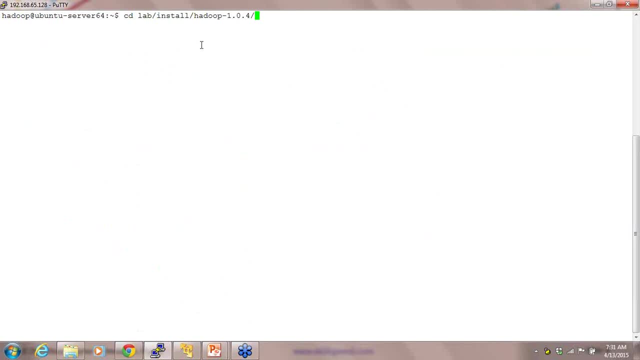 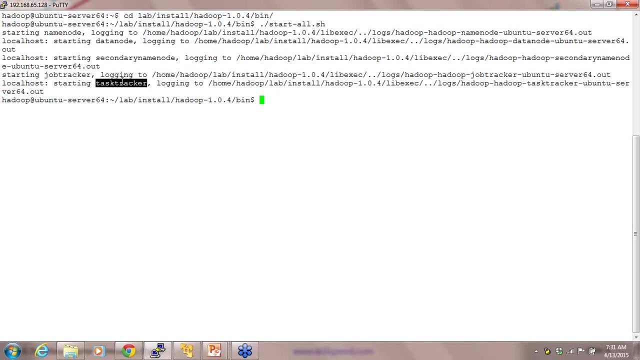 Now, now I'm starting Hadoop. okay, This is how I start Hadoop. When I say start all, it starts a couple of demons called name node, data node, the secondary name node, job tracker, class tracker. These are all the demons. 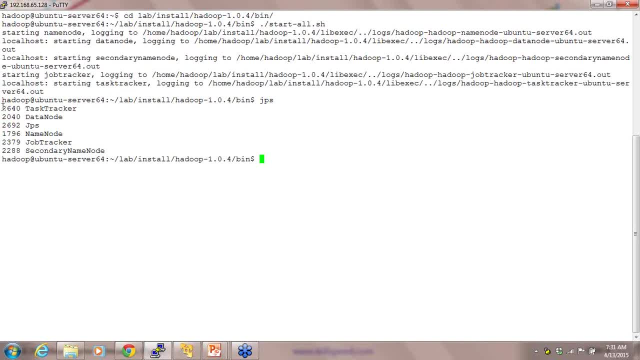 So when you do a GPS Java processes, it gives me all the demons, which has been started. okay, Once this is started, you know, okay, Even before I go in here, There are a couple of things that you would have seen in the past. 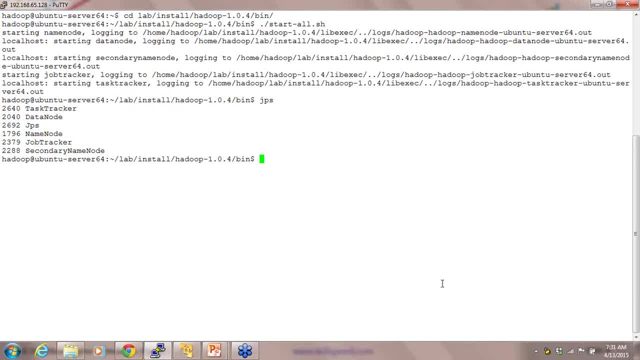 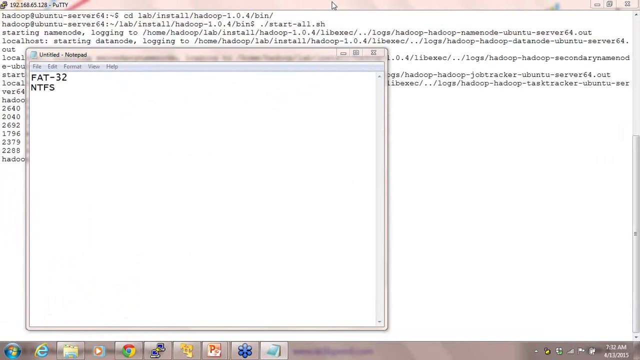 How many of you guys still remember FAT32, or how many of you know what an NTFS is? Let me say this: FAT32, how many of you remember this FAT32, NTFS and all Exactly Windows file system. file system is Dinesh Kumar Vishal. 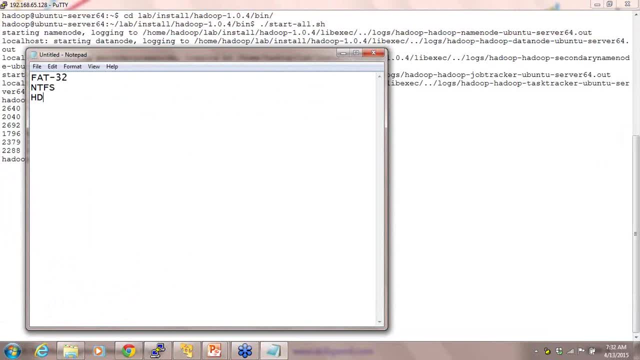 This is actually file system, so just let me extrapolate this to a distributed file system: it becomes SDFS. So SDFS was initially created by Google. this was Google file system initially, and then Google then made it open source, which became Hadoop distributed file system. 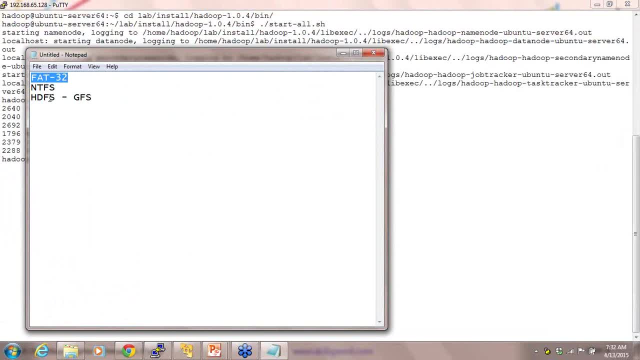 This is network file system. prior to that, this was FAT32, this was file system once upon a time, right, But this is. everything is NTFS. and now for a distributed environment. Google created something called as Google file system, Which went on to become Hadoop distributed file system. 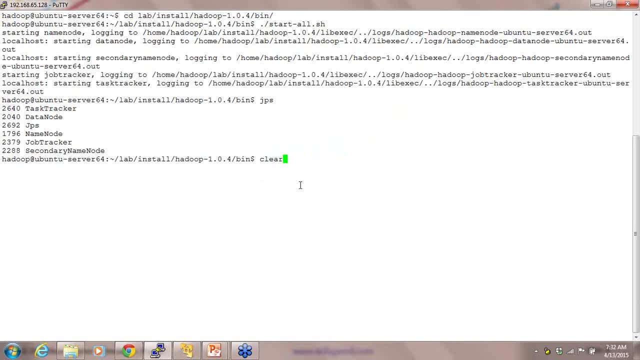 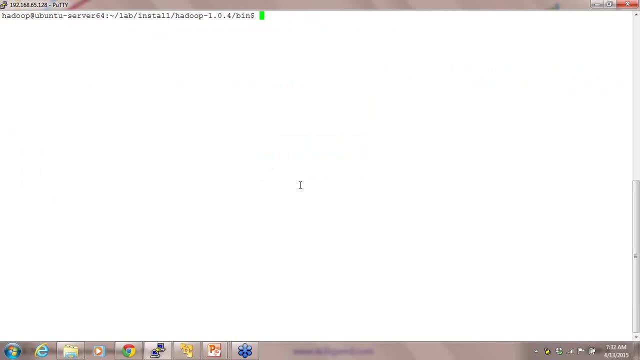 So now, having said that, let's go ahead and see as to how do I browse things in SDFS. Now, your file system. it resides in some kind of computer, right? Your operating system is on top of your file system. Your Windows was on top of FAT32, your Windows is on top of SDFS, so Windows is on top of. 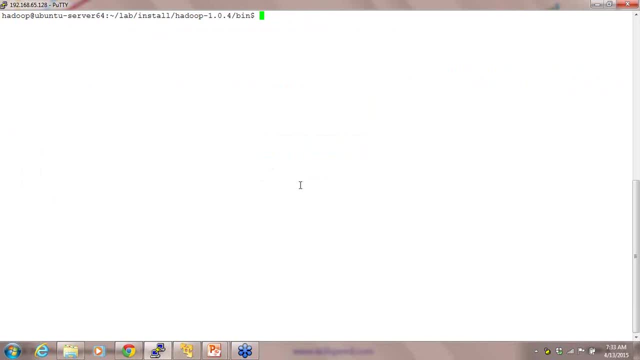 your NTFS And SDFS will eventually be on top of FAT32.. Right, It will eventually be on top of is on top of Linux. You see this, this is my Linux machine, right? Okay, inside my Linux machine I say Hadoop. 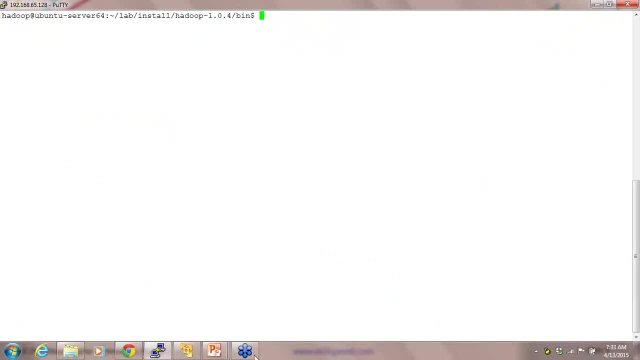 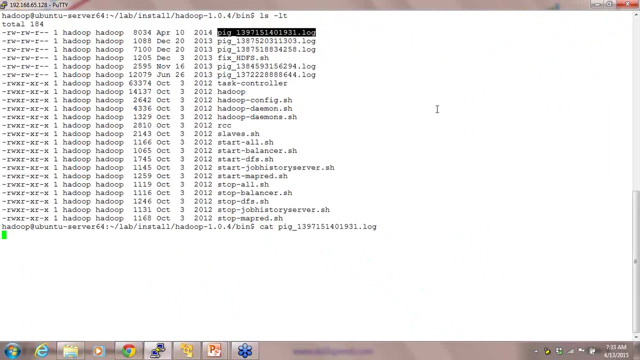 So how do I browse my Linux system? guys, If you have not seen this already, this is the simple stuff. This is simple stuff. okay, This is how I browse my Linux file system. right, I say ls, I say clear and then I say my ls-lt, which gives me this: I say care of log and. 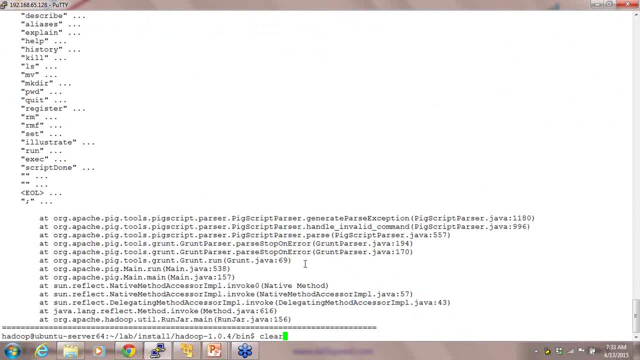 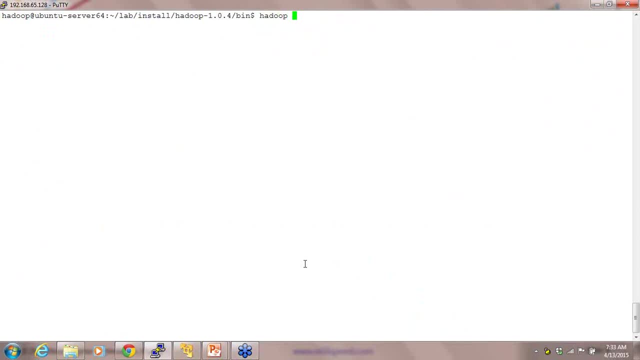 it gives me all the log related information. I again file clear because I want to clear up my so on and so forth. right, But how do I access or how do I browse my Hadoop file system? I say Hadoop fs-ls. 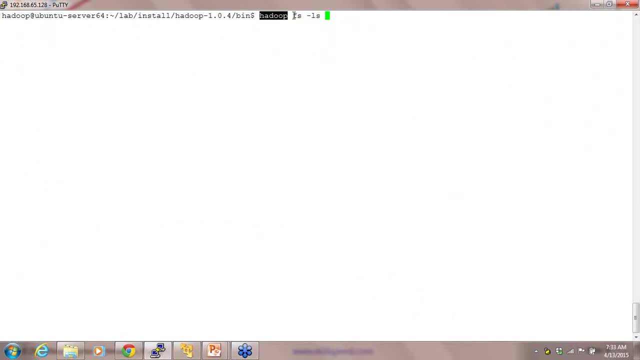 This says that I do not want to browse my local file system. I want to browse my Hadoop file system, Hadoop fs-ls. Now, there are a lot of concepts in the Hadoop, like MapReduce. there are a lot of ecosystem. 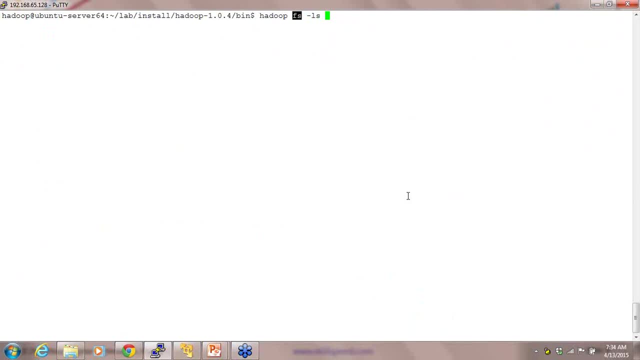 related tools in Hadoop right, Which which, Because of lack of time, I'll not be able to explain you that, but I want to straight away move to Hive so that I can give you a picture as to how you can straight away go. 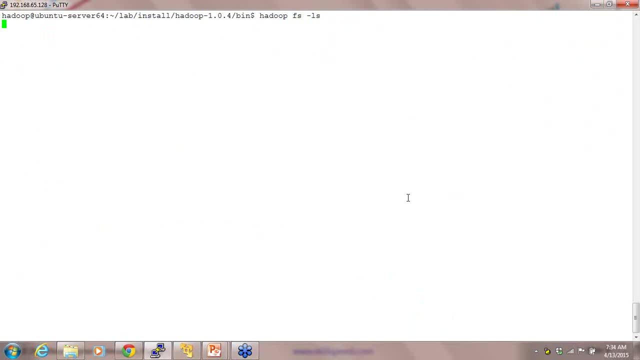 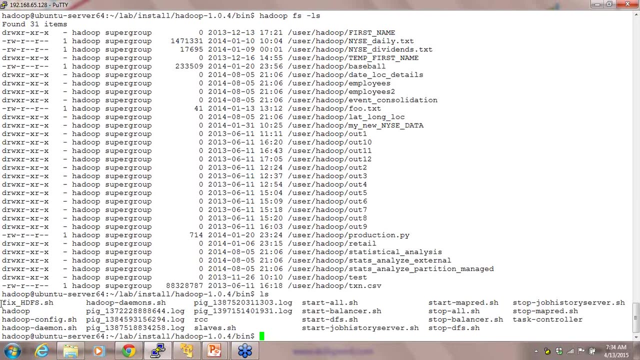 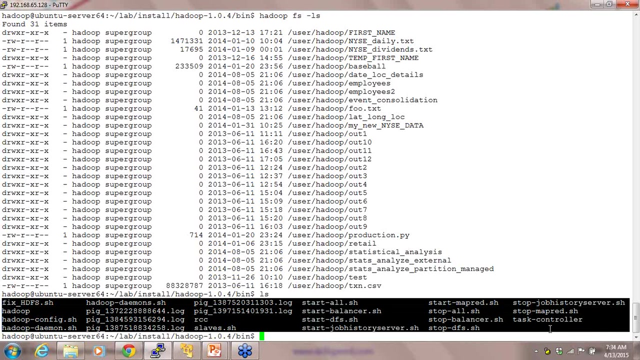 ahead and start using. When I say Hadoop, fs-ls, there you go. it gives me everything inside my Hadoop file system, Whereas ls will give you something which is in my Linux file system. So, with this example, you know that my Hadoop, or SGFS, resides on top of my Linux file system. 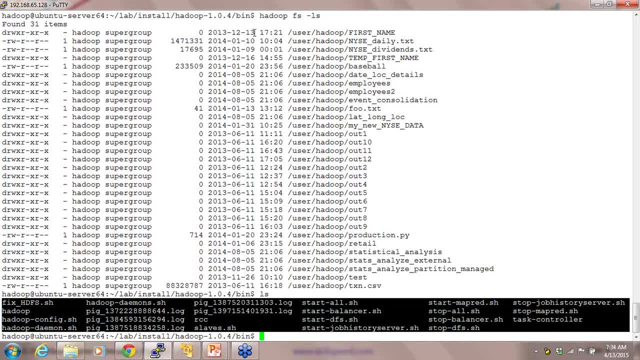 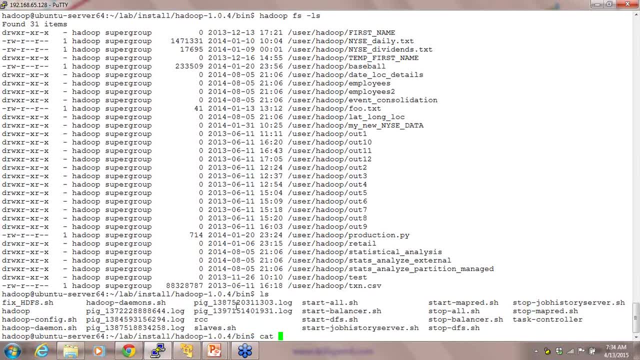 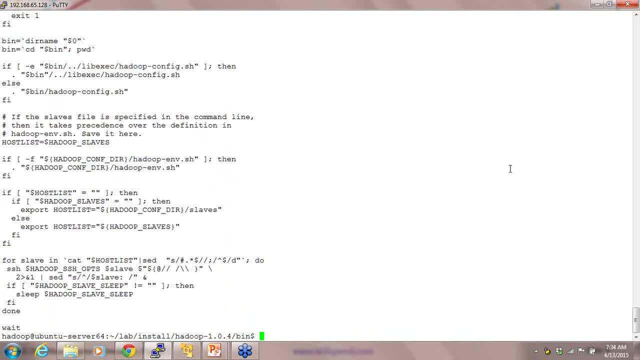 Okay, That's how it is. So this is Hadoop fs-ls. now how do I browse my? how do I see the data inside a file in my local file system or Linux file system? I say cat and then say slavessh. there you go. this is the data. 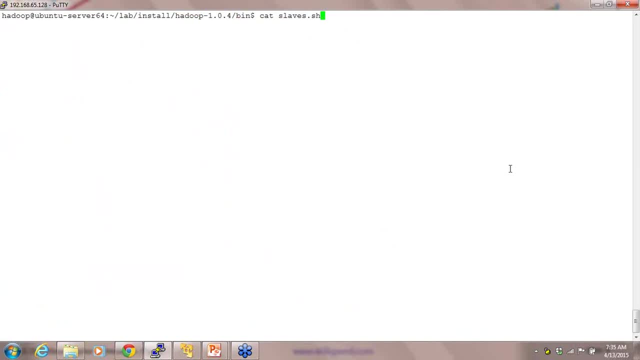 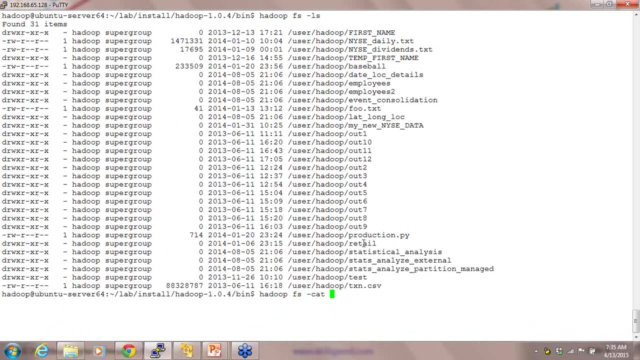 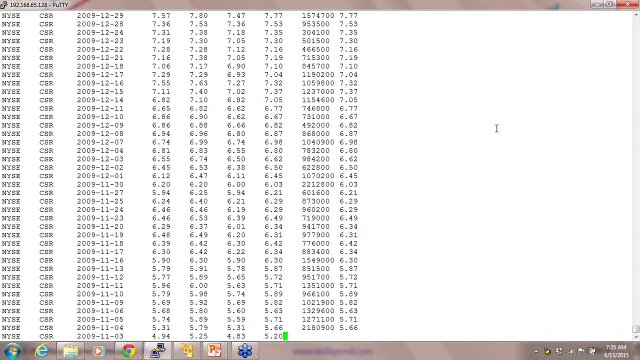 How do I browse? how do I browse my data inside my Hadoop file system? Let me first look into the file and then I say Hadoop, fs-ls And cat of, let's say nfc-daily. there you go. this is the data. 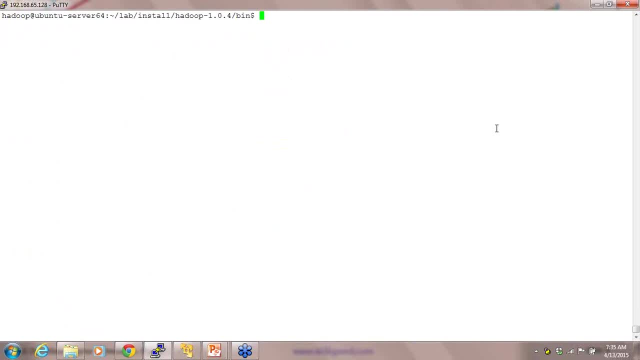 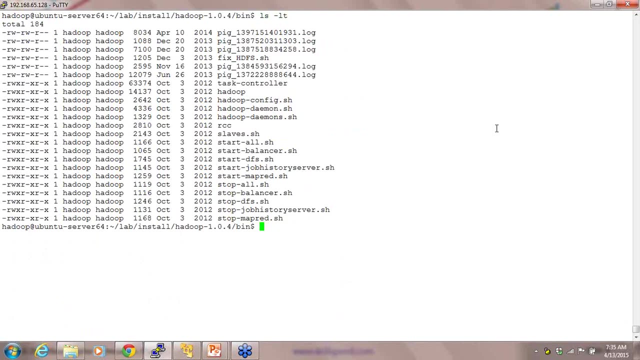 So isn't it quite simple, guys? This is about how do you browse it. Now, going back to my example of why the whole Hadoop file system is extremely scalable and flexible. I gave you an example of server going down. there has to be a downtime in order to upgrade. 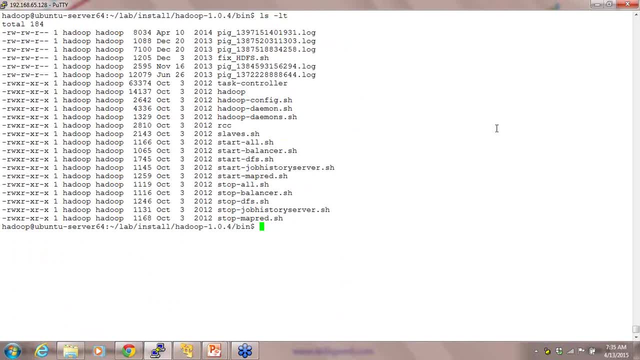 it in order to upgrade its performance. Okay, It's actually software in order to upgrade its memory, in order to upgrade its hardware, Right? So how do I upgrade a system from three node server to a hundred node server? This side: 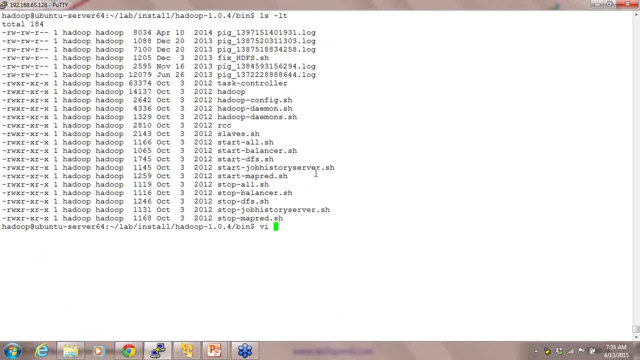 How do I do it? I say vi and then I say slaves. okay, this is I'm inside Hadoop. okay, let's let me go inside my conf c-o-n-f. this is configuration folder. inside that I say: there is something. 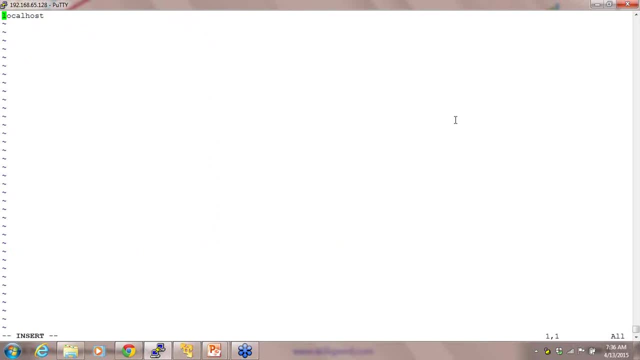 called a slave. Let's say, for example, I want to add- I see you guys have a lot of questions, but I'll take in some time- I want to add, let's say, a few more systems: 192.168.1.1,, 192.168.2.1,, 192.168.2.2.. 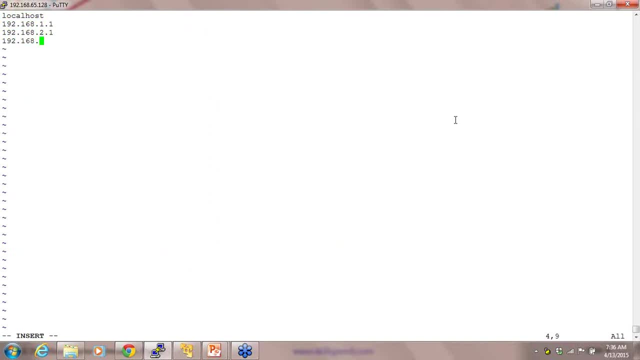 Let's say, these are the three machines that I want to add. That's all. You just open this file, you edit this file, you add the IP address of this machine or the computer names of those machines, and that's done. This system has been upgraded. 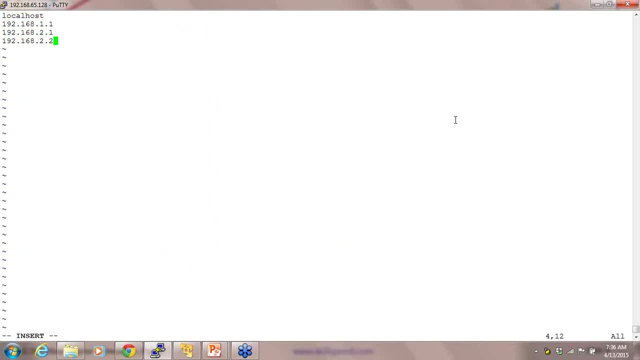 Okay, Thank you. It's that simple, guys. Okay, It's this simple Hadoop. It's just that Hadoop. people think Hadoop to be very complex and, you know, very complicated in nature, programming in Hadoop exercise. very complicated in nature, but it is actually. 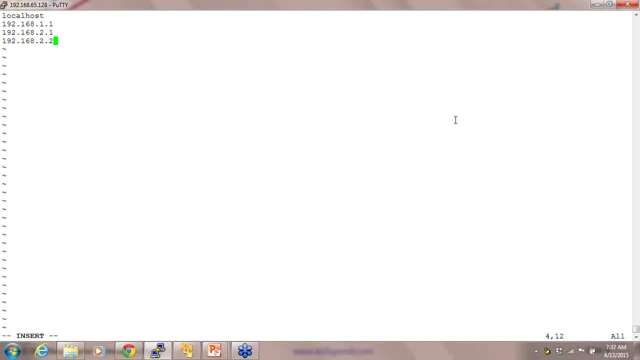 bringing you down one level down. You write a lot of functions in order to do some kind of programming, right? Let's say, for example, you want to take a sum of all the numbers, So how is it that you write? 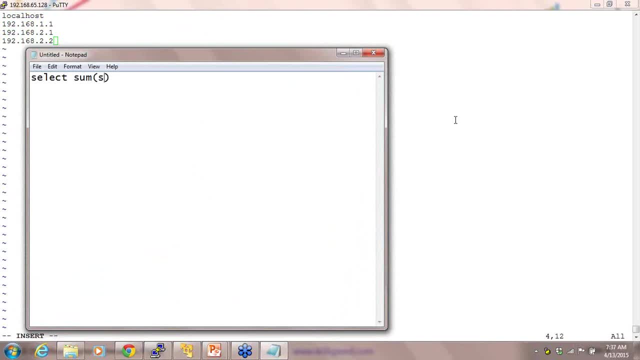 You say in your oracle or wherever it is. you say: select sum of all the numbers. So you have to take a sum of all the numbers in order to do that. Now, what you have to do is you have to break this down and you have to give it a very simple. 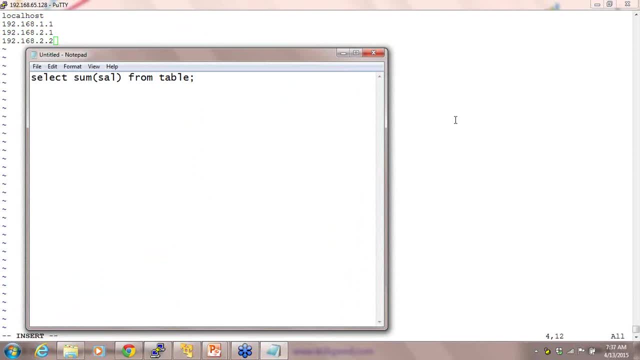 summary of salary from table. This is what you do, right, But with Hadoop, what you have to do is you have to break it down and you have to sum it yourself. Okay, You have to take each salary. Salary one is, let's say, 10,, 20,, 30, you have to take all this data and you have to. 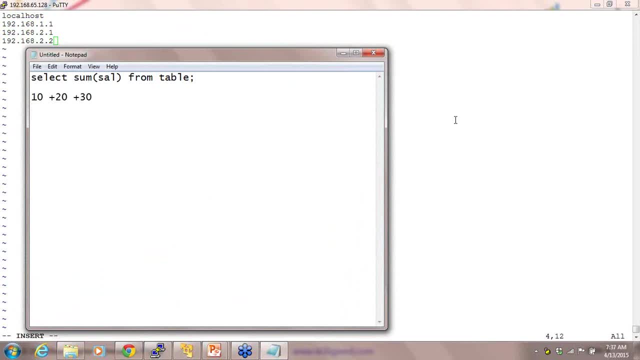 do this thing: 10 plus 20 plus 30. Something of this sort. Okay, It brings you down from functional usage to basic usage And if you know a little bit of functional programming, of functional programming, it becomes much more easier. even if you don't know, it's okay. 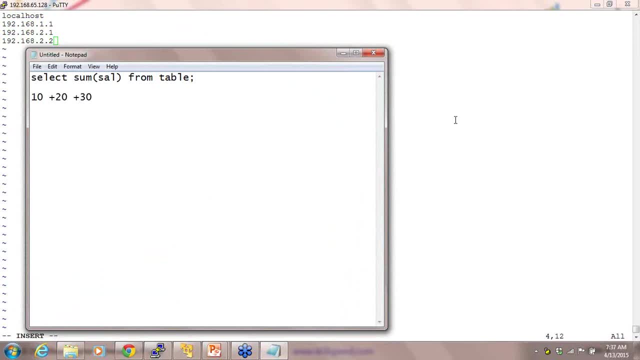 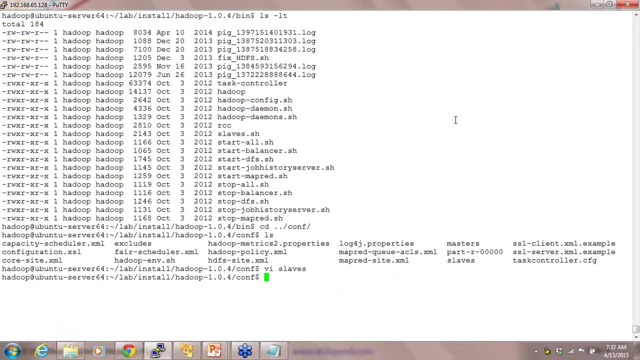 with little bit of unlearning that you have done, little bit of unlearning of the things that you have learned over so many years, you know you'll be able to program easily in Hadoop. Okay, let me go back to wherever I was explaining. 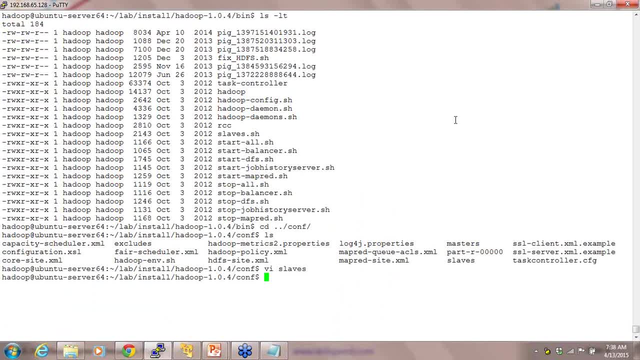 Now that I'm inside my Hadoop, my Hive runs on top of that. okay, Hive will run on top of Hadoop. Hadoop goes straight away into Hive. now I'm running Hive, okay, The first thing that I would show as to how do I use my commands which I've used in Linux: 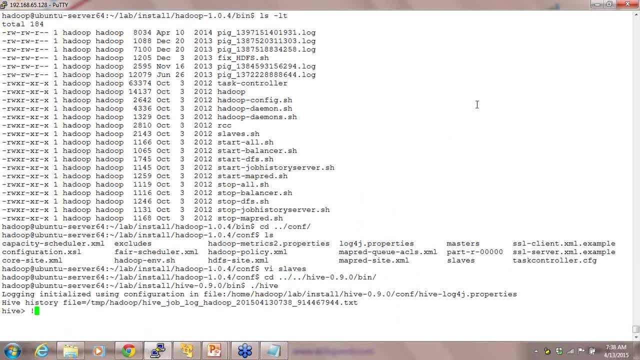 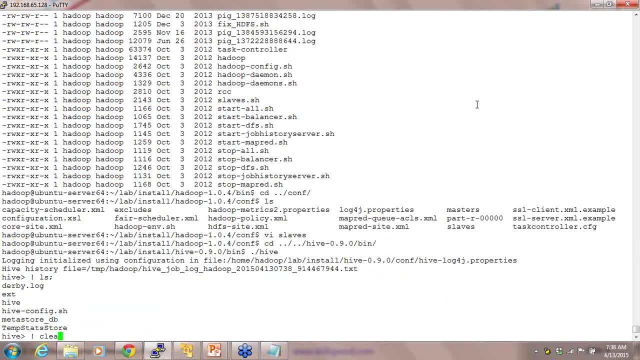 and which I've used in Hadoop from inside my Hive shell. so the only thing that you have to do is put an exclamation mark and then say: list- there you go. it's also listing me, exclamation mark. and then you say: clear, there you go. everything is clear, right. 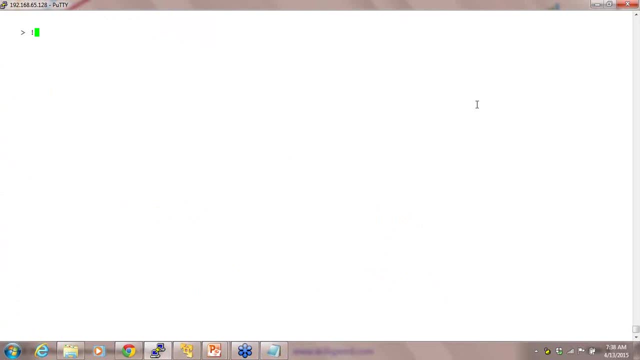 That's the first step. okay, With exclamation mark, you can use the command that you were using in Linux file system or in your Hadoop file system. Now let me look into your question. okay, VAMSI, a VI command. you just write your. 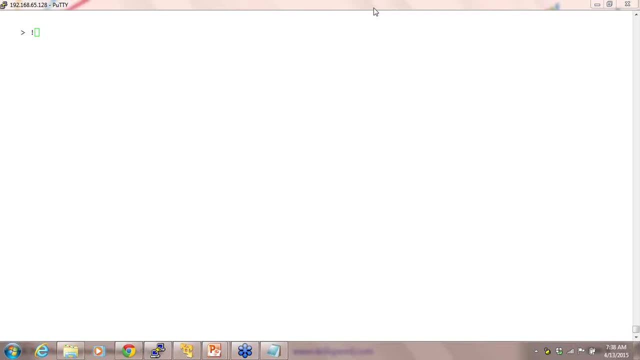 you can write your code in your Linux environment and then, using VI editor, you can edit your code. okay. One quick question says: is Hadoop compatible with latest Windows OS or is this restricted to Windows? With Hadoop 2.2, it's compatible with Windows as well, but whenever we are working in an 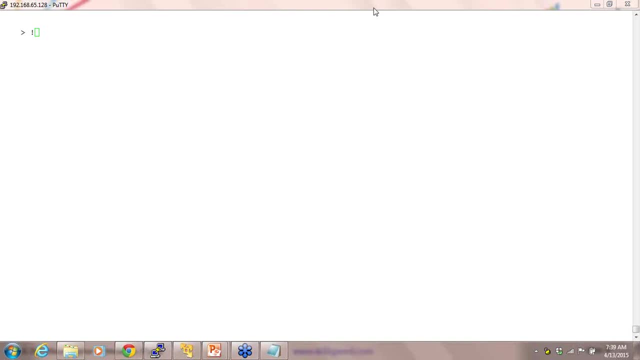 organization. right, we like the security that Linux provides rather than Windows, so we normally tend to use Linux. Where are these? okay, where are these nodes present? Rohini, if I understand your question, these nodes can be present anywhere. okay, let's say, if you are sitting in Bangalore. 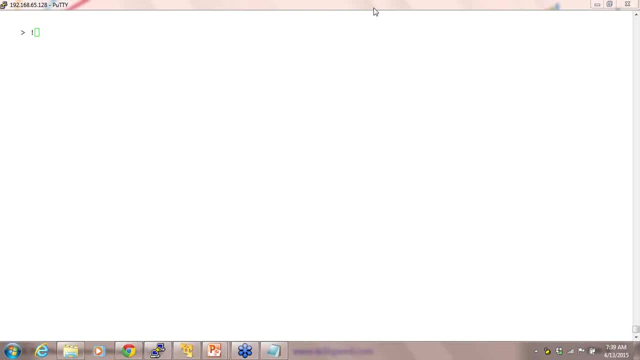 and you have nodes in New York, you can still do that. okay, but then the bad part about Hadoop is you might have to establish a tunnel from Bangalore to New York or you'll have to have a static IP or a computer name which this server can get. you know, you have no. 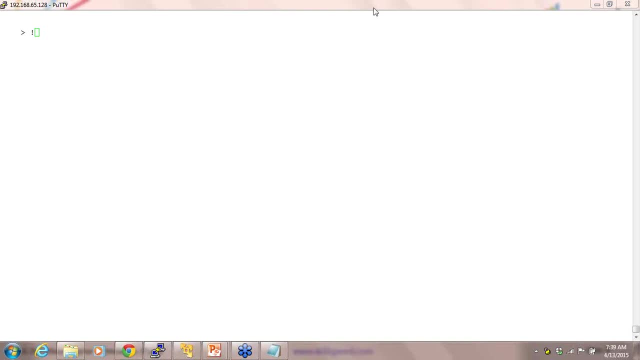 restrictions on where you can place your cluster in case of Hadoop. Is NetEase a front end of Hive? No, NetEase is a massively parallel processing system- Sudhir, okay. whereas big data in NetEase, the parallel processing, okay. guys. if you did not know what NetEase is, NetEase. 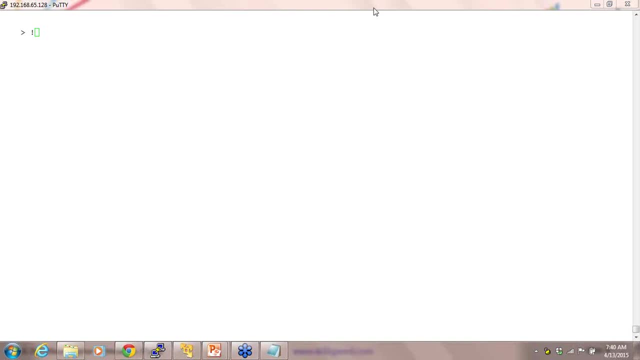 is a parallel processing system. It's a system from IBM- okay, it comes quite costly. and the parallelism in NetEase is because of its hardware and not because of the software- Sudhir, okay. so in case of Hadoop, the parallelism. 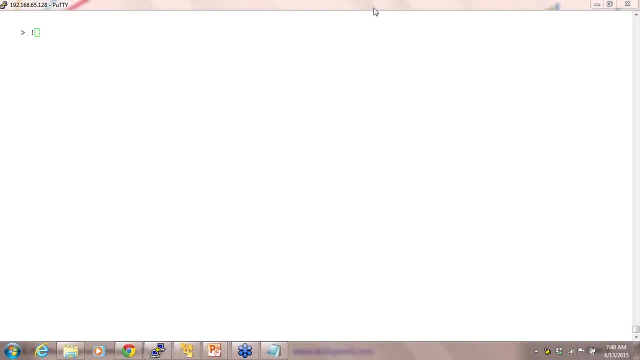 is because of software, but in NetEase it's because of the hardware. These are two different architectures. okay, we might be comparing apple and oranges. Okay, is it possible to export using Hadoop? Yes, it is possible to export using Hadoop. I'm going to show it to you in some time. 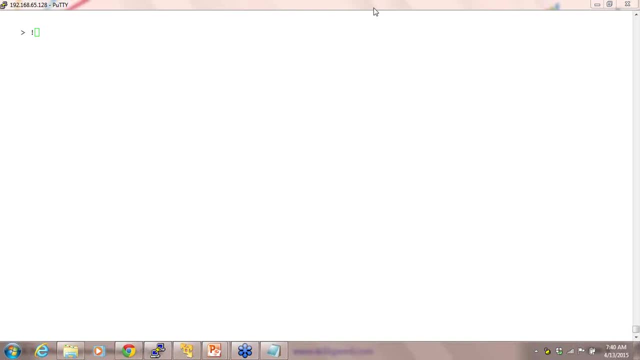 Melvin. Okay, is there no handshake necessary between the two systems? You will have to have a handshake, but you have network for handshake, right, Akshata? Does all the other nodes have Linux and have Hadoop installed in them. You don't even need to do that, okay. so that's the beauty of it. 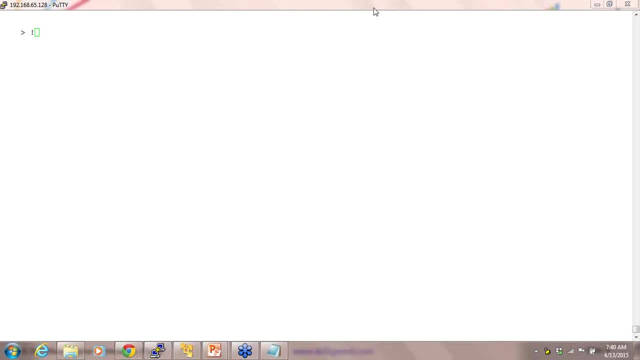 You need to install a couple of daemons called as data node. there is one daemon called as data node, but not the entire Hadoop system, okay. so let's see this. now let's go on straight away into Hive, okay. 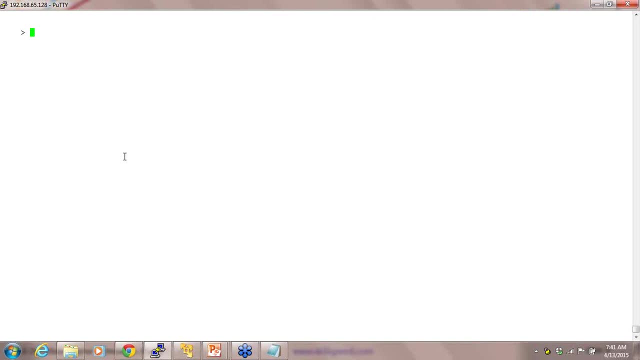 Now I'm inside my Hive cell. now. first thing I told you at the start is Hive is a query language. Now how does Hive look like? Let's say I start with, let's say I do a show databases. My system will be a little slow, guys. we'll be with that because it's my local machine. 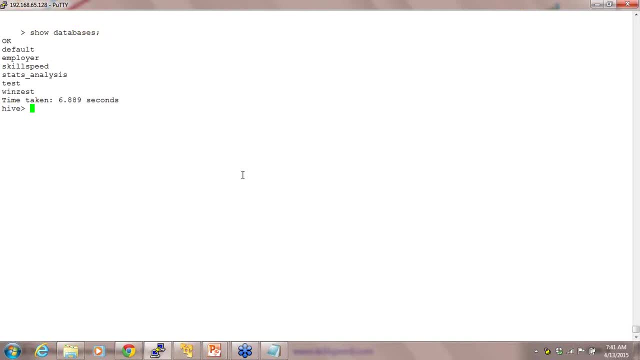 I have a VM on top of it. I have tons of applications running on it and that's why you know I have. Now, if I say show databases, I get this all. I get all this information right right Now. these are all databases. if I want to create a database, how do I do it? 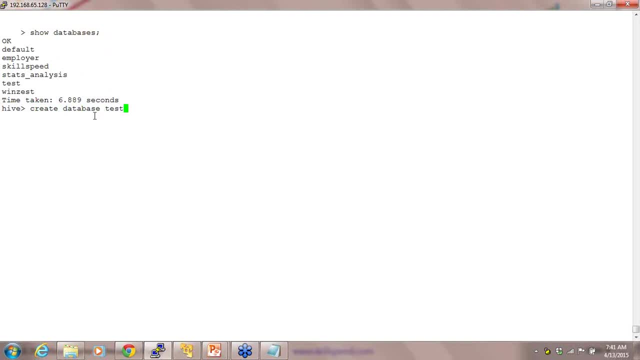 I say: create database, create database. and then I say: test right or test one, There you go. it created database. now I say: show databases, there you go. there is one database for test one as well. Now I use an already existing database which is, let's say, employer. 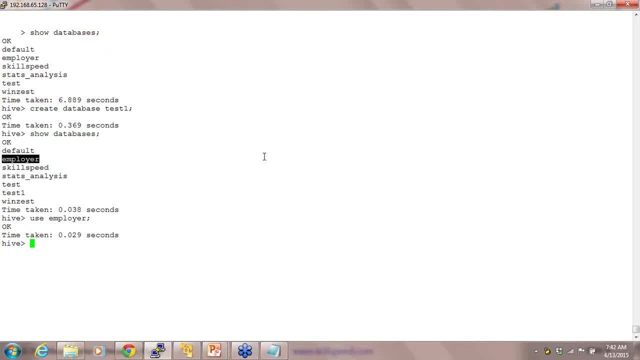 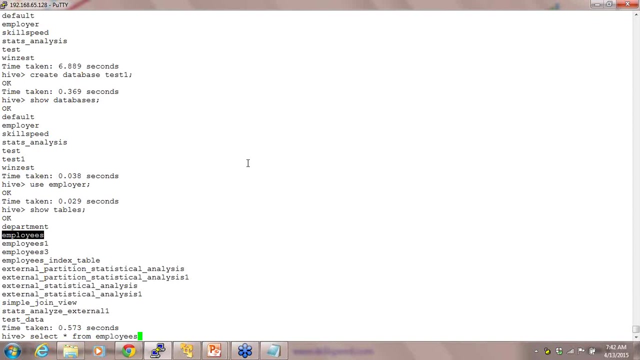 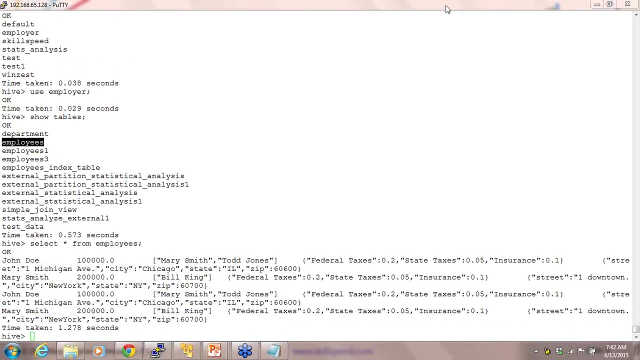 Okay, Okay, Okay, Okay, Okay. And now I say: show tables inside my this database. Now you see, these are all the tables inside my database. Now I say select, start from employees. there you go. Now this looks a little different, right? this looks exactly like SQL. 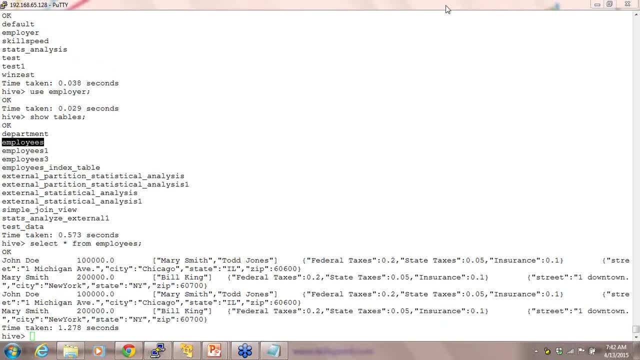 Yes, see why it's exactly like my SQL, but that's a little misleading, okay. Okay, might look just like MySQL, but when it works internally, Hive is a query language. Sushmita. Now, Hive is a query language which sits on top of Hadoop. 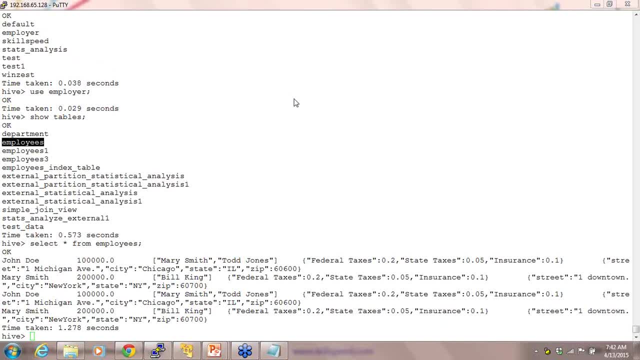 It processes big data. It does not process small data. It is useful processing big amount of data, But data output is JSON, Not necessarily Siva. data output can be JSON. data input or output can be JSON text, your structured database, your XML, it can be anything. 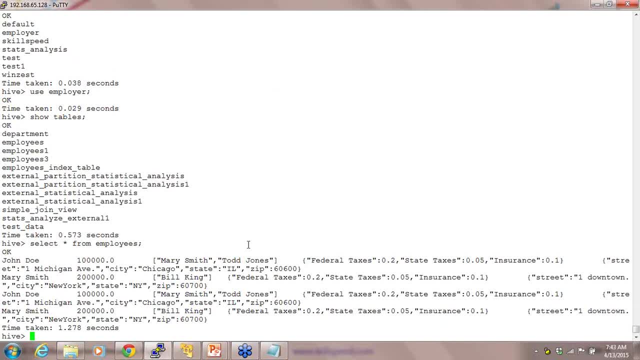 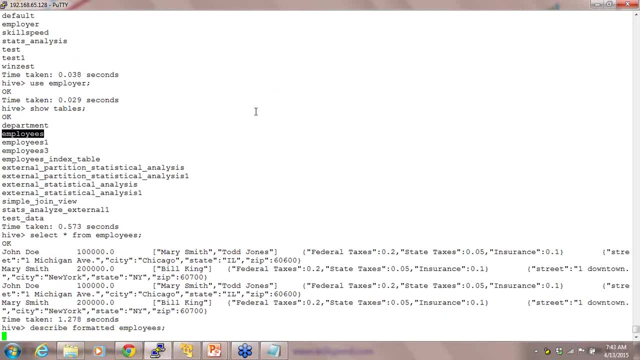 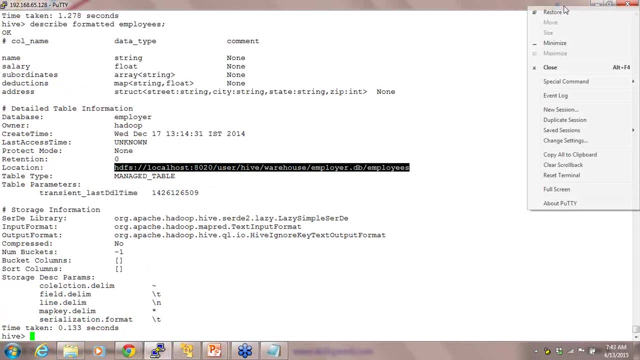 Okay, Siva. So here you see. Now let me dispel some of the myths. Describe formatted of employees. You would have seen this as well. Now let's see this. What is this? It says this is a location, okay. 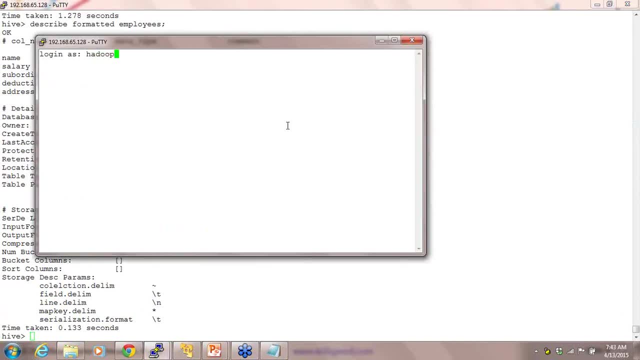 Now let me open one more window for you guys: Duplicate session and my Hadoop as a user name. Okay, It's still. okay, it's still connecting. Oh, it's taking a lot of time. Okay, Hadoop one, two, three. 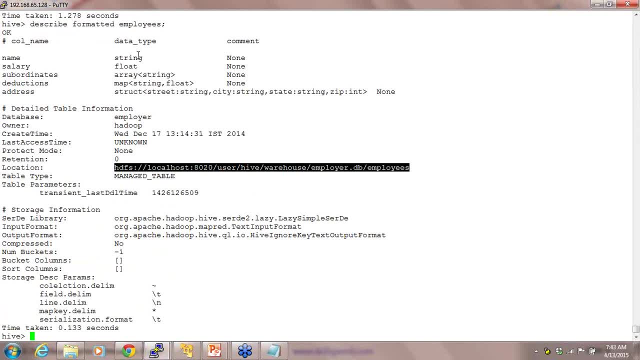 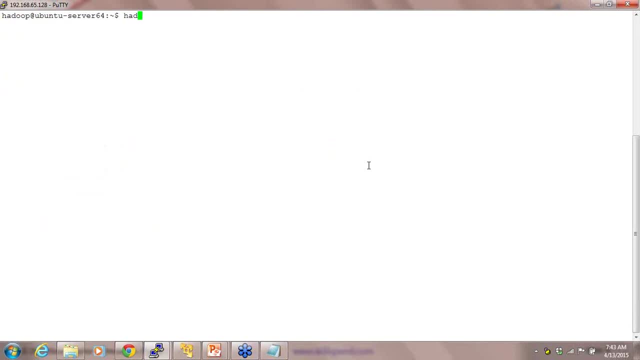 There you go. I clear the system. Now, what is this? It says that this table is pulling the data from this location. Now let me go and check from this location as to what it has. I say: Hadoop FS minus LS. 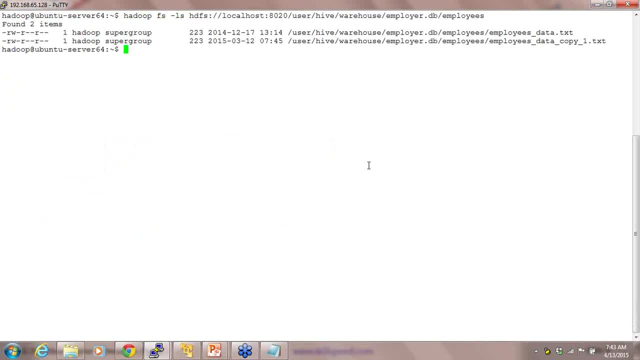 Does this location actually exist? Yes, it does exist, And you see that there are two different data, two different files here. Let me check Now. let me go here and say CAT, You see this, guys, It is the same data from this file. 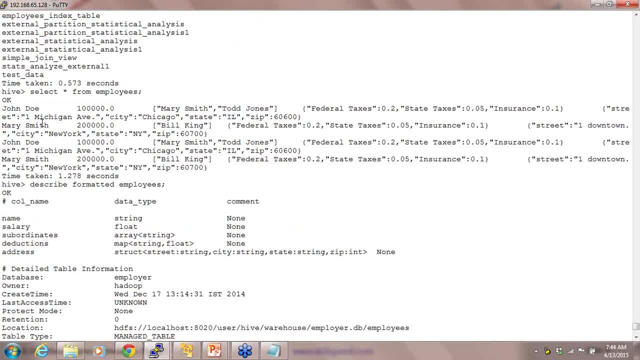 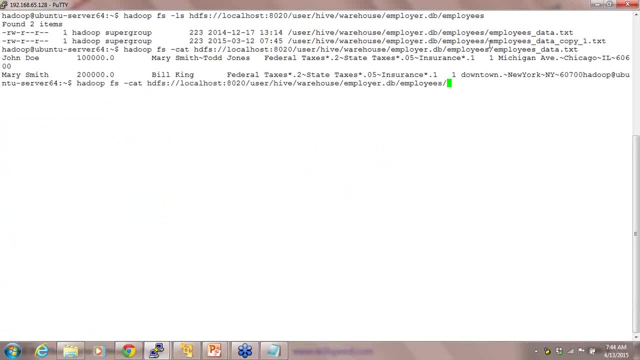 which is being pulled out and it's displayed here. You see, John Doe, Mary Smith. John Doe, Mary Smith. That's from the first file, From my second file, From my second file. there you go right. So basically, John Doe has been repeated twice. 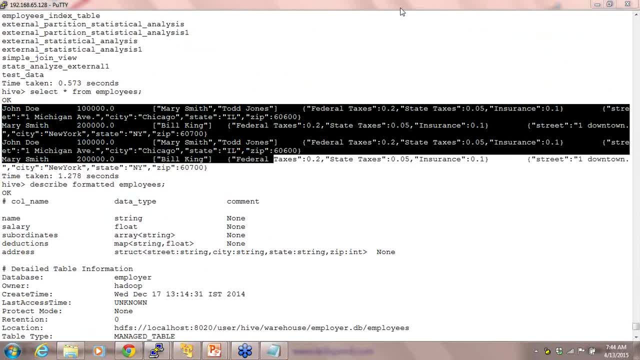 That's what I get when I do select star from table. So what does this mean, guys? It means that the data is being fetched directly from the file. It is not stored in any structured data. So externally you might feel that this is like MySQL or SQL, but internally it is different. The data 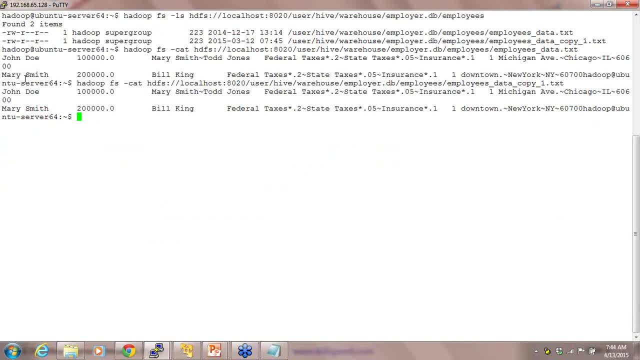 that is being dumped here when you say select star from table, is nothing but the location and it goes to this particular location and pulls out the data from employees table. The second thing here, very important thing: I said select star from employees. Now the name. 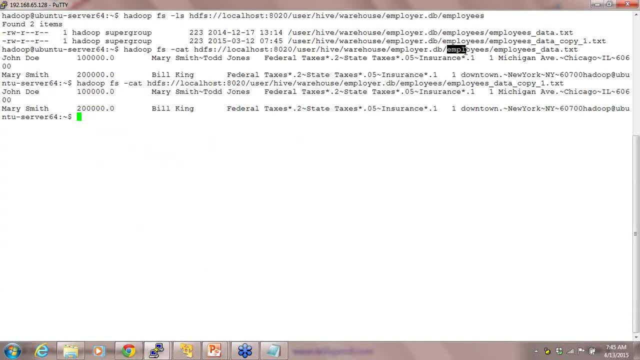 of employees is a table here, right? If you go here, the employees is a directory here. You see that. So whatever tables that you are creating in the backend inside HDFS, it is creating a directory And whatever data you are inserting into this table is getting. 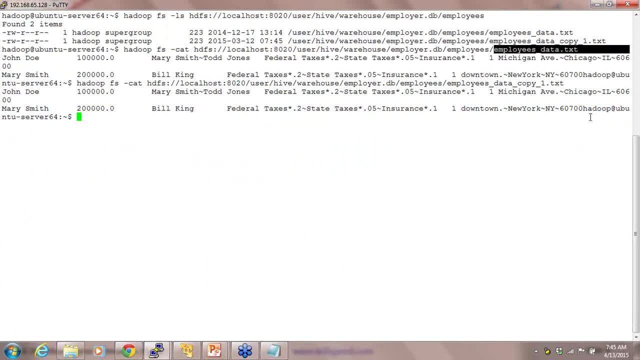 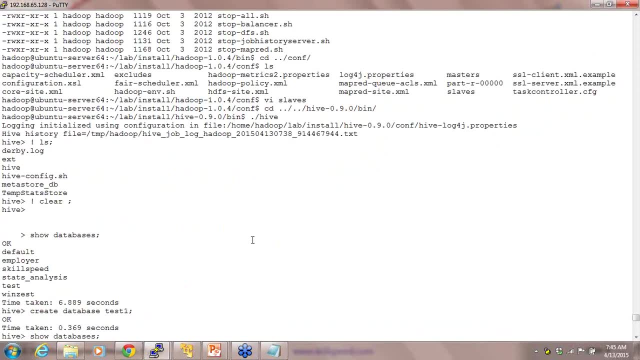 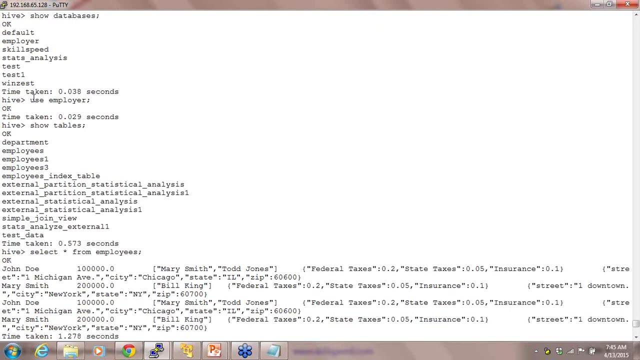 created as a directory, As a text file or a JSON file or whatever XML file, whatever you want to show the data as. And initially I also did one thing right. I said select star from employees. I said use employer. right, This is what I said. So what is employer here? Employerdb, That's. 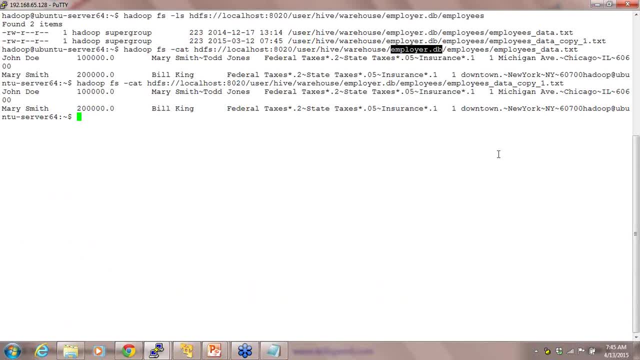 the database. So database is a directory. Your table name is a directory. Your data inside the table is a directory. Your database is a directory. Your data inside the table is a directory. Your table name is a file. Guys, is this clear? It can be used in clustering. 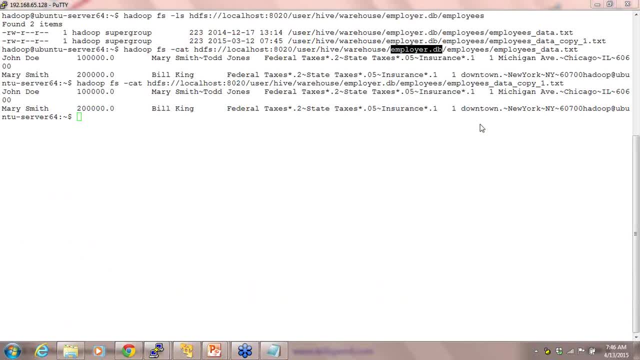 purpose or data transfer error It can be. it can be used to store data. It can be used to process data. It can be used for anything that you can think of. Okay, See what? So no relations needs to be defined in HDFS. No, The data that you store eventually is: 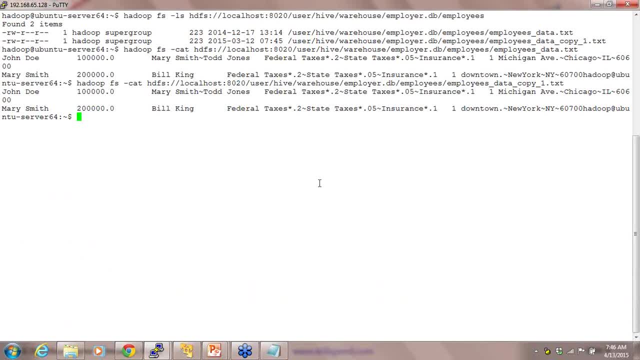 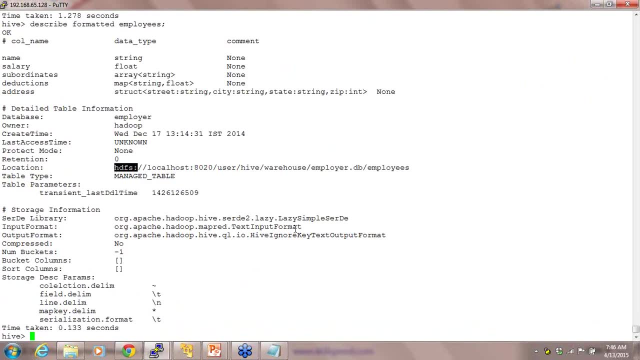 written inside HDFS. You see this, Where is the data stored? I say Hadoop, FS, LS. or if you go here when I say disk formatted, where is the data stored? guys, It's stored inside HDFS. So this is the relation In this. 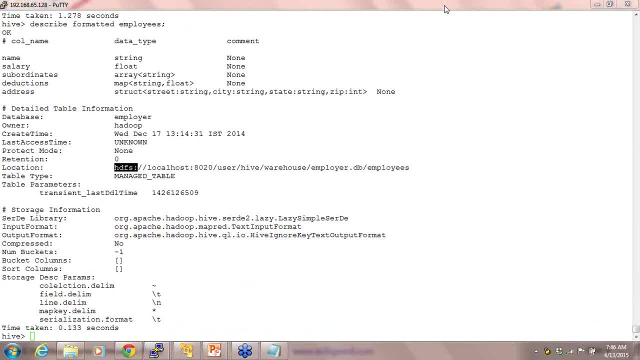 file should data be in certain format. The data can be in any format. It has to be: either it has to be in a normal format, a tab-separated format, comma-separated format, JSON format, XML format. You have a variety of options. Your data can be. 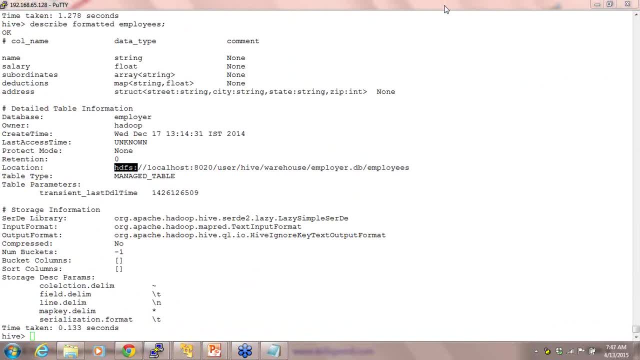 It can be in any format and you'll be able to read the data as you would normally read a table. You can. yes, Vishal, you can create a gzip file using Hive as well. Okay, You can create a gzip file. You can access, You can read, But reading is really difficult for. 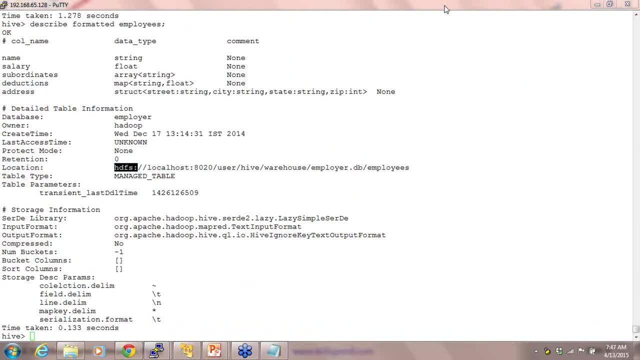 some of this Bzip2,. instead of gzip, we use the compressor format as Bzip2 in order to compress this data so that Hadoop can read it. There are some complications with that. There are some complications there which I will not cover it today. Okay, But then yes. 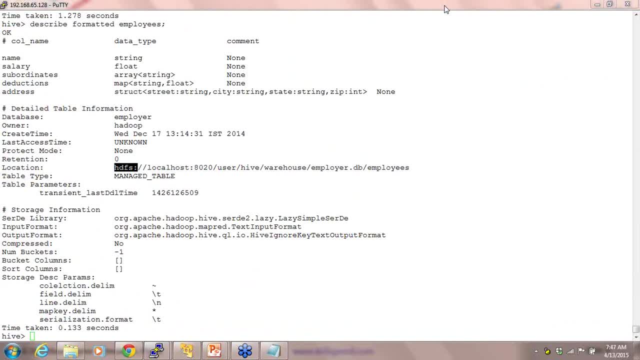 some kind of compression can be used with Hadoop as well. Absolutely, Rohini. Okay, Rohini is saying: if you say select star from employees where name equal to XYZ, then it has to check all files right. Absolutely, But there are concept. 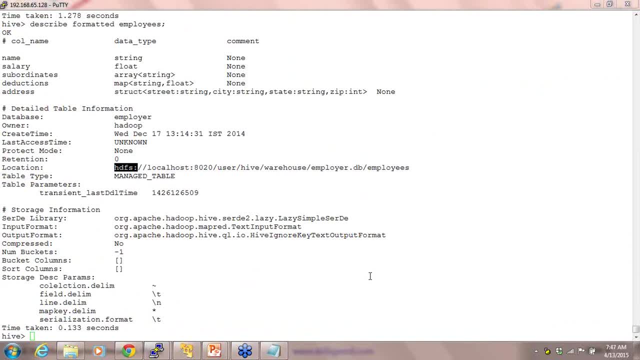 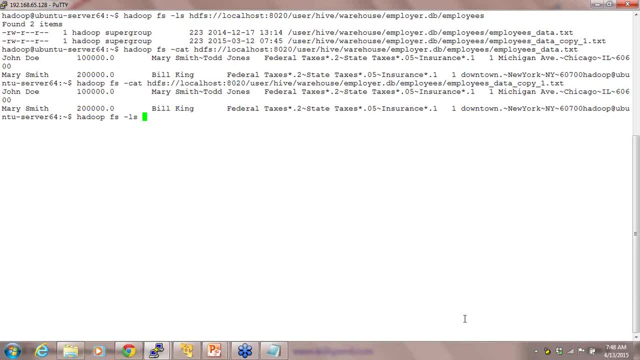 of partitions there, Whenever you do, and it's never an overhead, because this data that you see, this data that you see, will reside in different nodes. Each of this data will reside in different nodes. And when you say, select star from table, where column name equal. 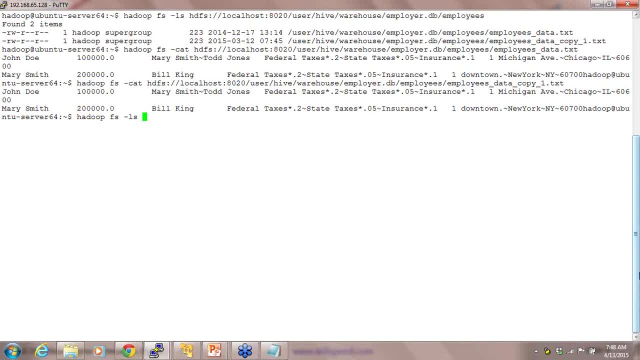 to some value. it is going to spawn a thread to, let's say, 100 different nodes And this data residing in 100 different nodes, it will start searching at once in all these 100 different nodes. So your chances of retrieving the data with 100 different machines is faster than 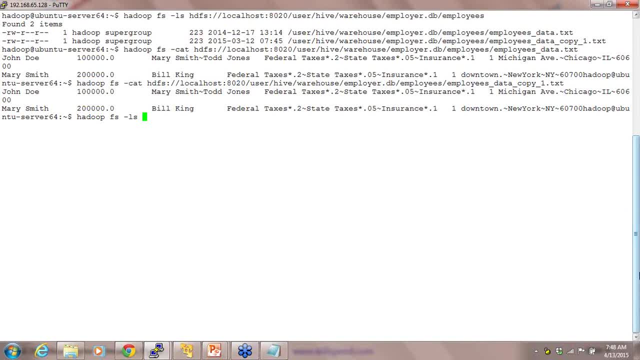 one machine. Okay, Rohini. Now I have lots of questions coming in from Vivek Abhishek, Vishal, Edwin. How long does it take to become a Hadoop developer? It does not take long, I would say, Edwin. if you know any programming language, for that matter. let's say you know one programming language, be it Java, Python or any programming language. If you know, it will take you around a month or month and a half time in order to become a developer. I'm not saying a good 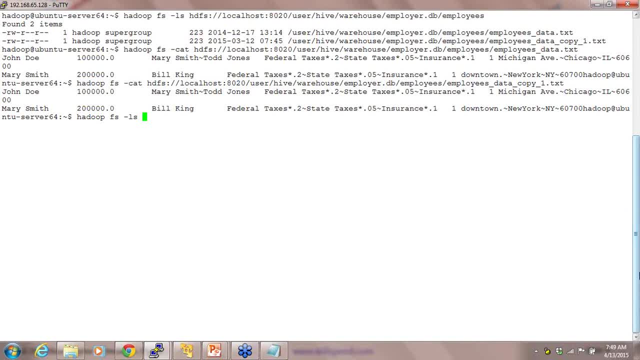 developer. I'm saying a developer. Okay, Can we have mixed data format? Yes, Anzal, you can have mixed data format as well. Yes, Anzal, sequence files. So we can have sequence files as well. How about processing unstructured? 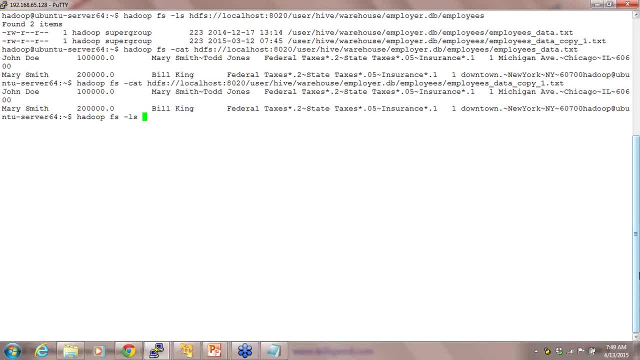 data. So this is unstructured data, right, Kumar? I mean you can call this a semi-structured, a JSON file, your XML file. these are semi-structured, But if you have completely unstructured data, let's say, for example, like a text file, you have to convert that into certain format. 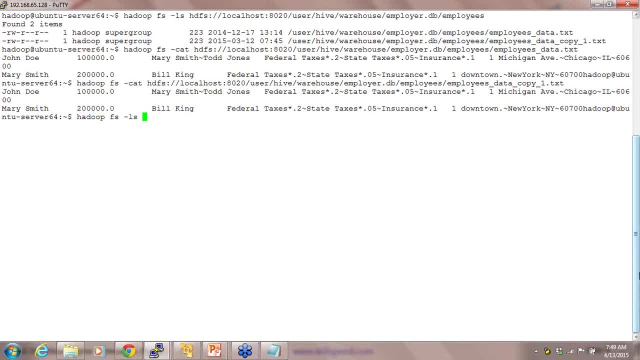 and then make sure that you process it with data. Okay, In order to process completely unstructured file, we use PIG. So we're not talking about PIG today. That's why I'm not taking you through the details of PIG. But if you have a completely 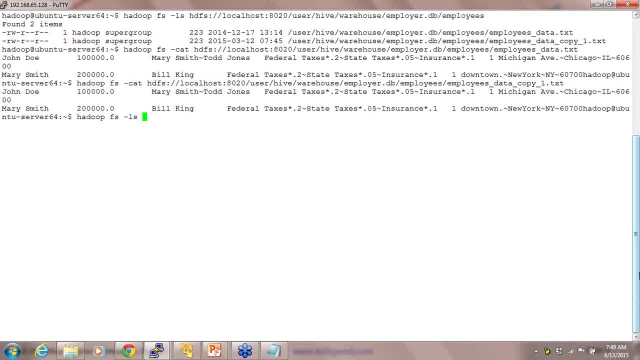 unstructured file. I use PIG, And then, once it gets certain structure to it, or certain semblance of structure to it, I go ahead and create Hive on top of it. Okay, You're not able to imagine nodes, right? I can understand that. Okay, So the way it works is: let's. 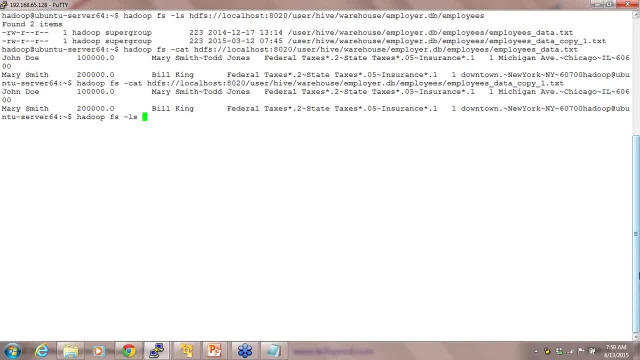 say: my machine and my machine can be part of a cluster and your machine can be one node, my machine can be one node. Okay, So I'm talking about a computer system is called as a node as well, Basically a commodity hardware, a hardware which costs very cheap, Are this? 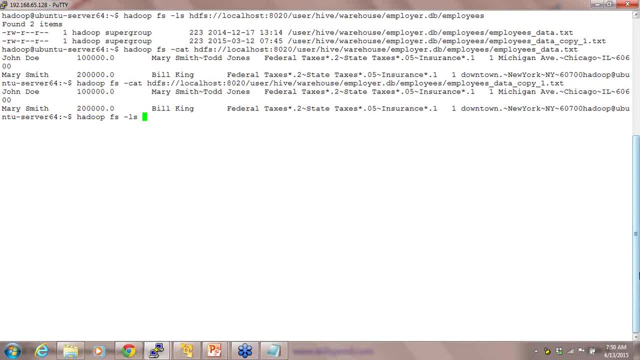 file indexed? No, these files are not indexed, etc. But you can create an index on top of this file as well, But that's of no use In case of big data environment. right, everything is called okay from one parent. 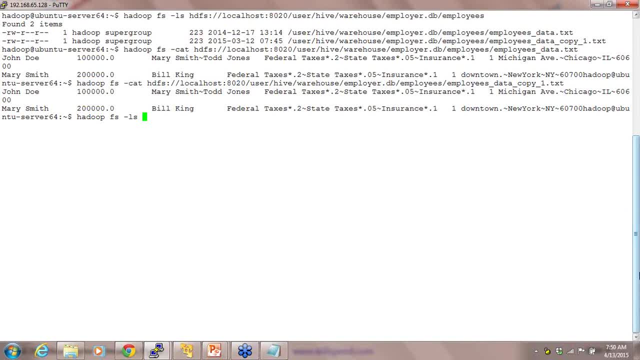 You know, hundreds of child will be spawned. From those child, further child will be spawned. And then if you- it's like if you're trying to search for X in a pile of data, let's say, if you're trying to search for a country in one GB of data, So first of all that one. 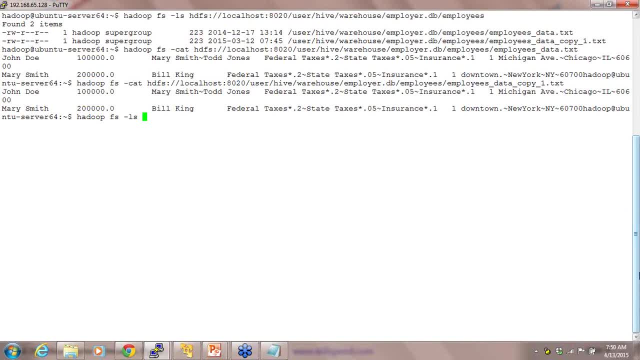 GB of data will be split into 64 MB chunks. Okay, So, for example, 20 chunks, right, 20 chunks will be passed on to 20 different machines. Once the data is there in 20 different machines, you have your search algorithm which will search for a country in all these 20 different. 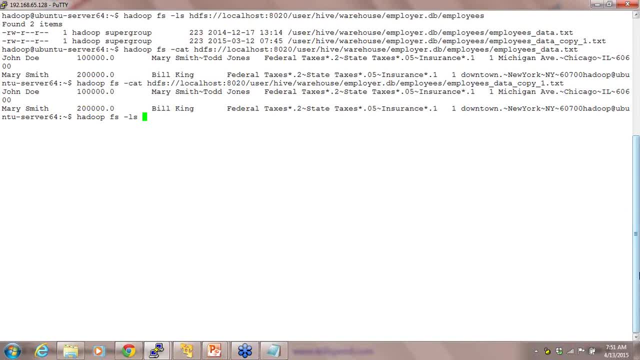 systems. So that's why it's easy. I'm sure you'll find it a little difficult to imagine, but just go ahead, do some kind of little bit of research and then come back to Hive. Okay, You'll find it very interesting and very easy. No problem, Rohini. 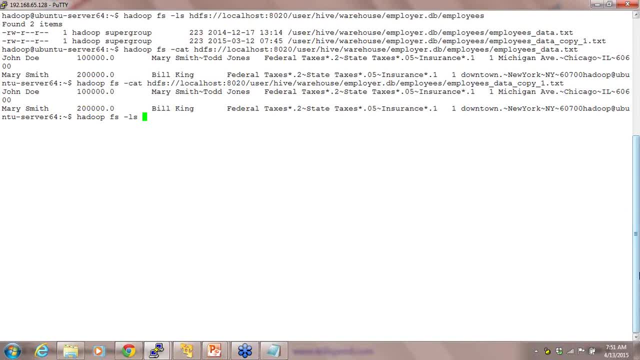 Whatever, replication of data across nodes. yes, there is something called as replication factor, Praveen. It is each data, each 64 MB of data, is replicated across multiple nodes so that you can have a search algorithm which will search for a country in all these 20 different. 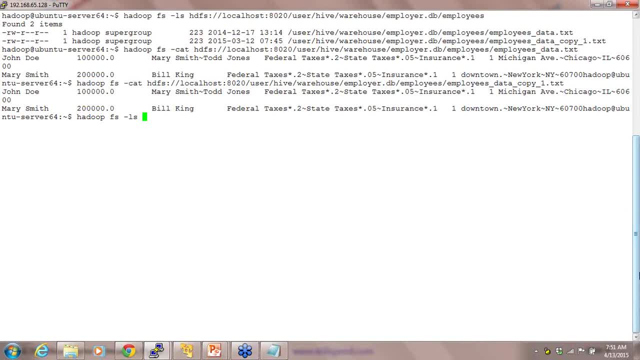 systems. So in case of eventuality, in case of failure, you still do not lose out on the data. Okay, So by default, there is again: if you go to HDFS sitexml, there is a file called HDFS sitexml. There is something called as replication factor. You just have to mention. 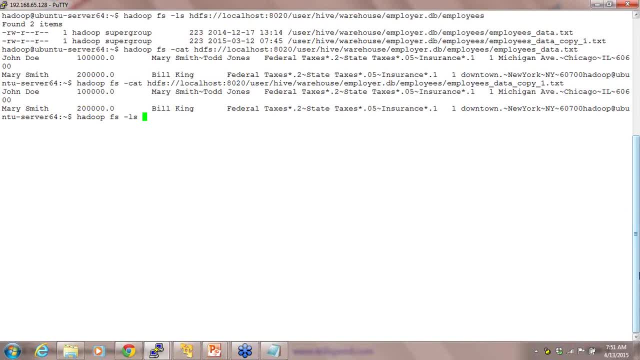 it's all configuration parameter right. You just have to mention one, two, three, whatever you want to. By default, it comes to three, And if you have replication factor set to three, the data will just be replicated in three different machines. 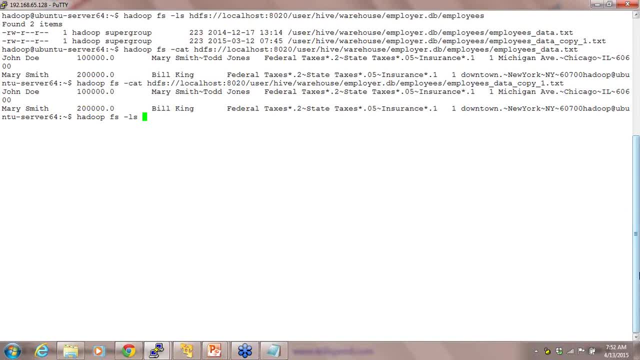 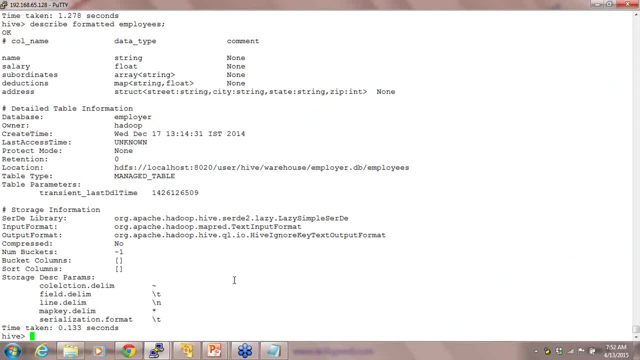 Okay, Anshul, let me explain this to you. Anshul, Vishal Kumar Nihalika, let me first explain to you as to what schema on read is. So schema on read is whenever I do an insert. 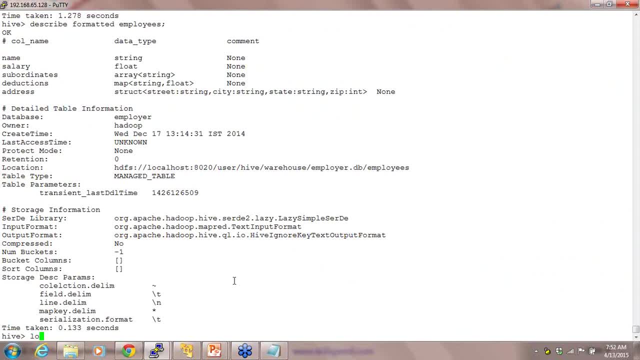 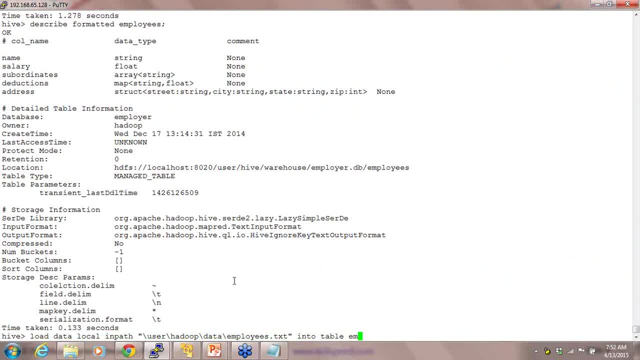 into table employees. now, I don't have this data. when I do this, what happens is that it does not validate whether this data, what kind of data it is. let's say, for example, in my employees table I have name, column salary, column subordinate, column deduction. 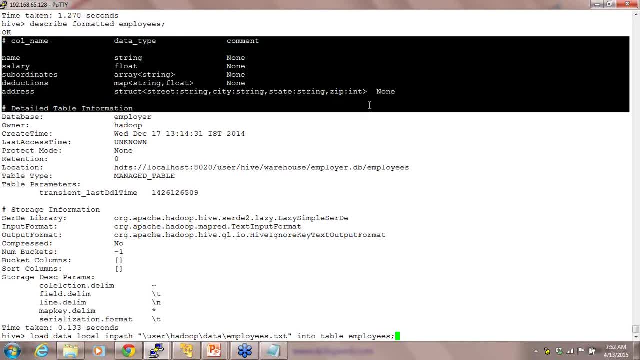 column and address column as well. I have this: five columns. but look at this: the data type of this column: array, map and sector. let's come to that later on, when I look into this table. and then let's say this employee's table, or, by mistake, what you did is you. 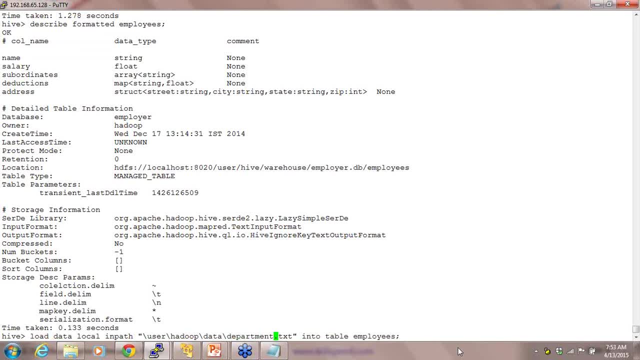 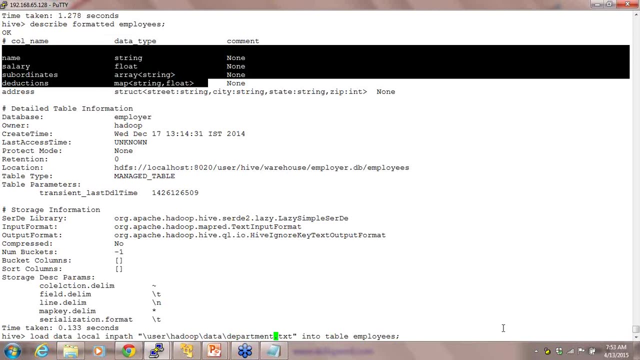 say departmenttxt, let's say by mistake, you are inserting departmenttxt into employees. it will still go ahead and insert the data, because it will not validate for each of this column with this data. it will still go ahead and insert it and eventually, when you are. 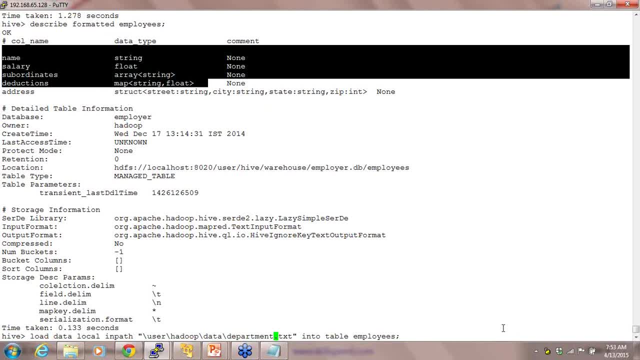 fetching the data from hive. you might not get it in a proper structure. eventually you might get it in a proper structure. you might get it in a proper structure and then you might get it in a proper structure. get all this data as one column itself. so that's called a schema on read. it's not validating. 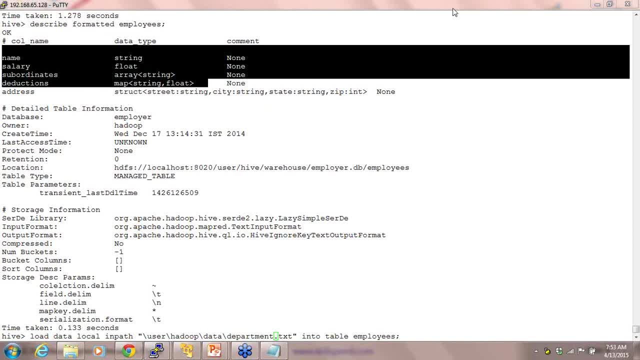 the data when you are inserting. it's only validating the data when you are retrieving the data. Okay, Niharika says so. do you always need to maintain a live connection with all your nodes? Yes, Niharika, that's true if it is across a network, if it is in one place, if you have 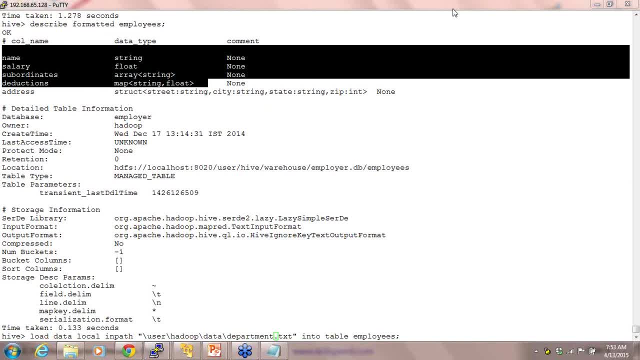 a hundred node cluster in one place, then it's all connected by hardware, right? so you don't have to worry about that. Yes, Niharika, that's true, but it's much easier than the way you are thinking it to. 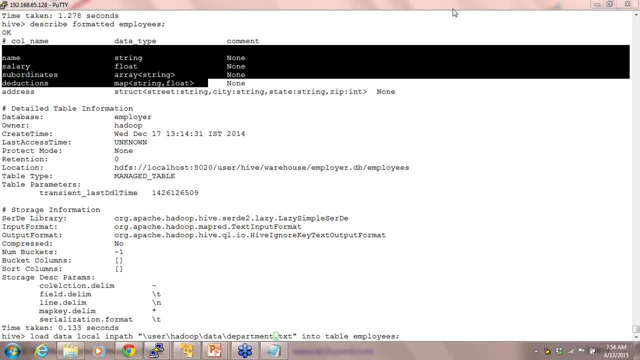 be right. even if it is not able to ping one server, it will eventually ping at least 30% server. yes, you are right. so normally it so happens that I have one cluster here in India, I have one another cluster in China, one in US, and so on and so forth. okay, If nodes? okay, Kumar, if nodes are connected to a network, then it's all connected to a server, right? so you don't have to worry about that. Yes, Niharika, that's true, but it's much easier than the way you are thinking it to be right. 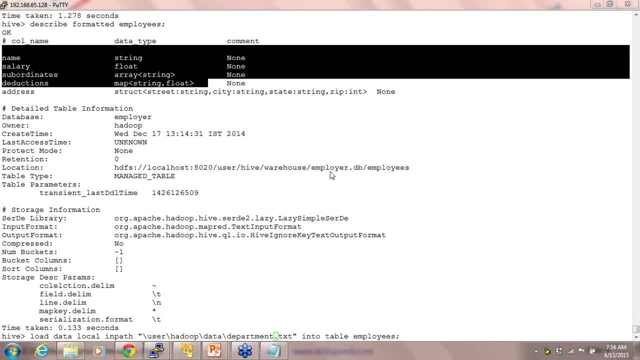 if nodes are across continents, big data transfer might take forever, but then see, the big data transfer that happens over network, across continents, is only as a backup. okay, it is better than you losing all the data. right, let's have one cluster here, one cluster. 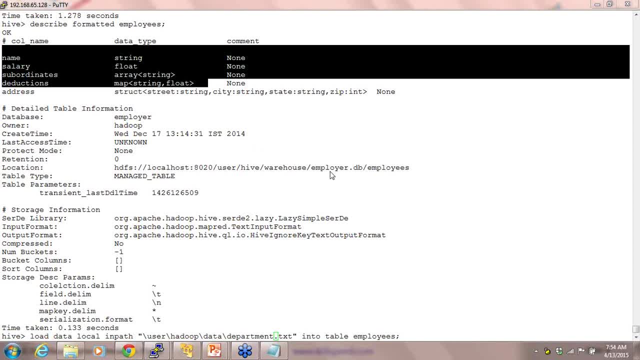 in China and one cluster in US. so the algorithm is so beautiful that, whatever data you upload it over here right, first of all it will search for the nodes which are nearest to my geographical location. Once that it loads the data over there, 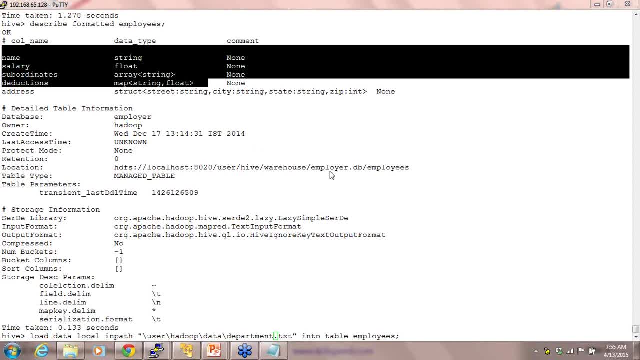 The next step that it does is in order to take any replication which happens in the background, which your program will not. your program will not even be disturbed. It will find someone which is nearest to that geographical location, so it will transfer the data from there to, let's say, from India to China and eventually the last option. 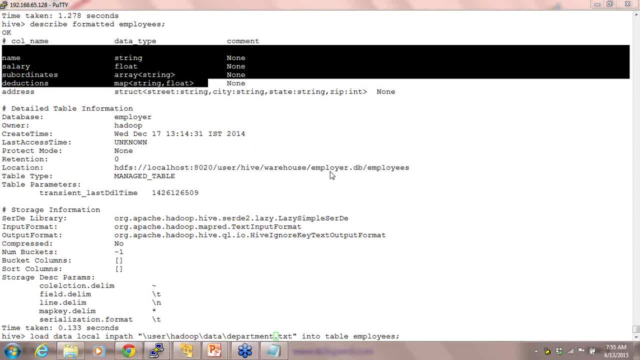 would be to transfer data from China to US. So all this has been thought of. the algorithm is quite powerful and it handles and it does a lot of things. okay, Okay, yes, Sumanth, see Sumanth. okay, Sumanth, it's a very good question. 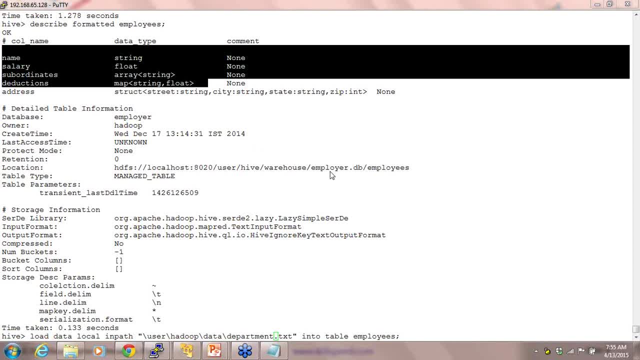 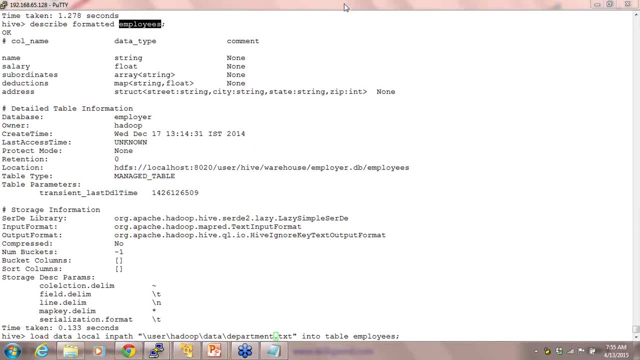 You are saying so. if you insert department data in the employees table, then read the employees table, would the columns of both department and employees be visible? No, you are not inserting the columns Sumanth. okay, So when I do this, right, see here, I have already created a table, so I have a table. 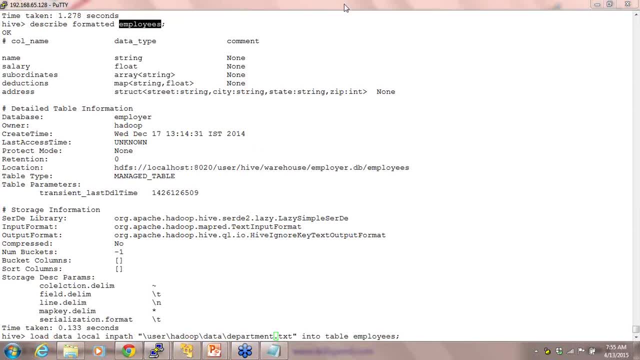 structure for columns. right, I have table structure for employees. I already have a column defined. When I load the data, I just load the data. It does not have any columns there. okay, And now it will be your job. see, this is another way of looking into things, right. 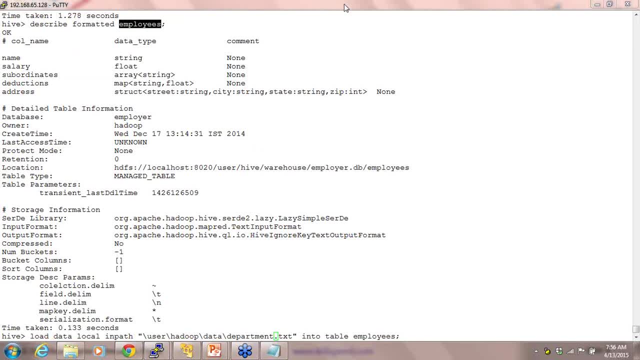 So far, because you are coming from Oracle or RDBMS background, right, that's why you are thinking from table's perspective. But in big data we do not think from that perspective. In big data, we think from data's perspective. 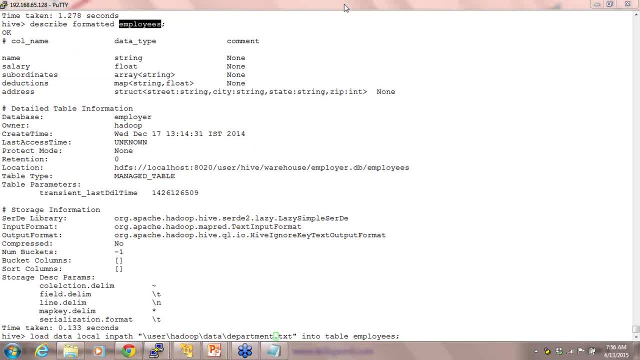 For example, how do you normally work in any environment, in any organization? Okay, How is it that you have designed your table in the past? let's say you work for XYZ company, right? You first think that this might happen, so let me create a table structure. 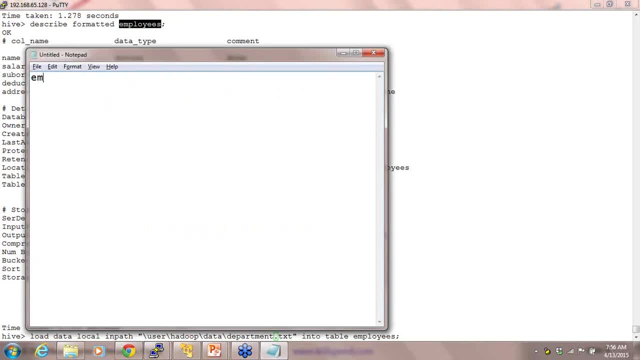 You first think of an employee. This is how you do right. Let's say: I want to create an employee table. You say I need to create an employee's table. In the employee's table I'll have a column called name, salary, age, ID and what else. 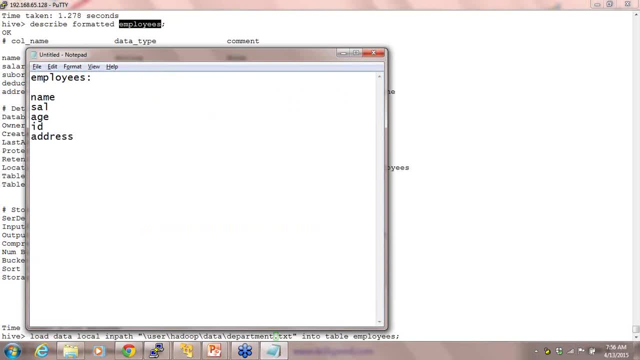 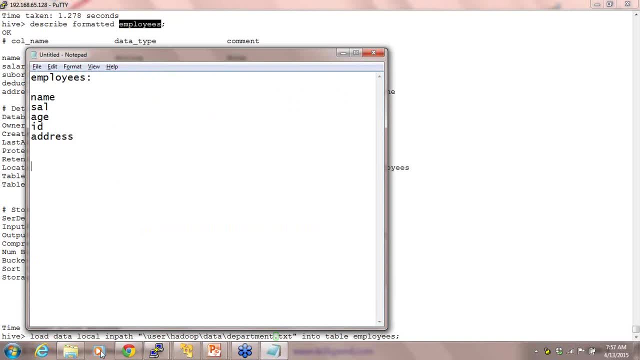 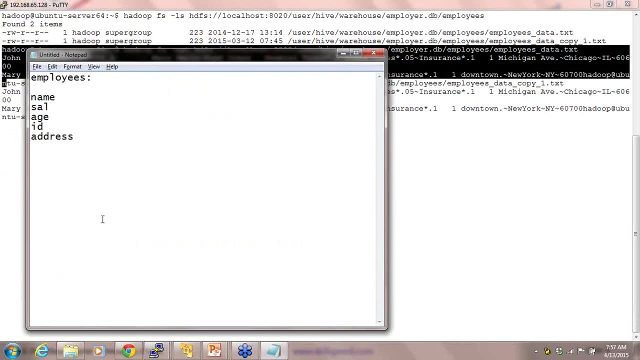 So, but then, when it comes to big data, first of all you go here and then you check what is the data. okay, You check the data here and then you say, okay, this is my data. Now, because this is my data, I need to create a table based on this data so that I can slice. 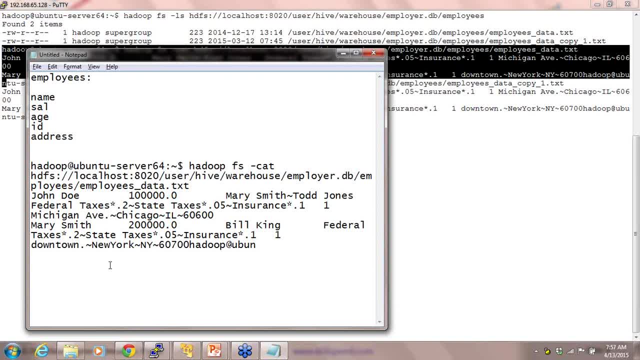 and dice this data right. So there are. it's a different world, It's a different way of looking into these things, okay, So So I understand the point from where you are seeing it. This was the point, you know. this is the vision that I had when I started working on. 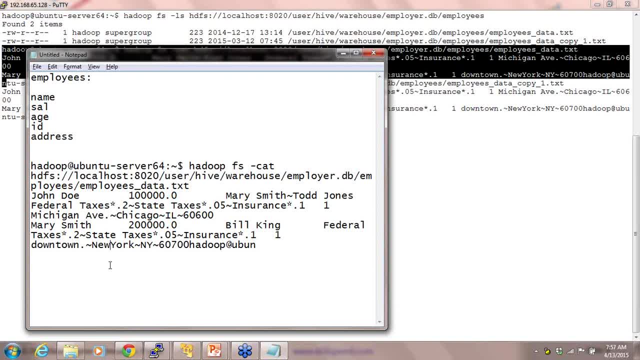 big data. But right now, I know that, when it comes to big data, I'm not just talking about MVs and GBs of data. right, I'm not talking about those data which normal database can handle. I'm not talking about those data. 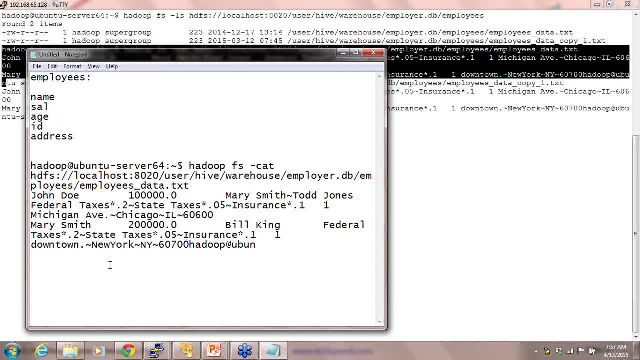 I'm talking about so much of data that normal databases cannot handle or normal environment will not be able to handle that. Okay, Thank you. Yes, When you define the input format, right, Sachin? so first of all, you look into your data and 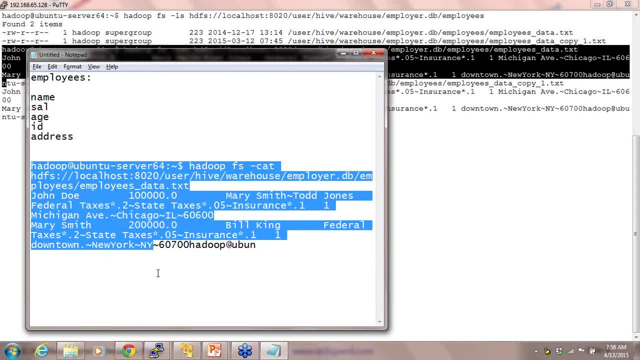 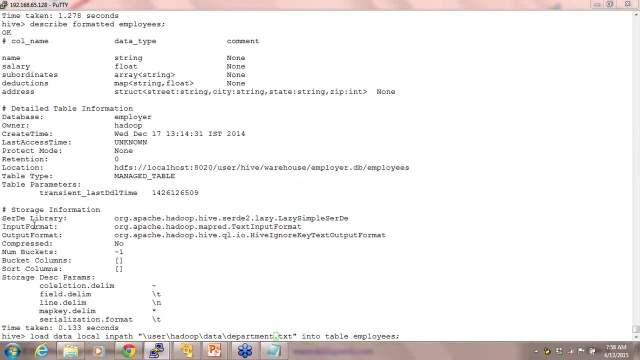 then you create an input format, okay, Sachin. So once you have seen your data, once you have designed what your input format will look like, you'll have to insert data which is of this input format. Now, when we go here- right, you see here, when I say select, describe format, it says: 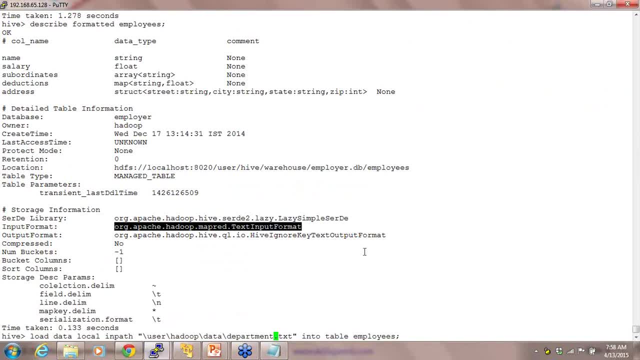 that the input format is a text input format. right, You define an input format first And then you start inserting into it. Now, how do you do that? You just look into the data first, you design an input format, and this all can be designed. 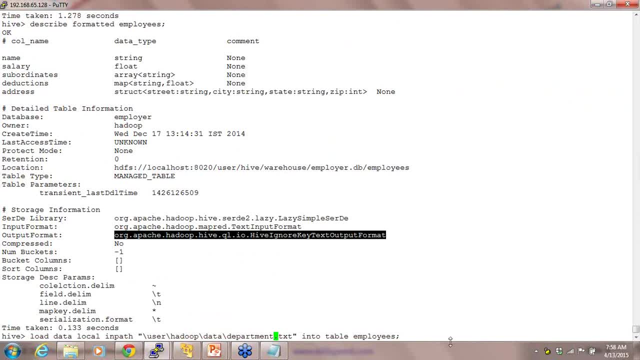 okay, This all can be customized. This all can be customized. Now, let me also take you through some more of this one. We are fast running out of time because I so this is what happens. okay, I just want to do now. if I say select, come start from employees. 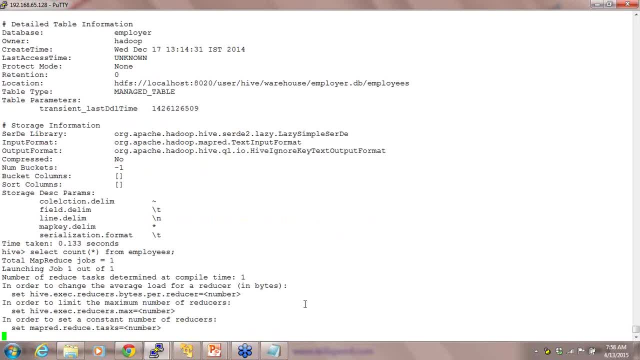 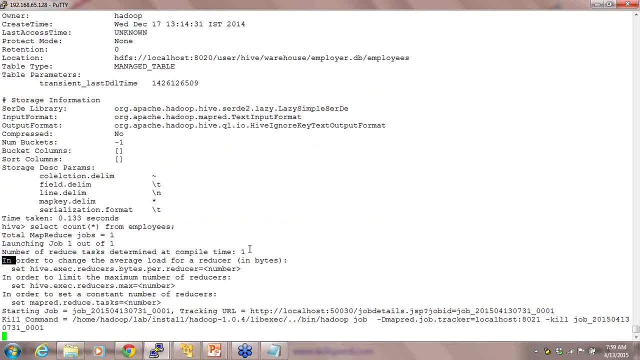 When I do that, what happens? Okay, You see this. It's launching map and reduce. So it so happens that in any databases it will go ahead, fetch the data directly from your table and do a count right Here. it's going through map and reduce. 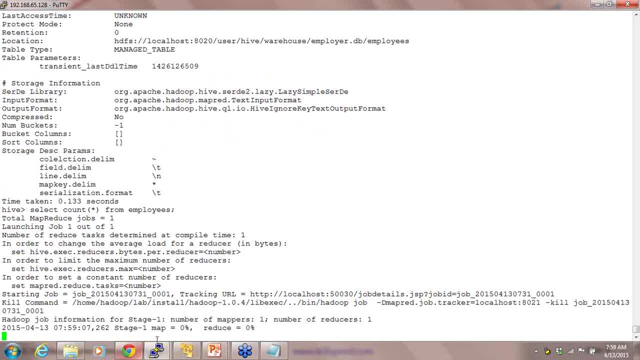 It says total map reduce job is one launching job, one out of one. It says map is zero, reduce is zero, so on and so forth. So it will continue until so. what it does is it will first take the file, split the. 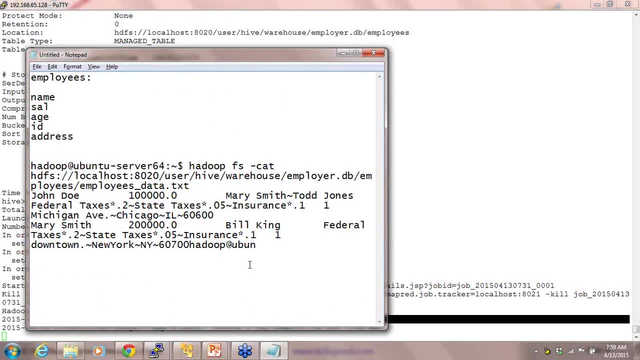 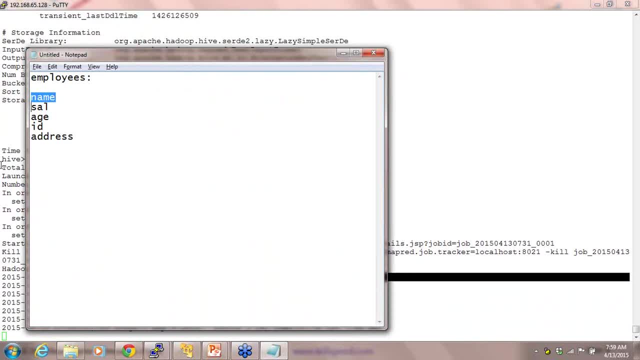 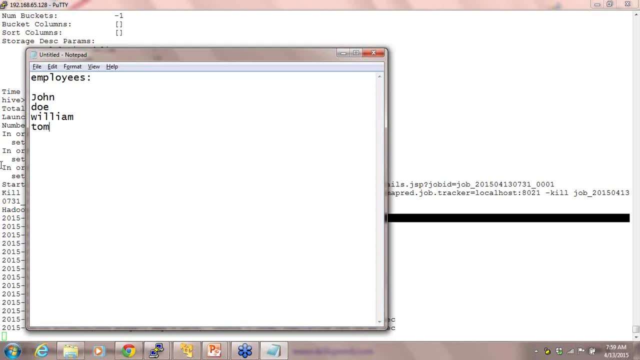 I have, let's say I have. let's say I have, let's say I want to count this. I have John Doe, William, okay, Tom, Let's say I want to count this. so what it does is it splits the data. 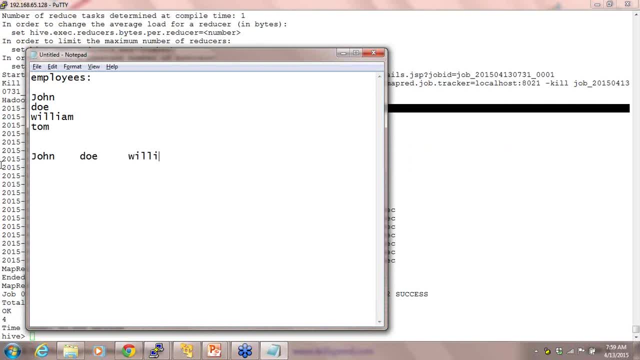 John into one system, Doe into one system, William into one system and Tom into one system. So eventually, from this system you'll get an output, something like this, saying that you know one, one, one, one, two, three. 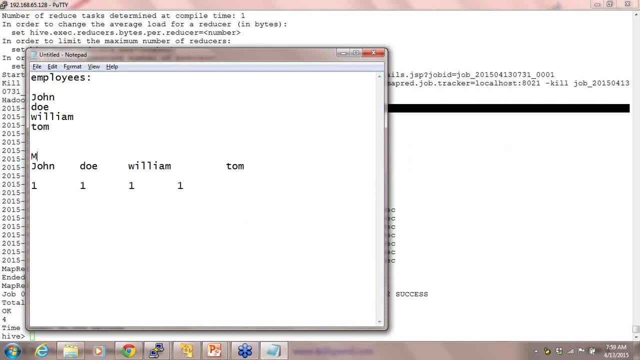 Okay, This happens in your mapper and this is what is happening in your reducer. It just takes this: 1 plus 1 plus 1 plus 1, and then you get 4 as an answer. So you see, here it got 4 as an answer. 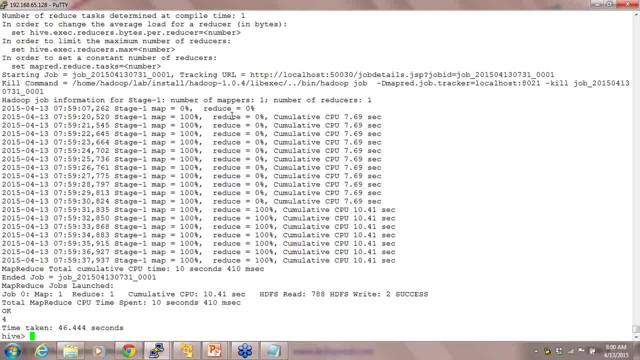 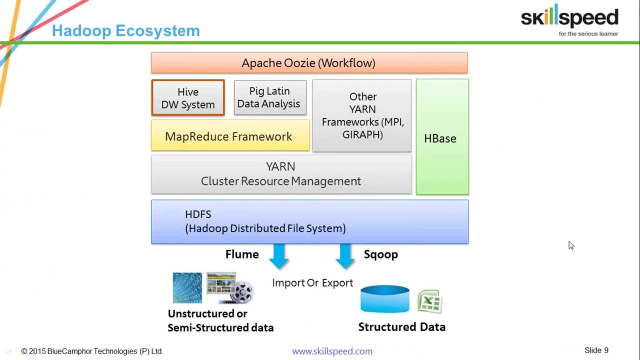 So map task is parallelizing the whole process, whereas your reduce task is aggregating the whole process. So, guys, I still see there are a lot of questions that you guys have which I might not be able to take it now, but be rest assured that we will have your questions answered via email. 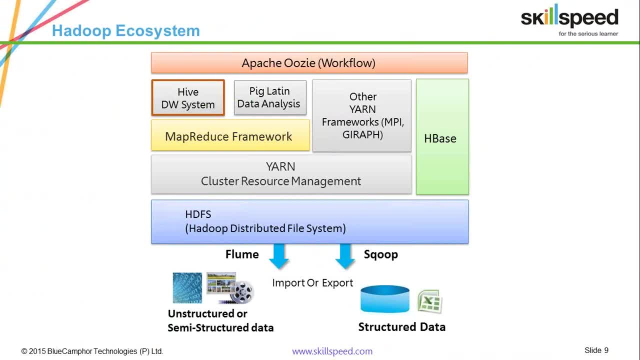 If you feel that that's an interesting question, or if that question is something which you will not be able to find an answer to, we'll certainly revert back to you. So this is Hadoop ecosystem. guys, We have Hive, We have Pig. 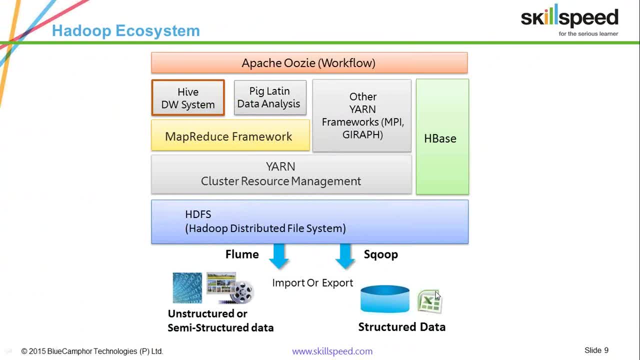 We are only talking about Hive. We have also discussed a little bit of HDFS To pull data from the Hadoop ecosystem. we have Hive, we have Pig. We are only talking about Hive. We have also discussed a little bit of HDFS. 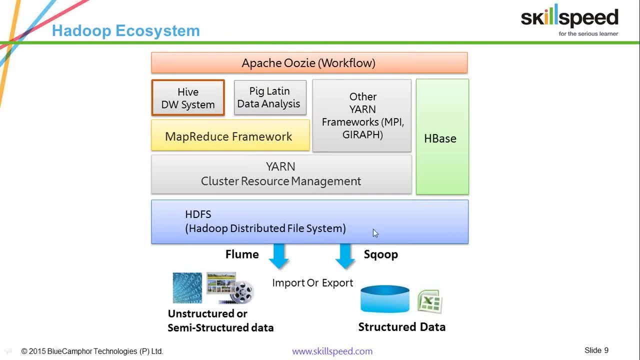 To pull data from the Hadoop ecosystem. we have Hive. We are only talking about Hive. We are only talking about Hive. We are only talking about Hive. To pull data from structured databases, we would need scoop. and to pull data from some. 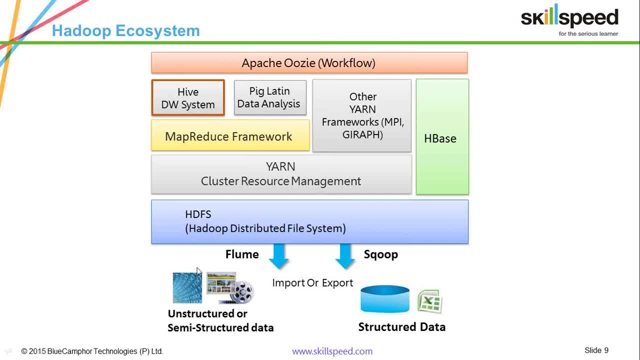 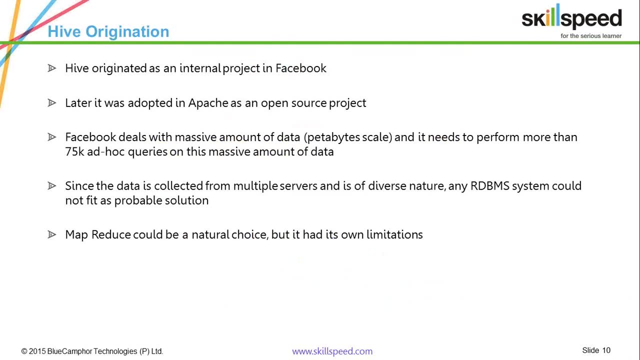 of you who have already asked me this question regarding how do I pull data from Twitter, etcetera that we use Hive Again, Hive originations. this are stories that will be shared with you. You can read about this as well. You can read about this. 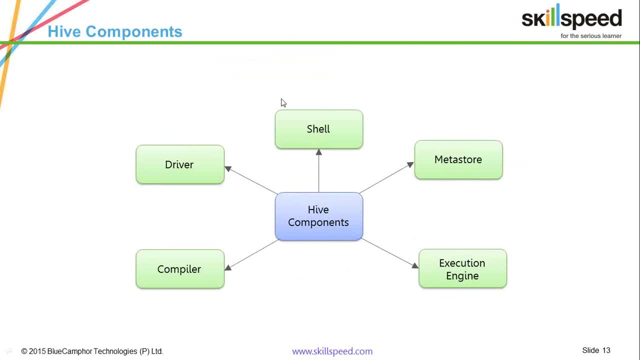 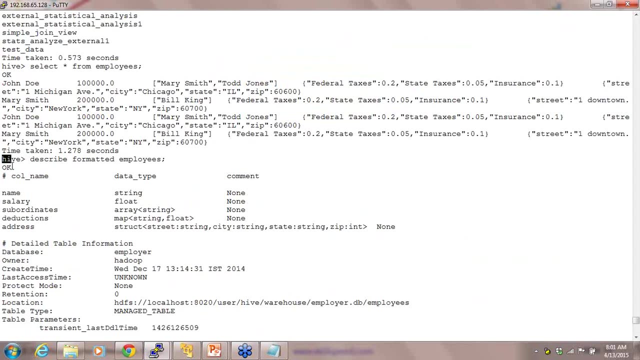 You can also access Hive using your Hive cell. These are Hive components. You have a Metastore. When I say describe, format it. it gave me all this information. This information I can store it in MySQL, only the metadata part of it. 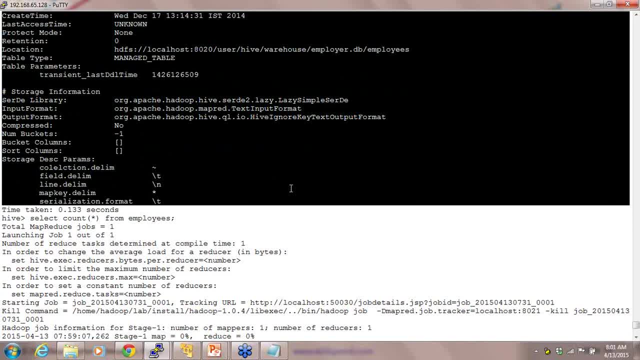 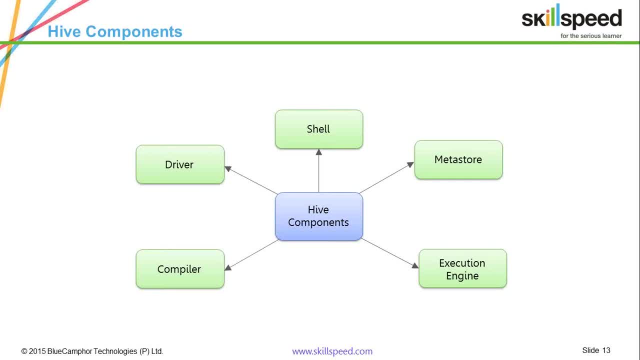 If you did not know what metadata is, it's the data which describes the data. right Data of a data is metadata, So I can store my metadata by default. the database is Derby and you can also configure it to store it in MySQL SQL Server, your database, your Oracle DB2, et cetera. 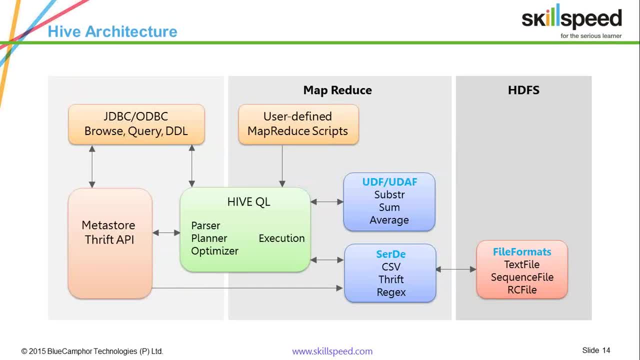 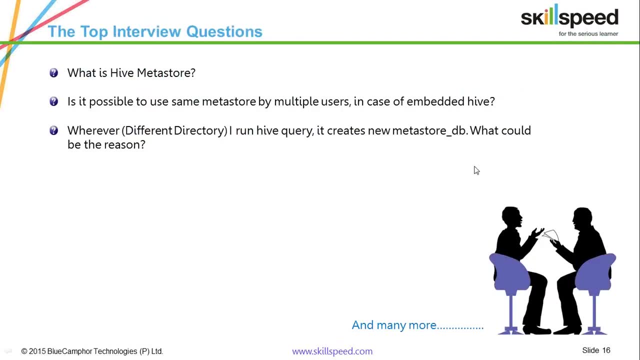 So this is architecture, not going into very details of it. This is top five, top couple of interview questions. what is Hive Metastore? it is possible to use same Metastore by multiple users in case of embedded Hive. So simple questions, right. 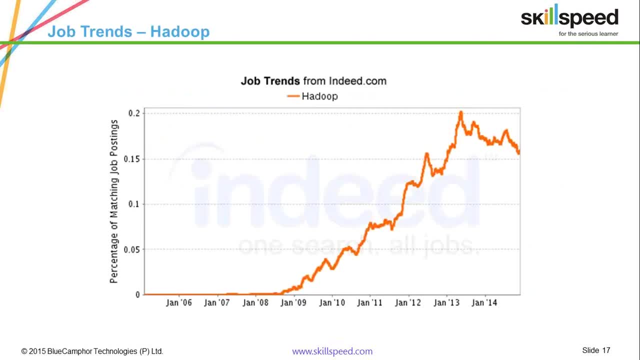 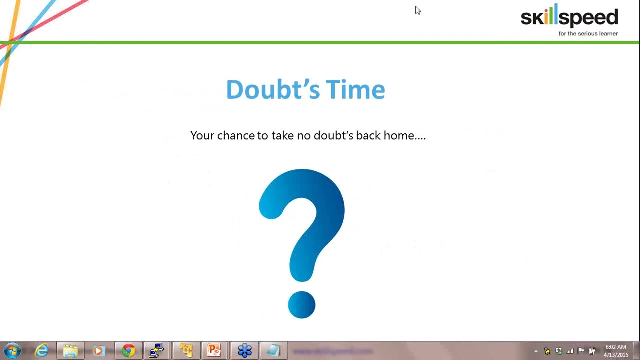 And last but not the least, the job trends. it's just here to stay. it's just growing from 2006 to 2014,. it's on the upward swing right now. So that's some more doubts. I'll take some more of your questions. 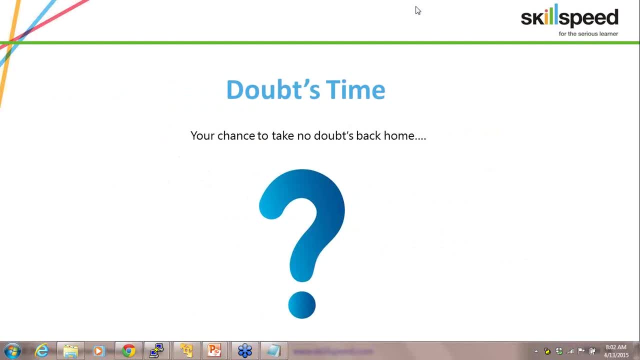 So will the class be about how to insert data or the query language? that Hive is our step to clean the data. So, Niharika, the class would be about everything, starting from how to set up the system to how would you slice and dice the data. how would you pull the data to, how would you? 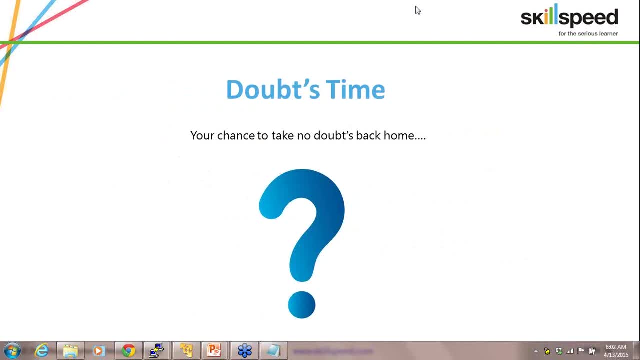 process the data to, how would you process using PIG, how would you process using Hive right And how would you process using writing your Python code? Sorry guys, some of you asked me to show How do I integrate Python and Hive. 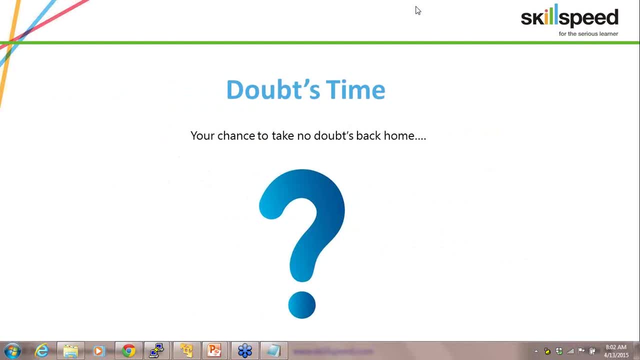 I did not have time so I could not do that. Okay, Sudip is saying: this was amazing Yogendra. No problem, Sudip, It's all my pleasure, It's my first time here. says Vivekananda. is there a way I can access the previous recordings? 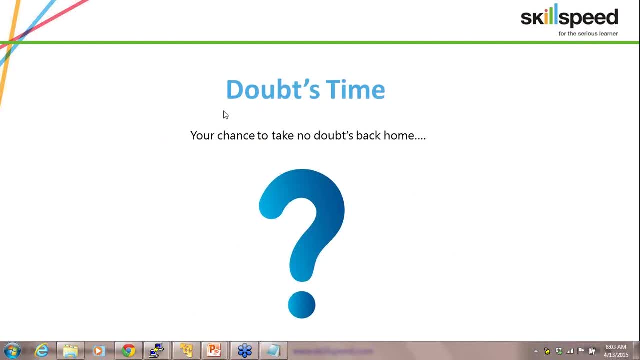 Okay, now, let me. now I will take in your questions a little bit later. but hey, Mohit, are you there? I would want you know, Mohit, to take in all of your questions on the courses, et cetera.